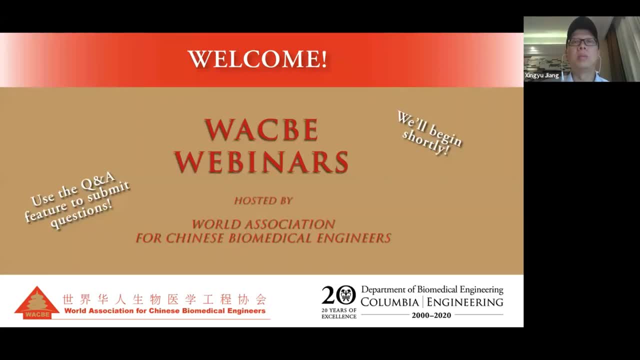 Okay, we'll get started. Welcome everyone to WACB webinars, our Distinguished Biomedical Engineering Webinar Series hosted by the World Association for Chinese Biomedical Engineers, or WACB. My name is Xinyu Zhang, or Zhang Xinyu in Chinese. I am from the Department of Biomedical 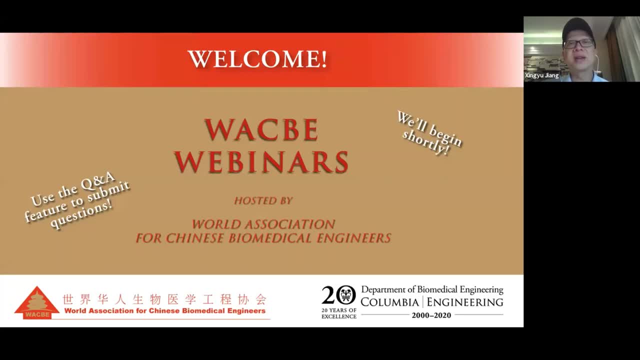 Engineering at the Southern University of Science and Technology in Shenzhen, China. The format of our webinar is the following: Our speaker will present for approximately 40 minutes and will leave 15 to 20 minutes at the end for Q&A Throughout the presentation, please feel. 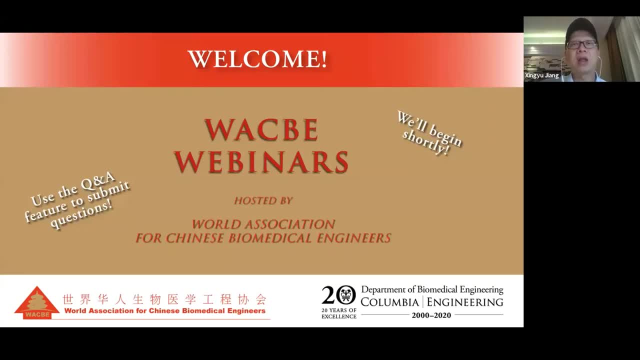 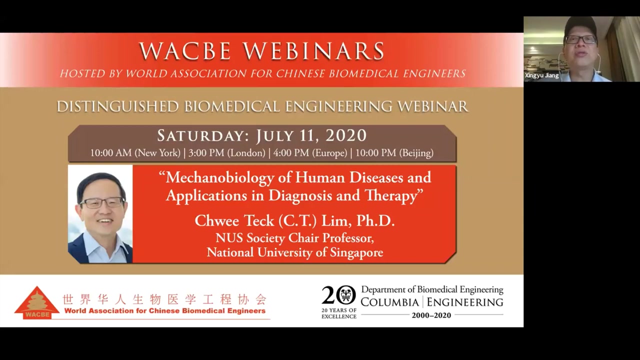 free to use the Q&A feature at the bottom of your screen to submit your questions. We will try to answer as many as possible. If you have any questions, please feel free to ask them in the Q&A session. Today we are excited to welcome Professor CT Lin from the National University. 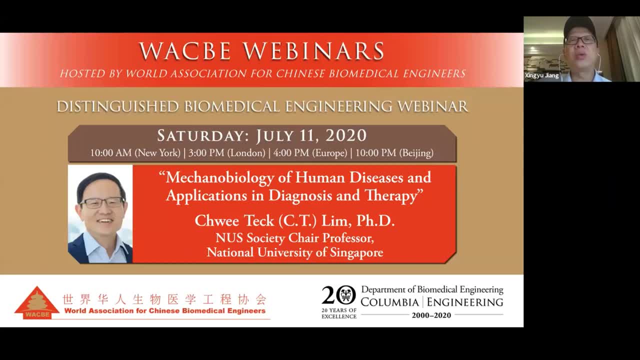 of Singapore. Professor Lin is the NUS Society Professor and Director of the Institute for Health, Innovation and Technology at the National University of Singapore. His research is in mechanical biology and microfluidics. He has co-authored over 400 peer-reviewed journal papers and given over 390 invited talks. He is an elected fellow of the AIMBE IAMBE Academy. 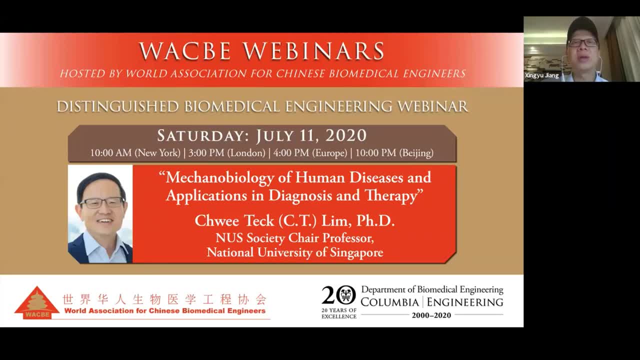 of Engineering Singapore and the Singapore National Academy of Science. He has co-founded six spin-off companies. He and his team have garnered over 100 research awards and are receiving honors including Highly Cited Researcher 2019, Asian Scientist 100 2016,. Wall Street. 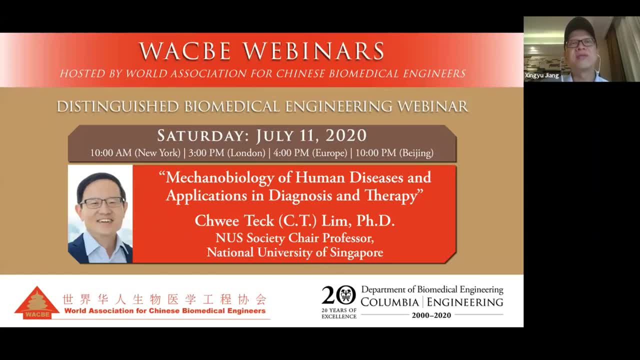 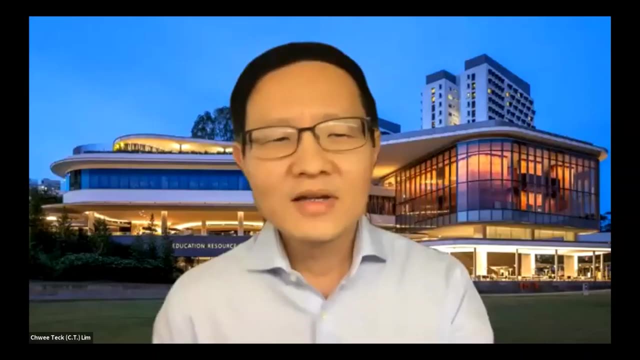 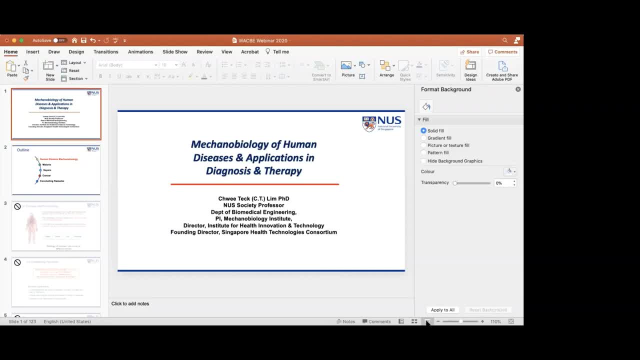 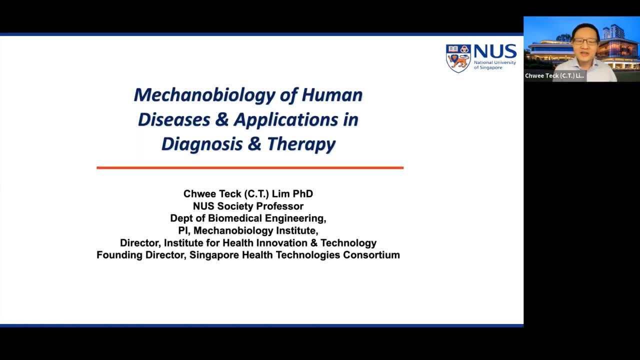 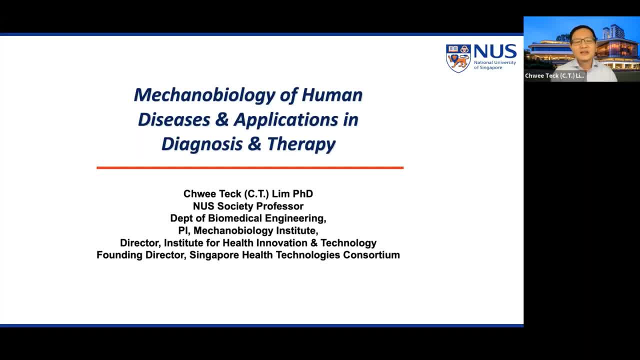 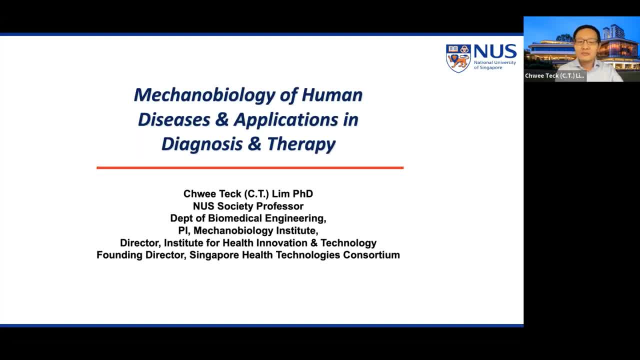 Ed Guo and also Amy, for organizing this whole series of webinar, and I thought it's a very important initiative because this is an opportunity for us to see how we can disseminate some of our research findings through such a very useful platform. For this talk, I'm going to focus on some of our work on mechanical biology of human diseases. 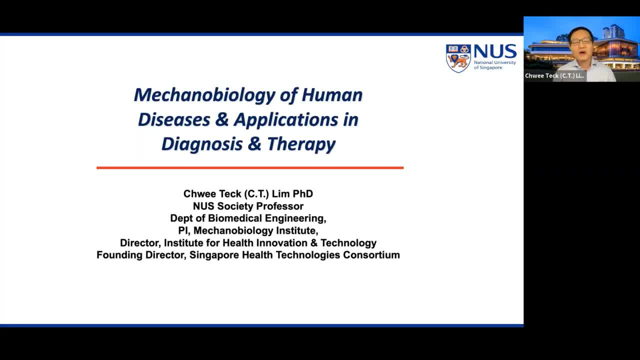 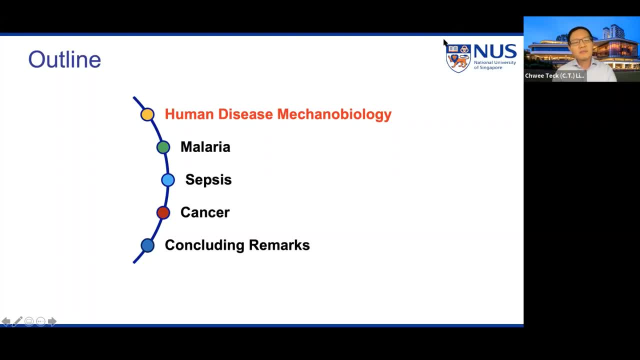 and also to share with you how we actually use some of the findings for application, diagnosis and also therapy. So this is the outline of my talk. I'll first talk about what is human disease- mechanical biology- and I will actually cover three diseases. the first is on malaria, second on sepsis. 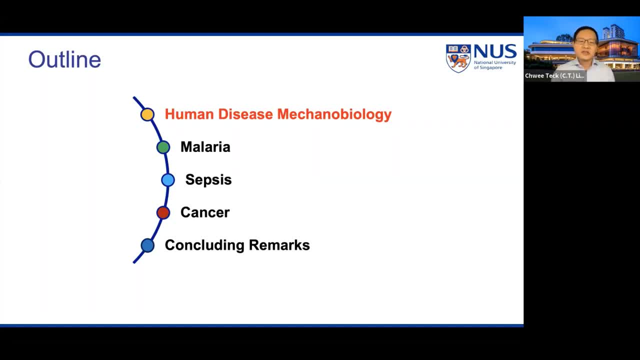 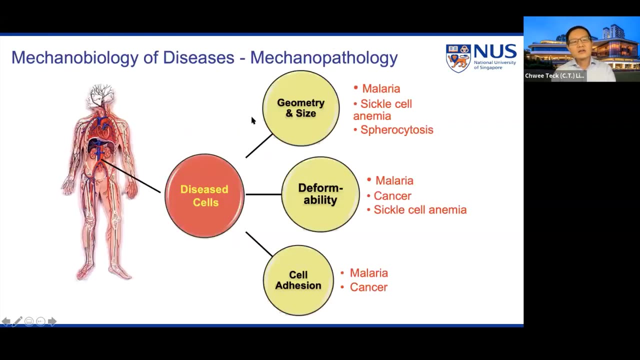 and then I'll end with cancer, and these are three diseases that we have been working very much in our lab and I will show you how we go about. So when we talk about diseases, from some of our studies on certain diseases we found that they do actually change in terms of biomechanical properties, and this can include geometry and 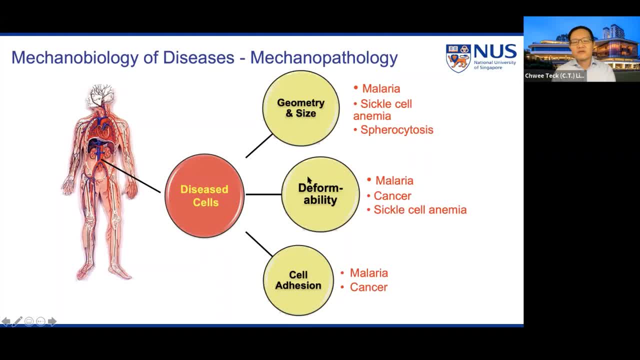 structure and size, as well as deformability and cell adhesion. Other associated diseases are, such as malaria, sickle cell anemia, spherocytosis and also cancer, and in fact, some of the changes in these biomechanical properties can give rise. 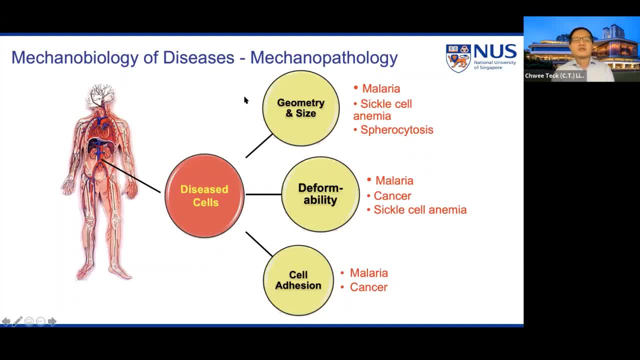 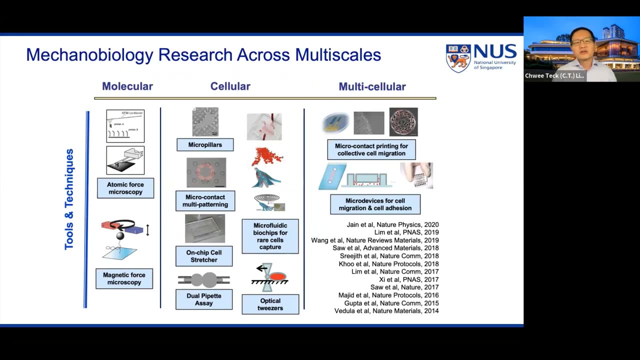 to or rise on diseases and we use the term mechanopathology to describe how changes in such mechanical properties can lead to pathological outcomes. So in my lab we have been: We focus very much on the cellular level. Actually, we do also engage in quite a bit of the molecular and multicellular studies. 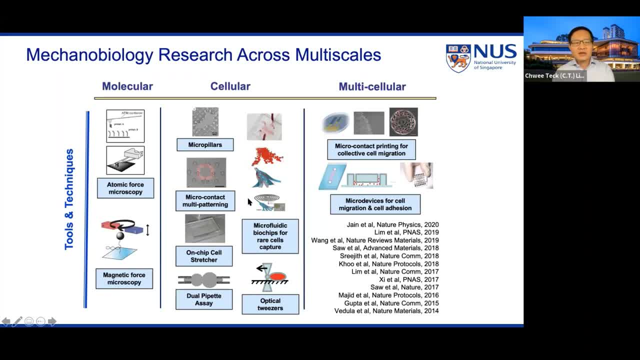 as well, and this diagram here shows some of the techniques we have been using to conduct some of these studies. For example, the molecular level: we do use a lot of the AFM and magnetic force microscopy. and at the cellular level actually we do a lot of, for example, micro pillars, where we 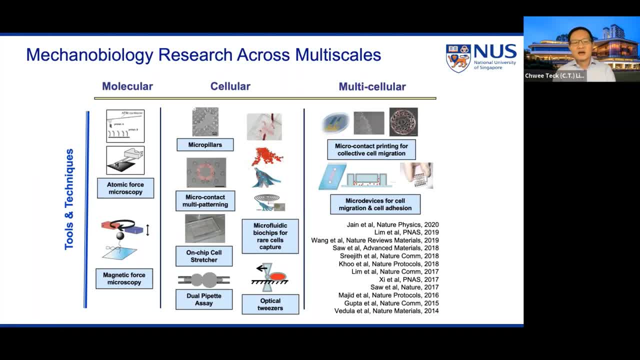 put cells in the pillars To measure contractile forces, as well as micro contact multi-patterning to see how cells would respond to the surface that the cell adhere to, as well as developing other techniques like dual pipette assays and optical tweezers to measure cell adhesion and microfluidics. 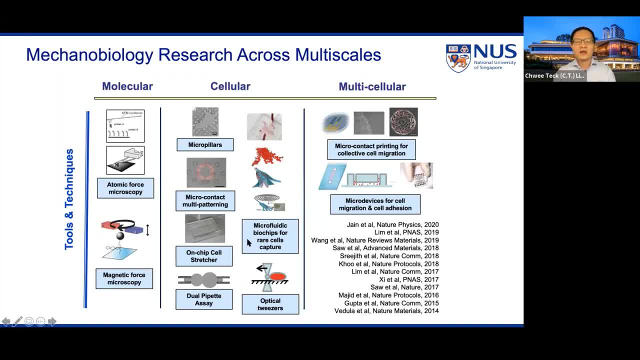 to be able to capture some of these disease cells from a large population or other cell types. So, at multicellular level, actually, we have been also doing a lot of collective cell migration work in relation to, for example, wind healing and a lot of some of the techniques we use. 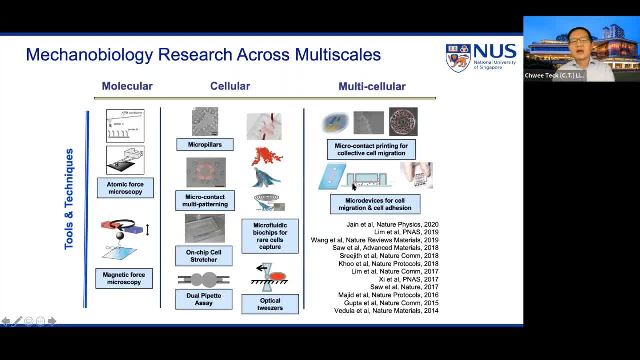 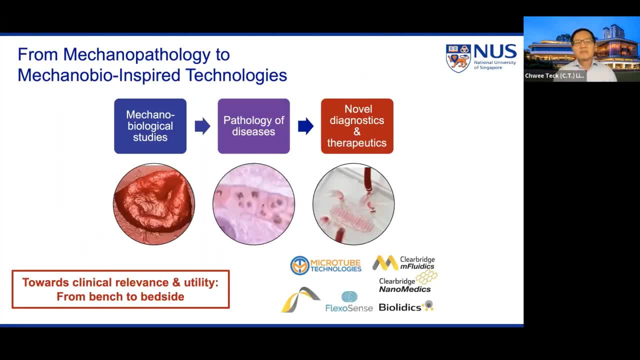 also not only including micro contact printing but also microfluidics where we can flow cells, look at how cells will adhere to surfaces. So in our lab, basically, we conduct a lot of basic research for start to understand the mechanical biology of human diseases And the approach is somewhat, actually quite, of interest to our clinicians, because when 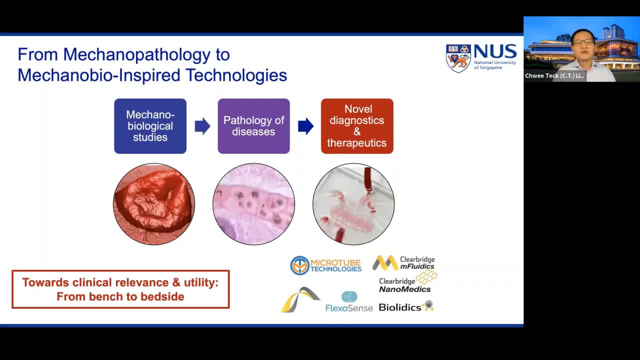 we first started this research the clinicians didn't quite understand what we are coming from, but after working in the last 10-15 years I think they do appreciate us coming from the mechanical biological perspective and this is a kind of a different approach in looking at diseases and how changes in mechanical biological properties can lead to the pathology. 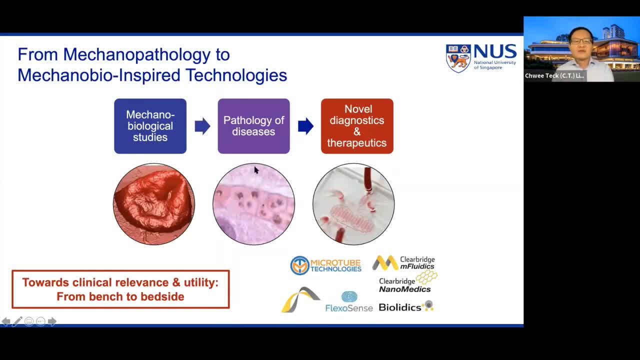 of diseases And as an end-to-end discussion, I would just like to say thank you so much for your time. Thank you, I myself am also very interested to see how this accumulated knowledge can be applied to develop very novel diagnostics and therapeutics. 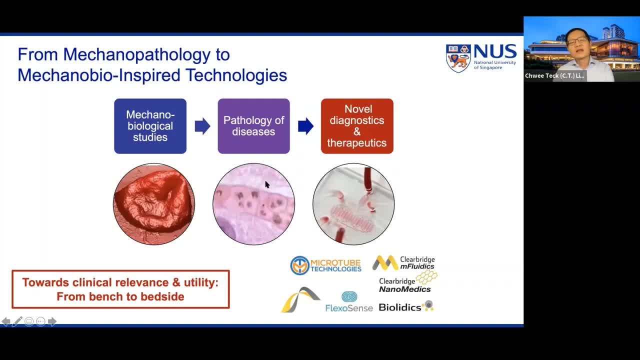 In fact, the first half is basic research but the second half is a lot of translational work. So half of my group actually works a lot of basic research and the other half of translational work, And actually this led to a number of spin-off companies as well. so we are very keen to 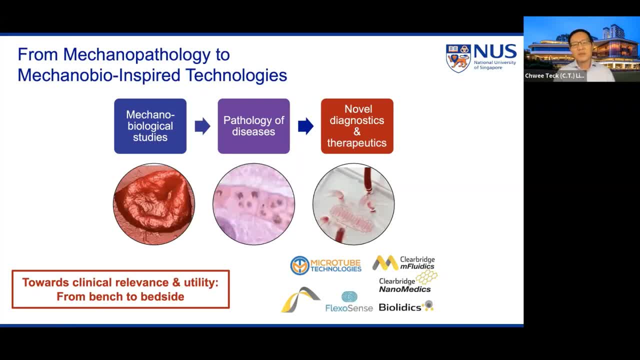 see how this, how we can bring some of this from the beginning and to the end of the quest. Thank you. we research from the bench to the bedside, So now that we really try to aim towards clinical relevance and also utility. So let me first go to the first disease, malaria. 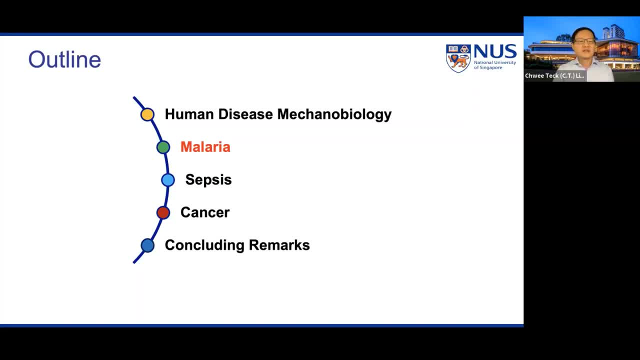 So this actually is the disease that I first work on when I first started my lab, And it arises actually from a coffee break that I had with a colleague of mine from the microbiology department, So he was telling me that he's working on malaria. 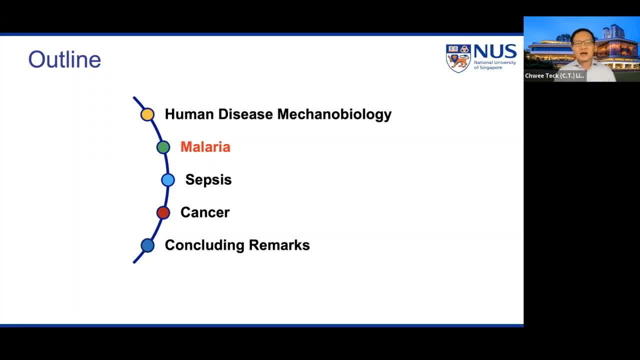 and he says that the cell, when a red blood cell gets infected, it becomes stiff and sticky or the cell adhesion actually increases. And so when he told me of this problem, I realized that actually it relates to mechanics and we have some equipment that we can help them. 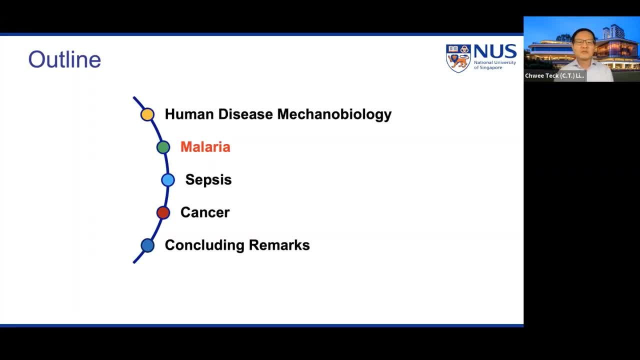 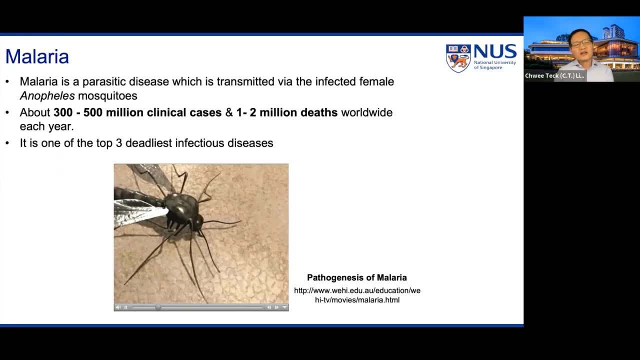 to study that, because when he was looking at this problem they weren't able to quantitatively measure the stiffening of the cell or the increase in cell adhesion. But before I go into the some of the findings, let me just introduce what is malaria? 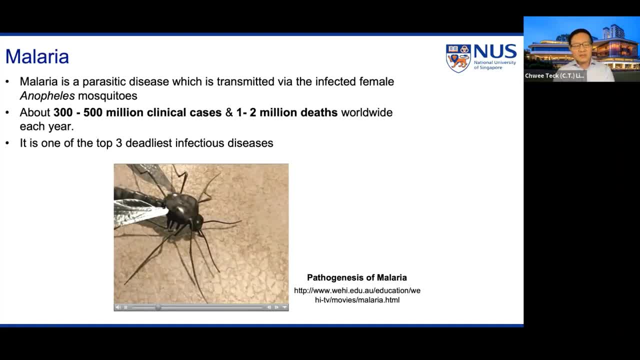 So malaria is actually one of the three most, one of the three deadliest infectious diseases. So it's a parasitic disease which is transmitted through a female anopheles mosquito. So every year there are about 300 to 500 million clinical cases and one to 2 million deaths each year. 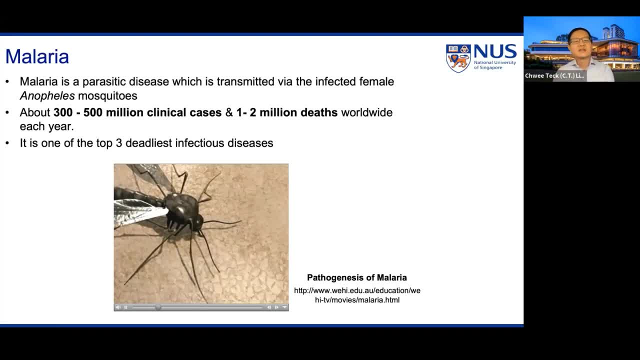 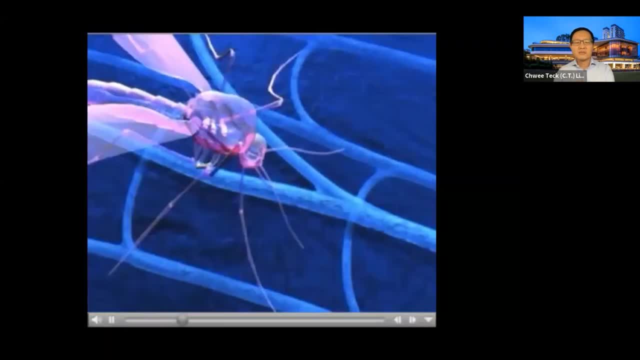 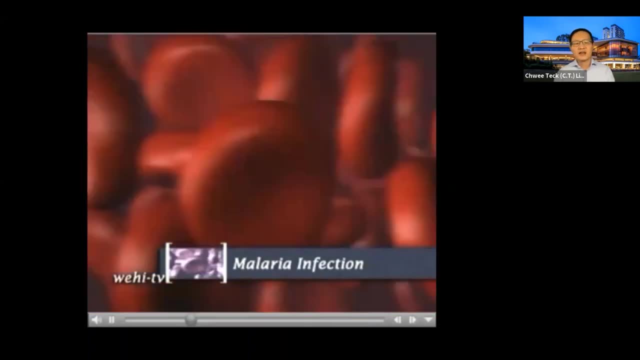 So you can see that how serious this disease is and how it works. is this So: when an anopheles mosquito take a blood meal from a person, it will inject parasites into the bloodstream, where the parasites would then go into the liver cells and from liver cells. 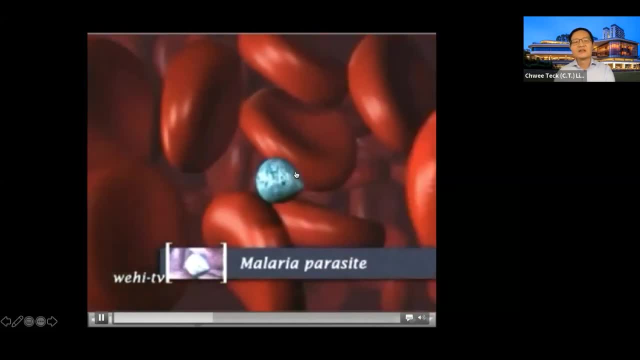 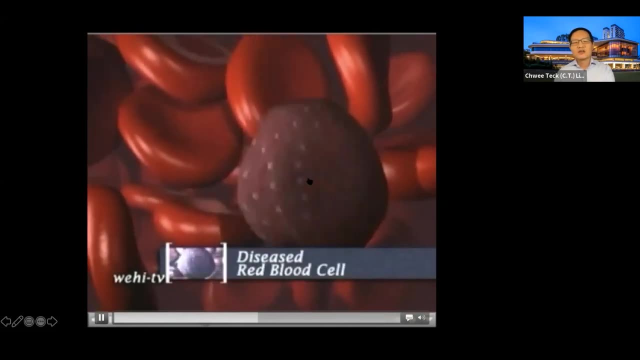 it will develop into this myrizoid, as you can see here. So once the myrizoid goes in the bloodstream, it can actually attach to a blood cell, squeeze its way into the blood cell, causing massive changes to a blood cell. The blood cell becomes stiff and sticky. 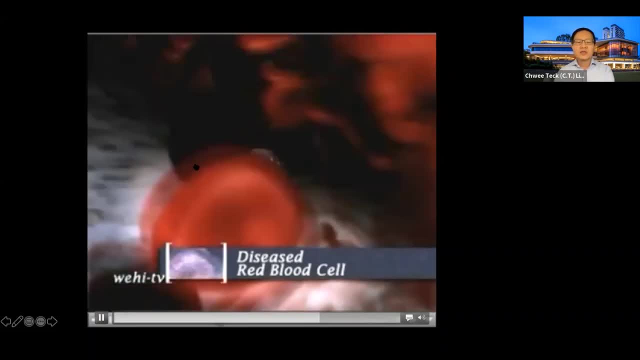 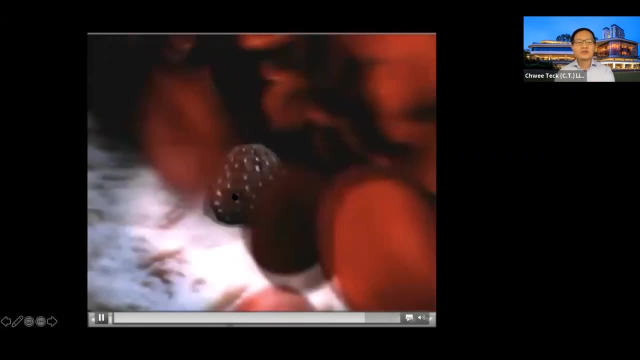 So it becomes sticky, it can actually adhere to the, to the surface of the blood vessel, And within two days it will actually multiply from one to about 10 to 20.. And then, after you break out the infected cell and start to infect other red blood cells, 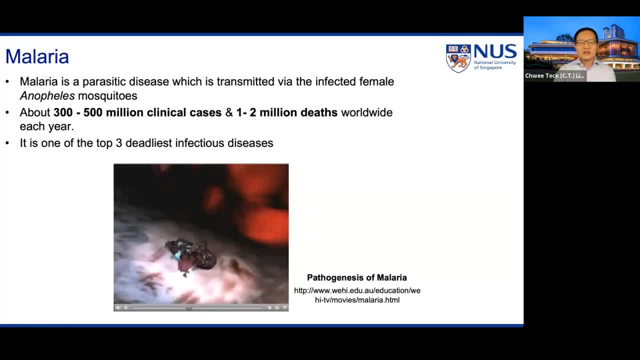 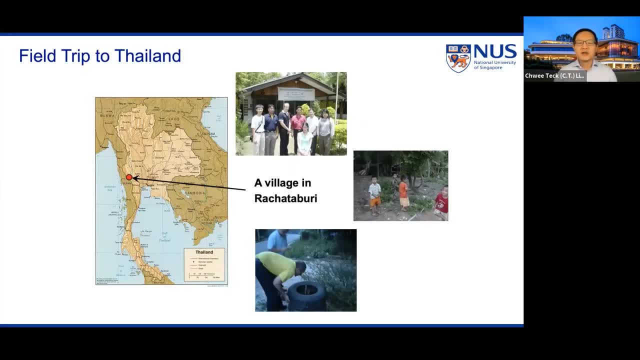 And so this is the life cycle of the pathogenesis of the malaria, And so when we started this research, we also collaborated with a group, Professor Wu Sa- actually from the Mahidol University in Thailand, So we made a field trip to this place. 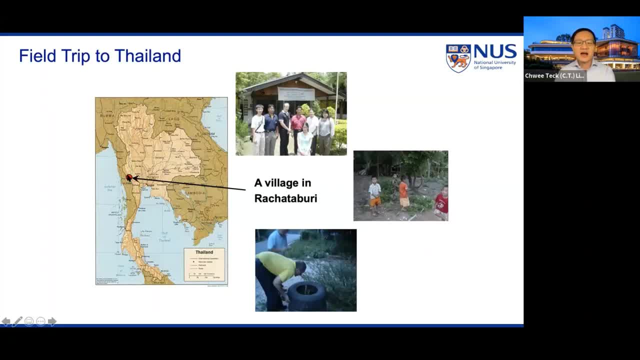 called Ratchathaburi, which is at the border between Myanmar and Thailand. So in there over there, there's a village which house about 500 villages, and they're actually refugees from Myanmar. So when we were walking around the place, 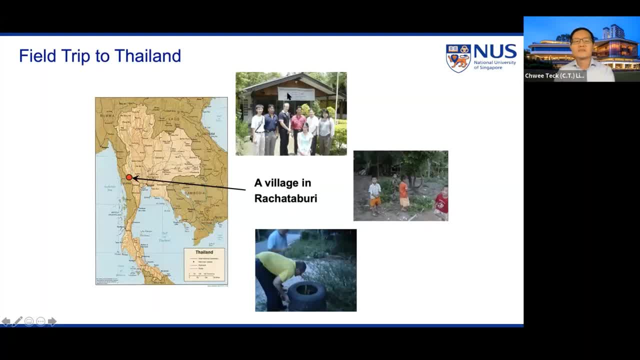 so this is the clinic where the villagers will come to seek help if they fall sick, And so when we walk around, there are a lot of adorable kids there, And when we look at, for example, rubbish like, for example, a discarded wheel like this: 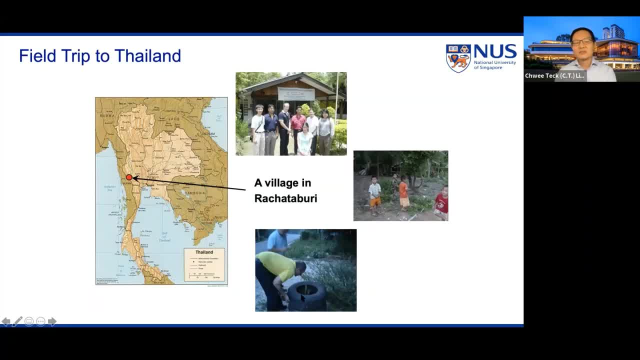 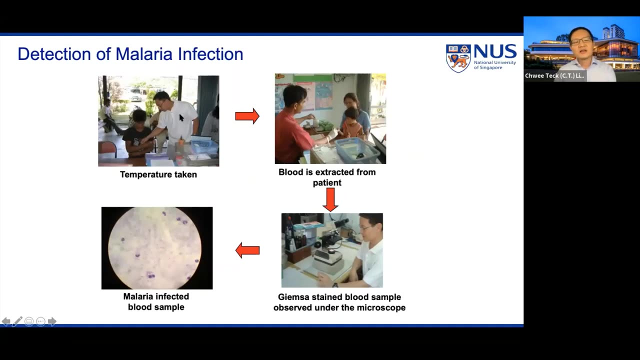 a tire, a wheel tire like this, and it's the perfect receptacle for collecting water And we look into it. actually it's a breeding ground for mosquitoes, So the infection is really quite serious over there. So what happens is if a villager is sick, 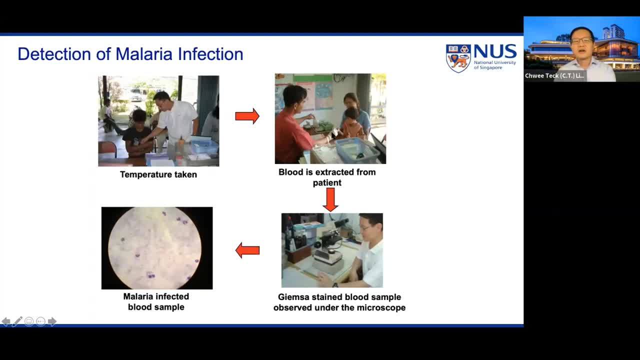 the villager will come to take a blood test. So the medical officer will do a finger prick to drop a few bloods onto a glass slide And then after that we'll do a ginseng stain and within half an hour 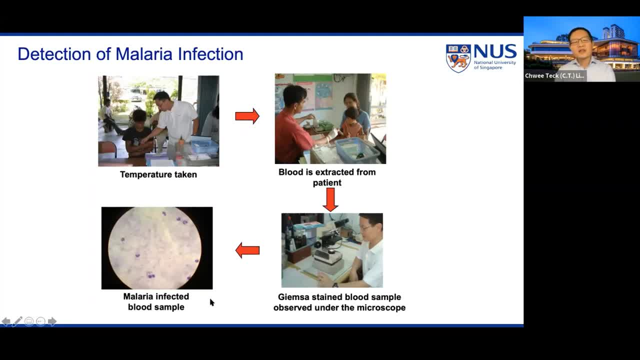 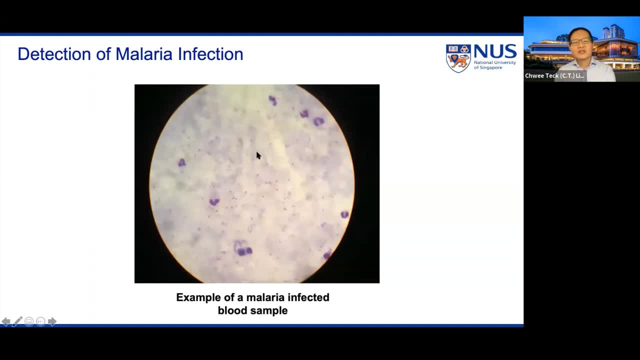 we'll look underneath a microscope, as shown here. So under the microscope, this is how it looks like. Let me show you a large figure. So over here you can see that these are actually in the background are actually red blood cells. 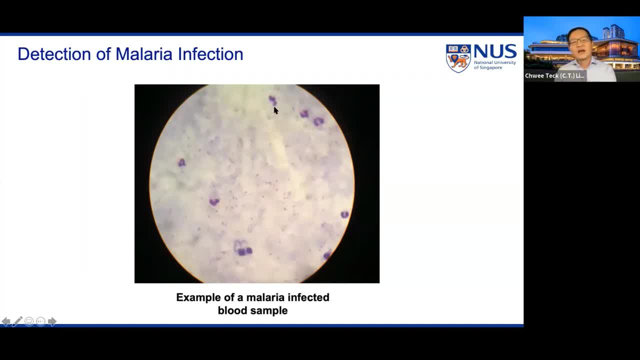 They appear published in color is because the ginseng stain And this larger patches of published color features are actually white blood cells. But if you look very closely there are these tiny little specks inside the cell. These are actually malaria parasites. 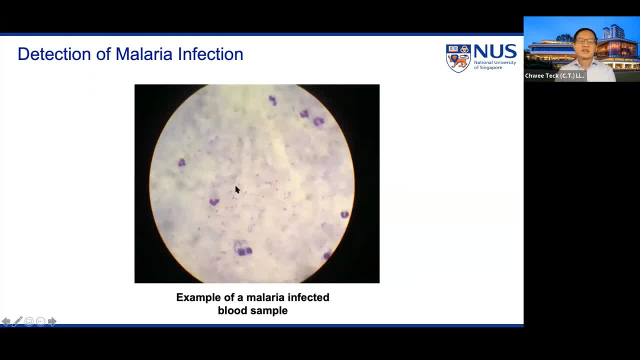 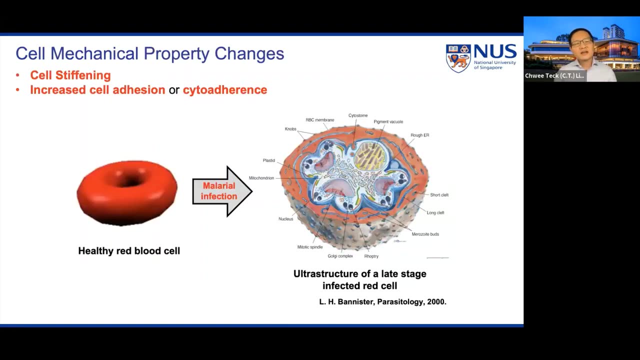 So from this picture itself, or the image itself, you can tell that the person has been infected with malaria. So once we found that it's positive, the doctor or the medical officer will then administer anti-malaria drugs to the patients. So when we look at what happens to a red blood cell, 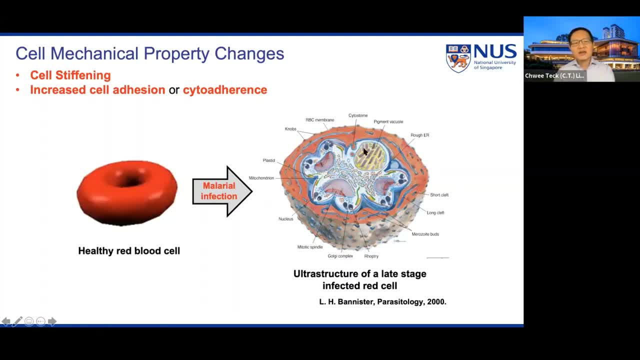 when it's infected with the parasite, it actually not only becomes stiffer, but also there's an increase in cell ignition and there's an increase in parasite adherence. So this is what happens inside the red blood cell. So you can imagine from a red blood cell. 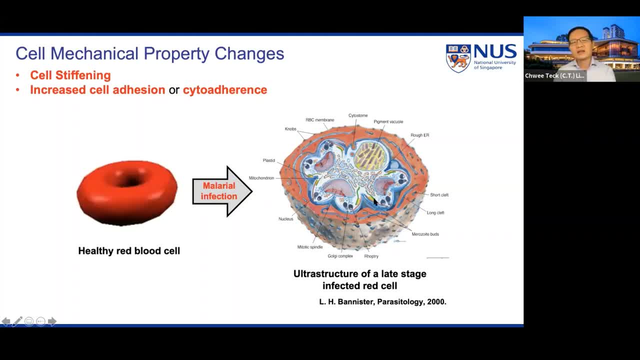 which just contains hemoglobin, to one that contains many other organelles and so on. inside the cell, apart from the parasite itself, And also on the surface of the infected red blood cell, you can see these tiny little knobs. These are actually proteins that gets embedded. 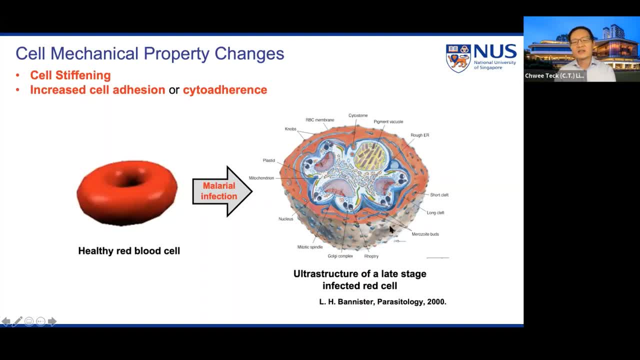 in the membrane of the red blood cell, And these are the knobs that cause the cell to be burned. So the red blood cell can be very sticky or very adhesive to the endothelium, And this is what causes this whole red blood cell to be both very stiff and very sticky. 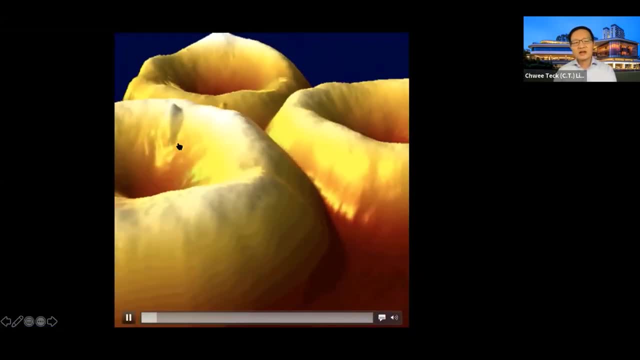 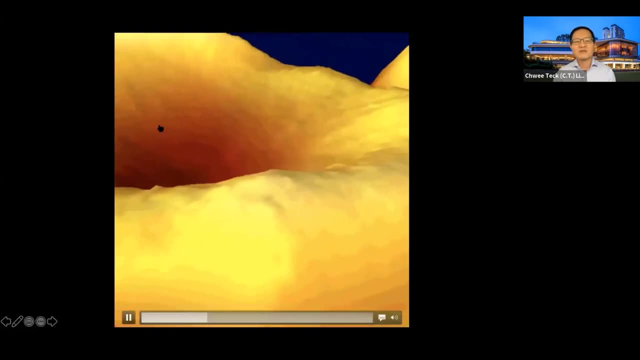 So if you look at the red blood cell- healthy red blood cell- this is how it looks like. So using AFM, we were able to image the red blood cell. You can look at the red blood cell itself. it's biconcave in shape and the surface is relatively smooth. 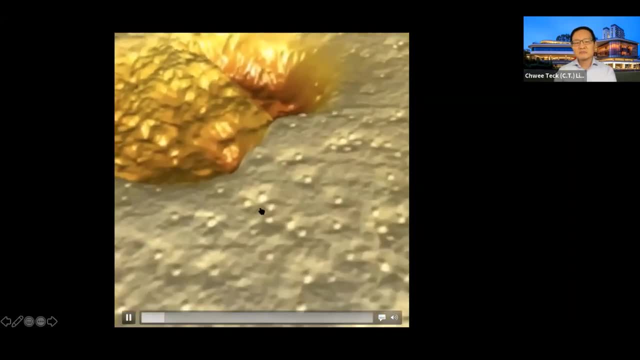 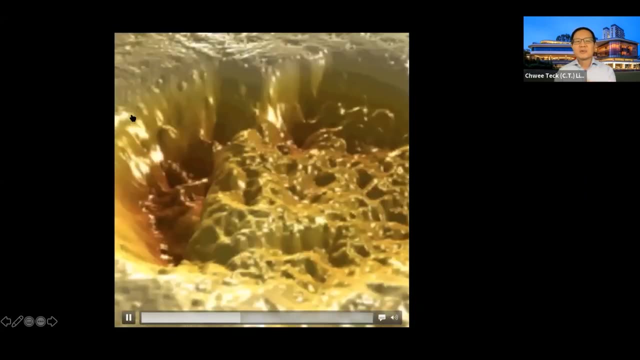 If you were to look at an infected red blood cell, this is how it looks like You can look at the surface. there are all these little knobs. These are the cut protein that is secreted by the parasite that gets embedded in the membrane. 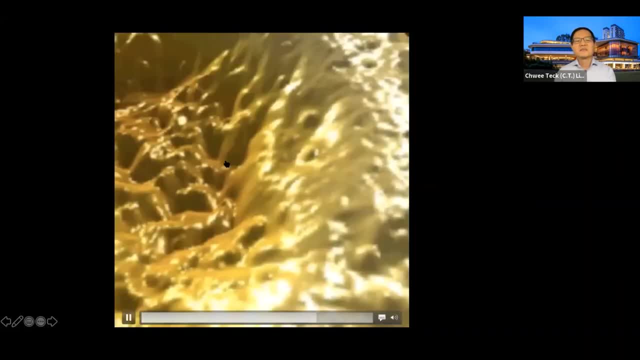 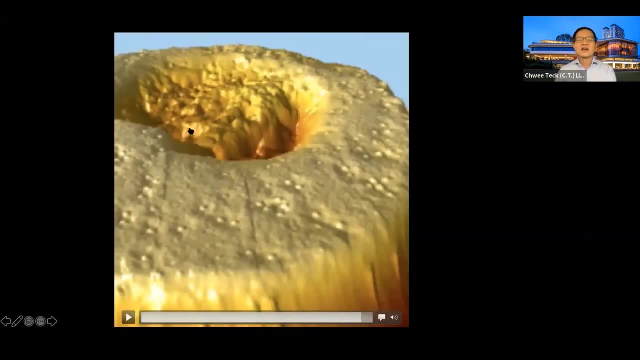 And this is what causes the cell to be very sticky. And also, if you look at this red blood cell right in the middle is actually where the parasite is. So it looks like a crater because when we smear the infected cell on the glass slide. 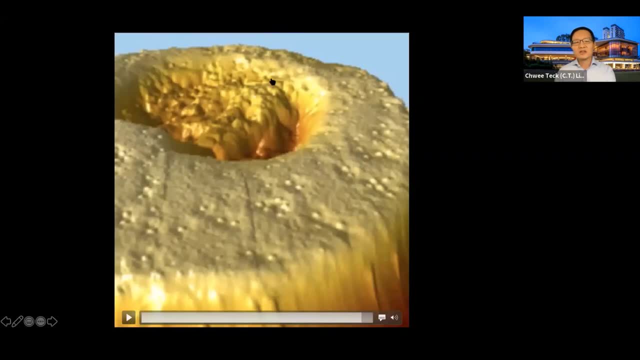 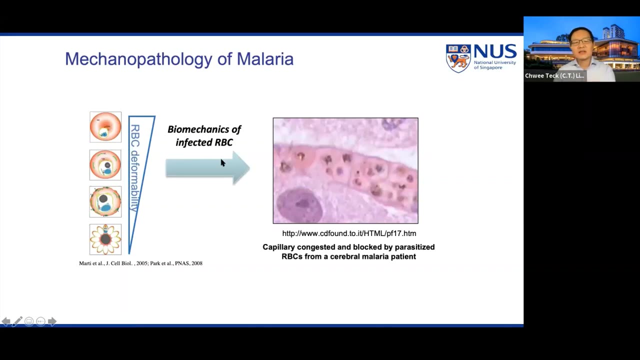 the membrane actually sticks to the parasite. So over here you can tell where the parasite is. So over here you can tell where the parasite is. So the mechanopathology of the malaria is such that when the cell becomes stiff and sticky, 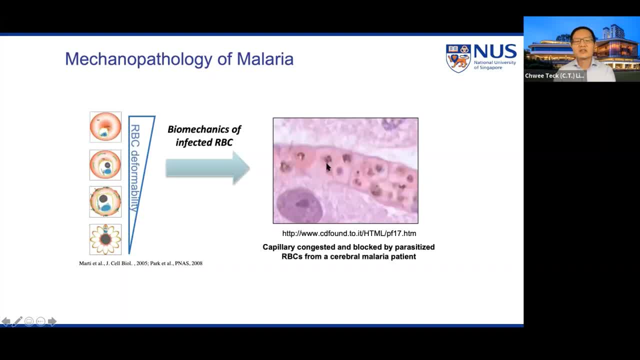 it will actually be able to clog the capillaries, And so this is bad news for our body, because our red blood cell has to be very deformable and non-accessible in order to flow through the circulatory system, But when he becomes stiff and sticky, 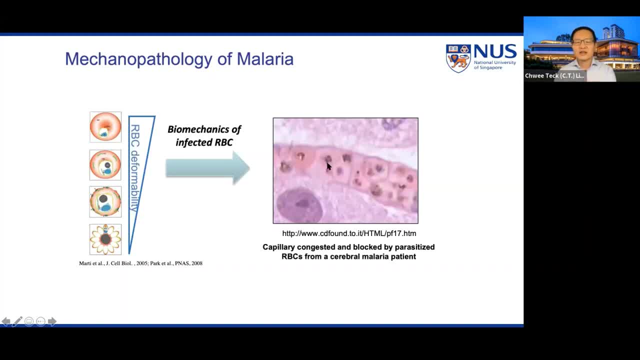 this is what is going to happen. The capillary can get congested, And so this is a picture of a capillary that's blocked by the infected red blood cell from a cerebral malaria patient. So in our lab we have actually been doing quite a number. 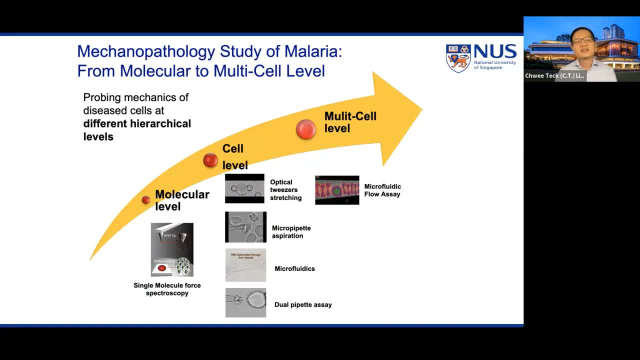 of different studies: mechanobiological studies, not only probing the adhesion and the molecule level, but also performing a cell mechanic study at the cell level and thereafter multi-cell level, just to mimic what happens if a group of infected cell flows through the narrow capillaries. 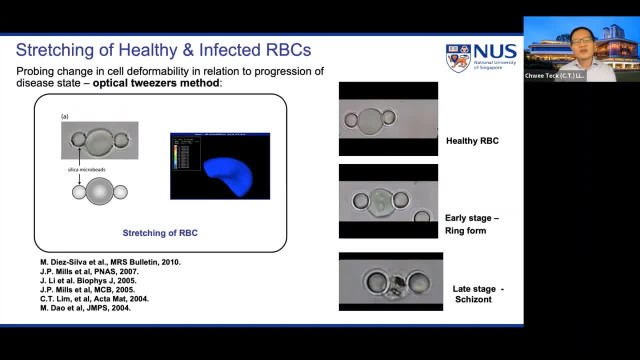 And straight in time. we'll just talk about the cell mechanics work. So one of the first experiment we did was use optical tweezers to stretch malaria-infected cells. So how the experiment works is this: we attach two beads to the side of the red blood cell. 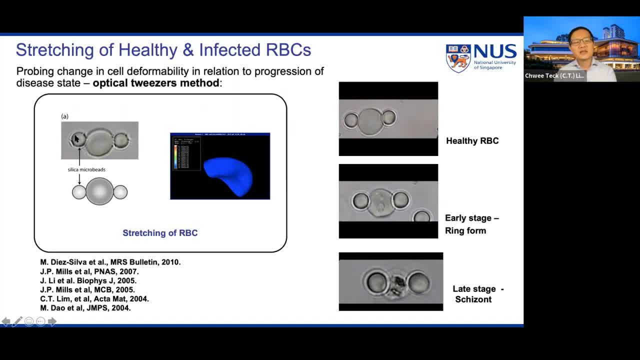 So for our case we are using a single laser. So one bead is attached to the surface of the glass slide, The other bead is trapped using a laser. So when we move the laser or if you move the glass slide, we can actually spread the laser. 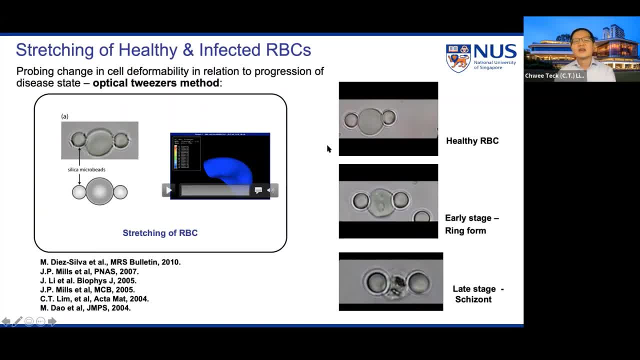 So when we move the laser, or if you move the glass slide, we can actually spread the laser to be able to stretch the red blood cell. So let's look at the stretching of a healthy red blood cell. So this is what happens when we use the laser. 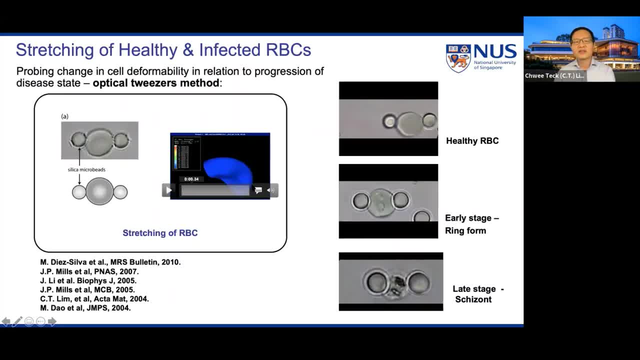 to track one bead and move the laser, we can actually stretch the red blood cell. So over here. if you look at the experiment itself, the amount of force we apply is actually very small. It's about between zero to about 170 to 180 piconewtons. 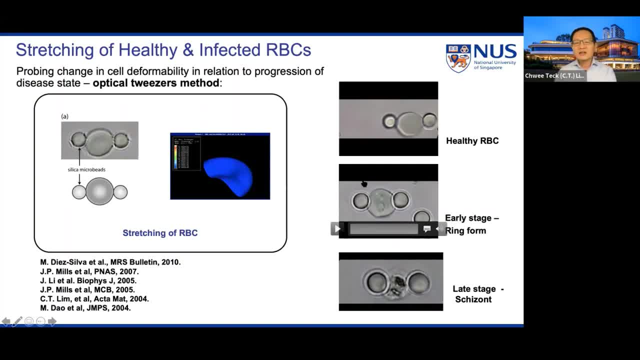 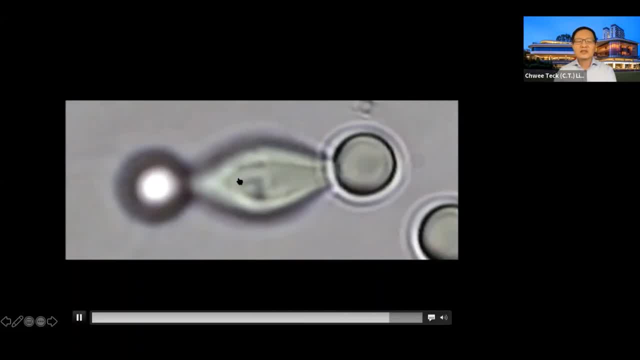 but that's large enough to stretch the red blood cell At the early stage of infection and you can see there's a parasite inside the red blood cell. the cell is still somewhat deformable, So this is about between zero to 16 hours of infection. 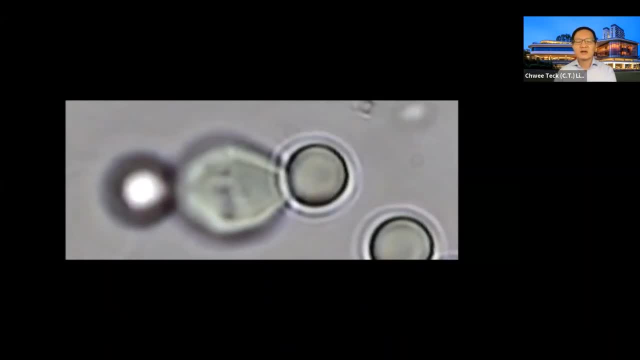 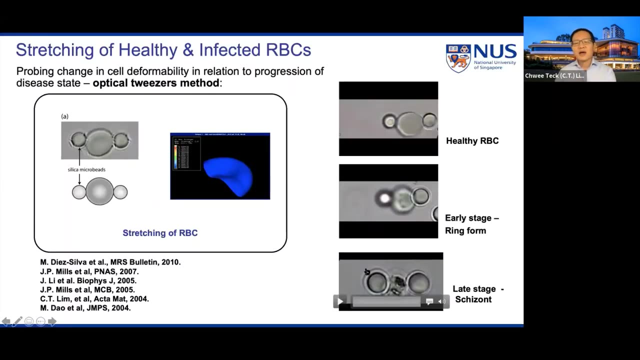 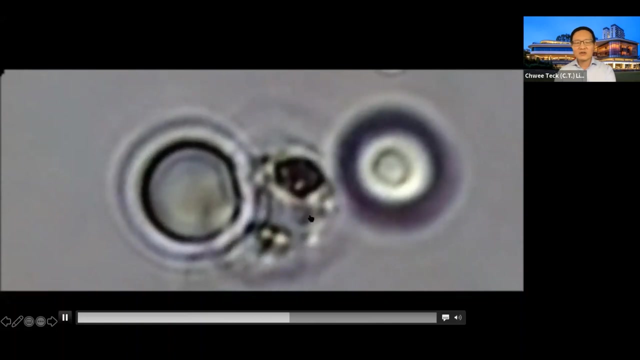 And, as you can see, the cell is still quite deformable. Of course there's already some increase in stiffness, But at the late stage when we try to stretch the red blood cell, we can hardly stretch it. So this is really a very late stage infected red blood cell. 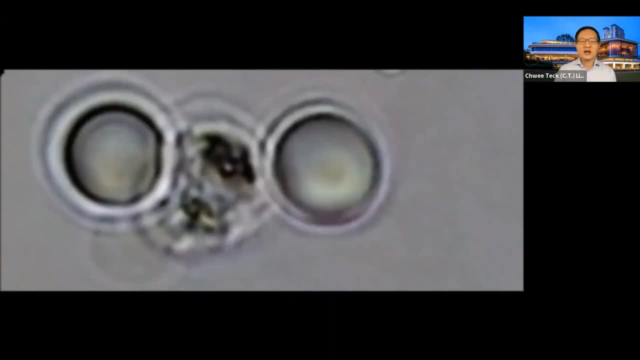 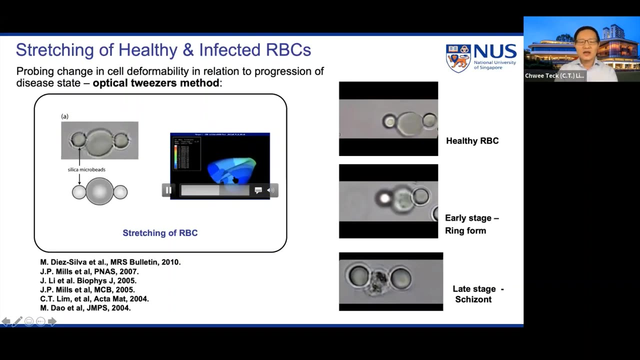 So by using the same amount of force we can hardly stretch it. So it shows how stiff the cell is. So it shows how stiff the cell has become. We also did some finite element modeling so that we can work out what the increase in shear modulus. 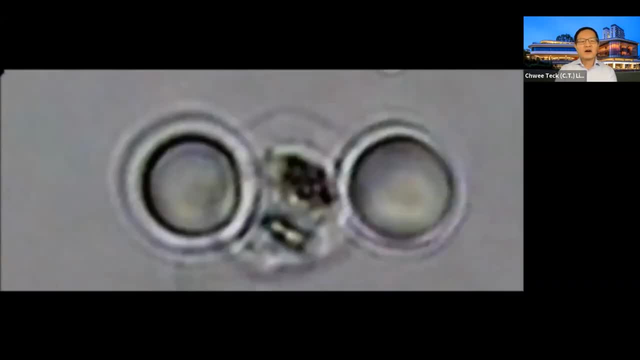 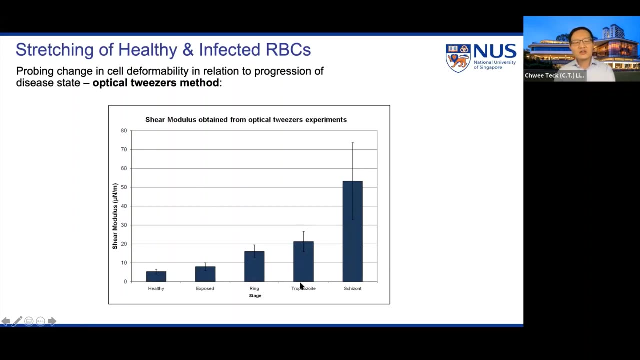 is on the membrane And from our studies we found that the shear modulus obtained from optical tweezers experiment showed that from healthy to the late stage there's about almost a tenfold increase in the shear modulus of the infected red blood cell membrane. 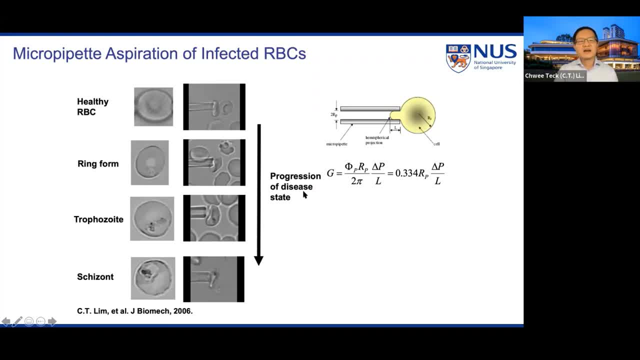 We also do other interesting experiments Like, for example, micro pipette aspiration on the infected cell. So if you look at this movie here we use a very small pipette to aspirate the red blood cell And you can see that the amount of cell 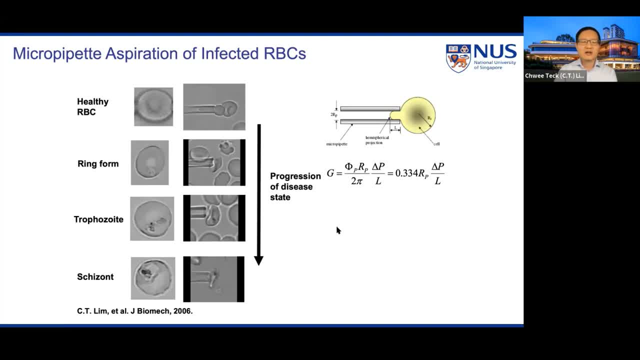 that is sucked into the pipette is quite large, So that shows how deformable the cell is. At the ring stage, where you can see there's a parasite inside the cell, you can see that the cell has started to get stiffer. 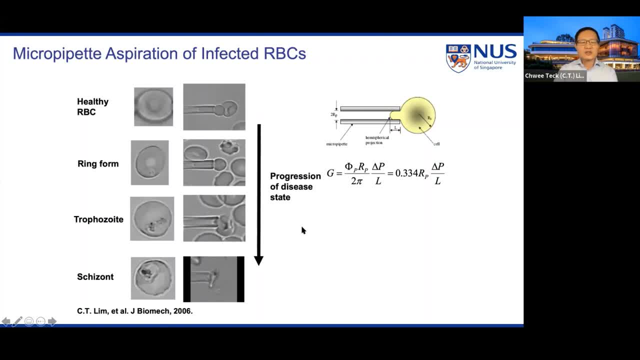 And then this is the trophozoic stage, which is the, you know the mid-stage infection, And then, at the final stage, schizon. we can hardly aspirate the cell at all. You can see how stiff the cell has become. 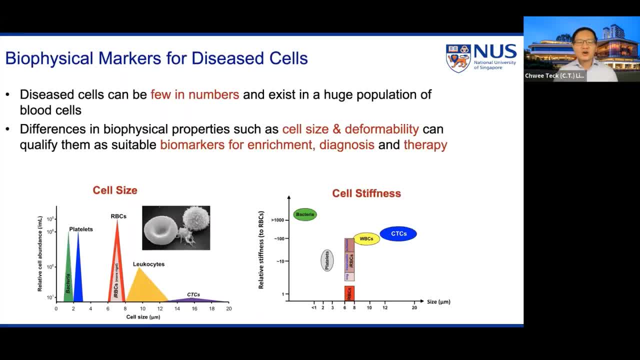 So from these experiments we also wanted to see if we can develop some way of a device that we can be able to. if we take blood from a patient, pass through our device, we'll be able to harvest or be able to detect and obtain. 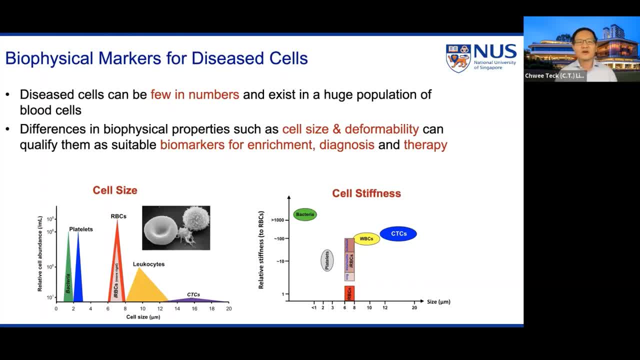 some of these infected red blood cells. So it's kind of a device that can go for enrichment and thereafter diagnosis. So we know that the number of red blood cells that's infected by malaria is actually very few. There's only a fraction of a percentage of the red blood. 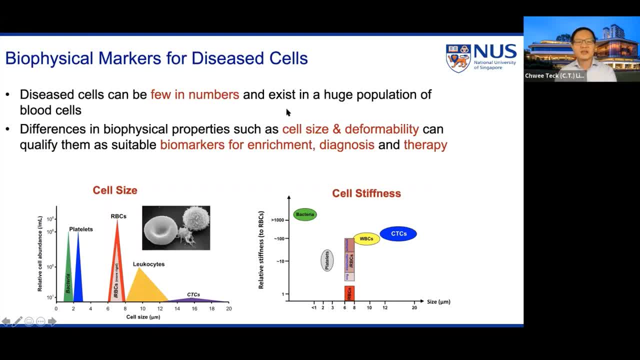 cell And there exists a huge population of other healthy red blood cells. But we do know that there's a difference in biophysical properties And, as I've shown you just now, there's a difference in terms of the deformability of the infected. 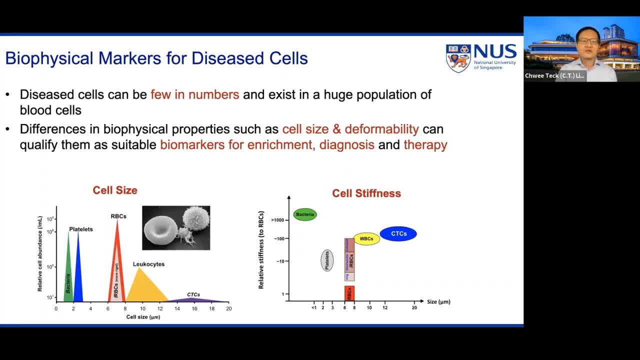 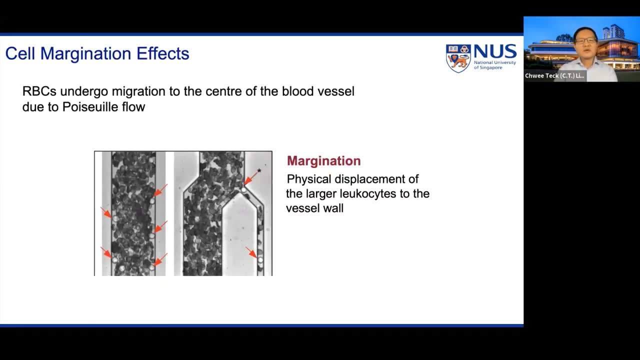 red blood cell versus healthy red blood cell. So, using the differences in this cell deformability, we think that we can use this as a biomarker for us to enrich and diagnose these malaria-infected cells. So, when we move ahead, we started to look at cell margination. 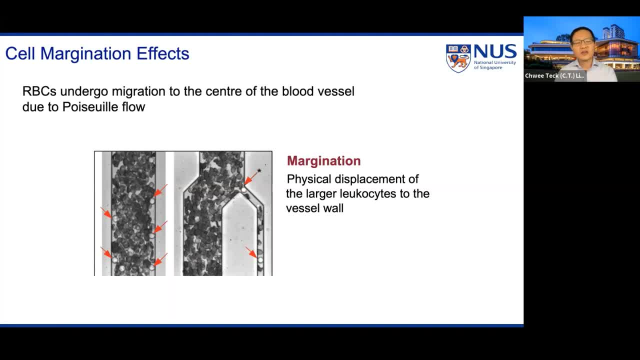 to see if we can make use of this phenomenon to isolate infected red blood cell. So we do know that when the red blood cell undergoes migration in a channel like this or in our blood capillaries or blood vessel, there is this possible flow effect. 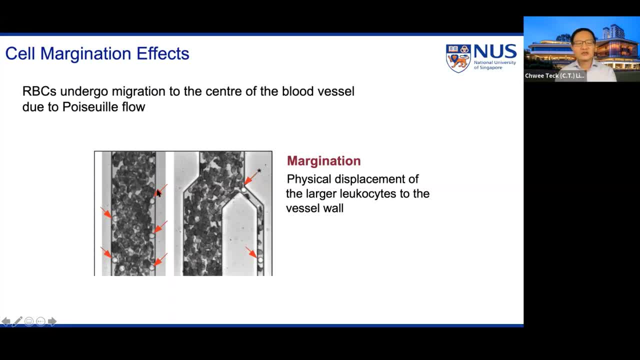 where the larger glucoside actually gets marginated to the side of the wall of the channel or the blood vessel. So we know red blood cell is stiffer than red blood cell And so if the infected red blood cell is also stiffer, 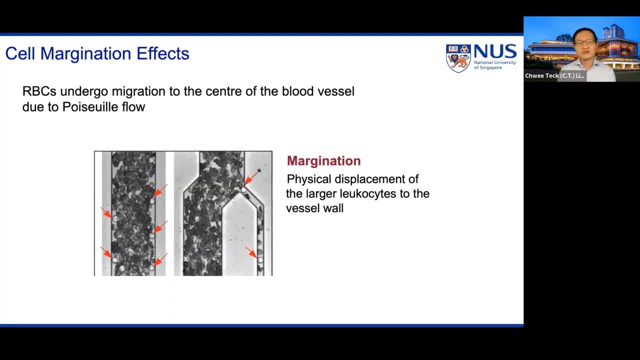 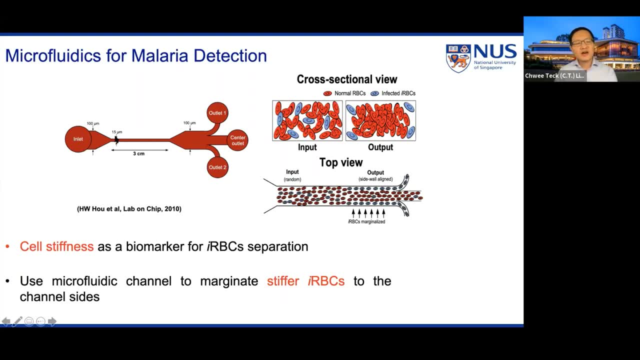 then we might be able to use this cell margination, in fact to actually push the cell to the side of the wall and thereafter isolate them. So we came up with a microfluidic device like this, a very simple, very long channel microfluidic device. 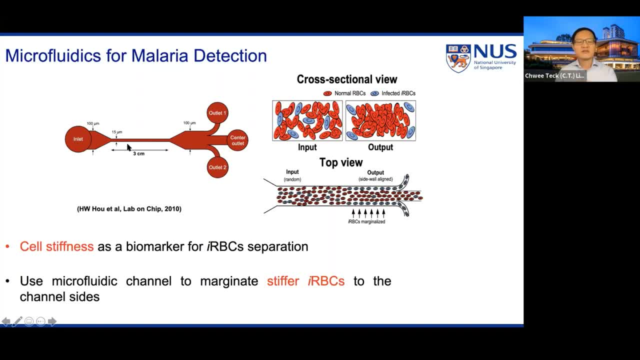 And it's about 3 cm long, but the cross-section is about 15 microns by 15 microns, And so the idea is that we can flow red blood cell in infected red blood cell And as it passes through, as it flows through this long channel, 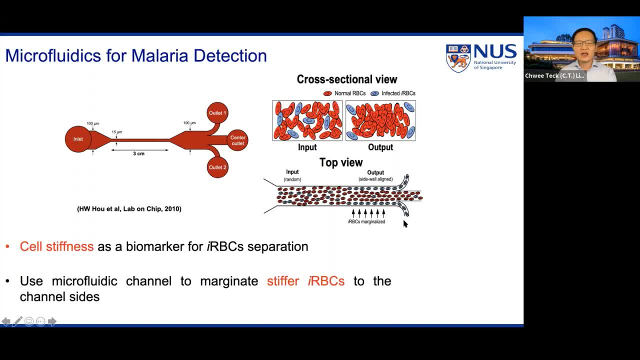 the stiffer red blood cell will get pushed to the side of the channel and thereafter we can retrieve them. So we are using cell stiffness here as a biomarker for us to separate the infected cells from the healthy red blood cells. So let me just show you a movie of what 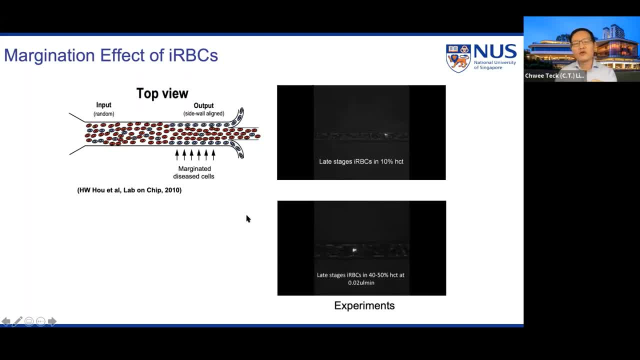 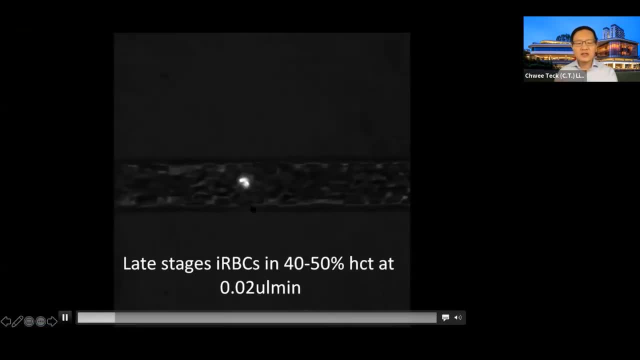 happens when we have an infected red blood cell flowing among a large population of healthy red blood cells. So you can see here, the stained cell is an infected cell And this is in hematocrit 40% to 50%, which is what we are seeing. 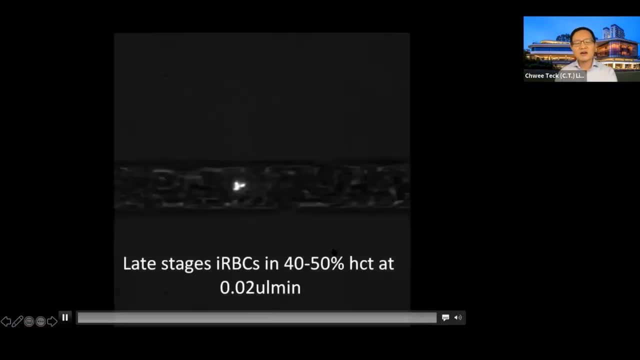 in our human body. As the infected cell flows through the channel, we can see that it gradually starts to marginate to the side of the channel. So you think from this experiment we know that the stiffer red blood cell actually will marginate to the side of the channel. 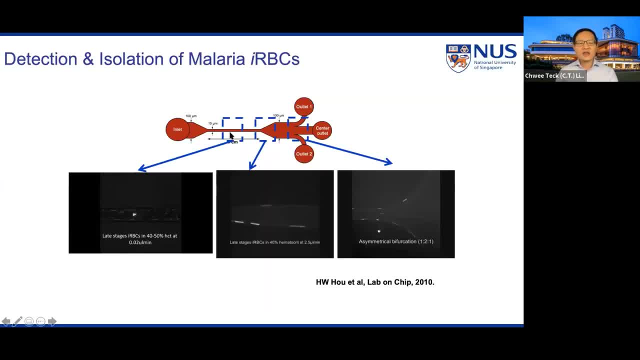 So thereafter we came up with this device to see if we can isolate them. So we do know, as it flows through, the infected red blood cell will marginate to the side of the channel. So what happens is as it comes out. 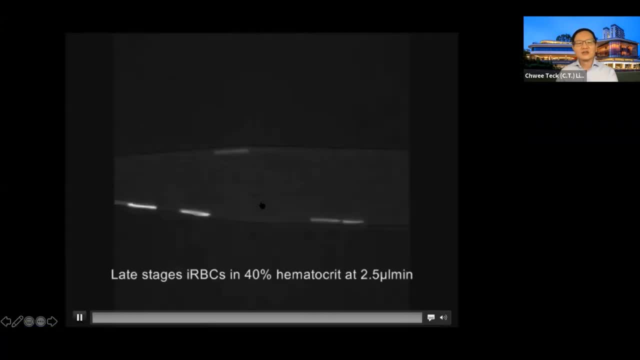 comes up over at this region. here you'll see that a lot of the infected red blood cell will start to marginate to the side of the channel, And thereafter we will be able to try to isolate them. So this is a neat way. 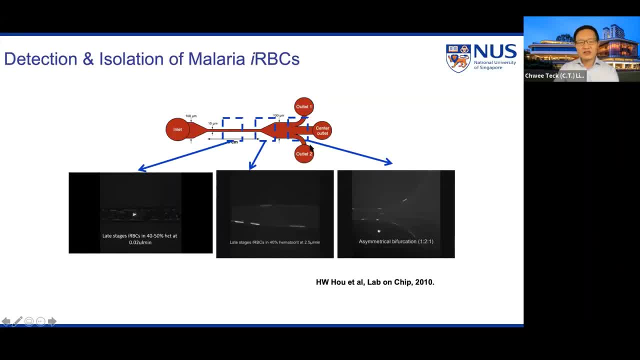 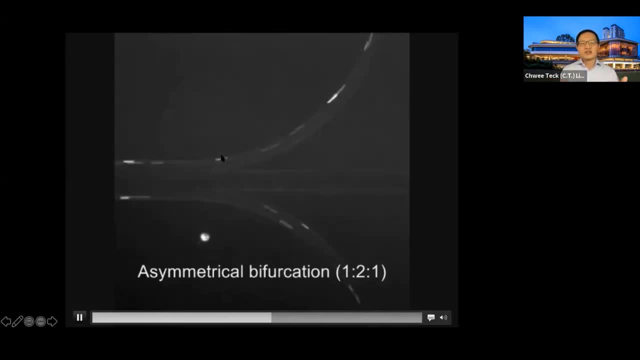 And then at the end of this device, where a lot more of the infected red blood cell will start to go into outlet one and outlet two. So this is what happens. So now you can see a lot of the infected red blood cells start to marginate to the side of the channel. 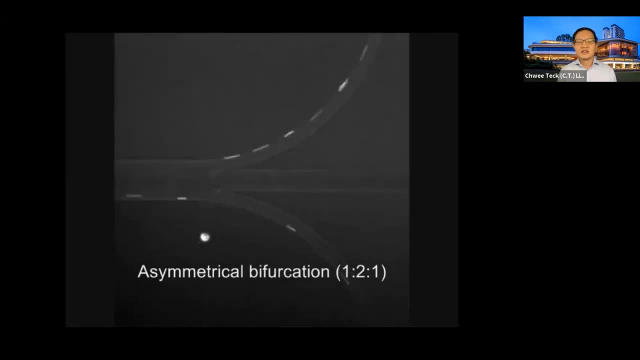 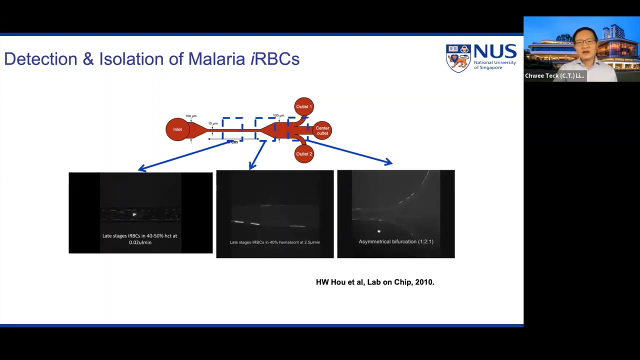 And this is one way where we can isolate the disease cells- infected red blood cells- and then send it for diagnosis. One reason why we want to develop this is also because sometimes, when we do a finger prick and we have a drop of blood on the glass slide. 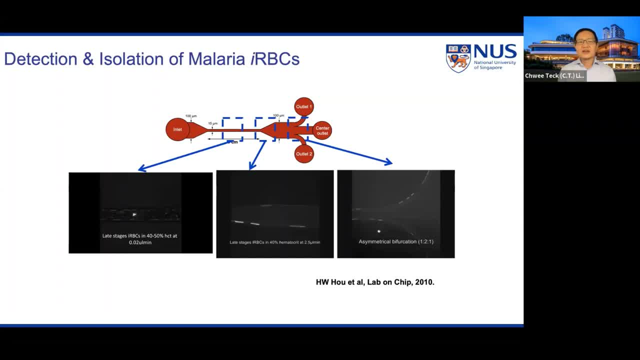 sometimes it's actually not very easy to see the infected red blood cell, And sometimes because the smear cell has multiple layers of the cell and to look under the microscope is actually quite challenging, And so, if there's a way for us to take a drop, or two drops, 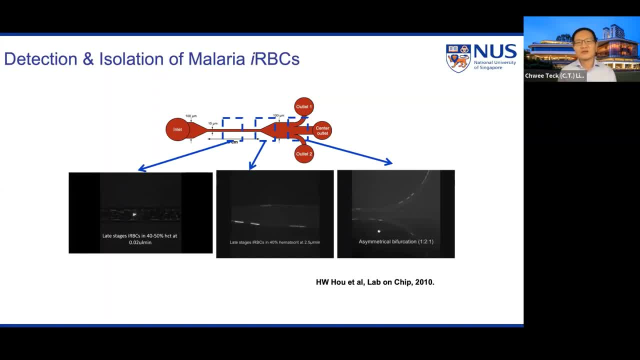 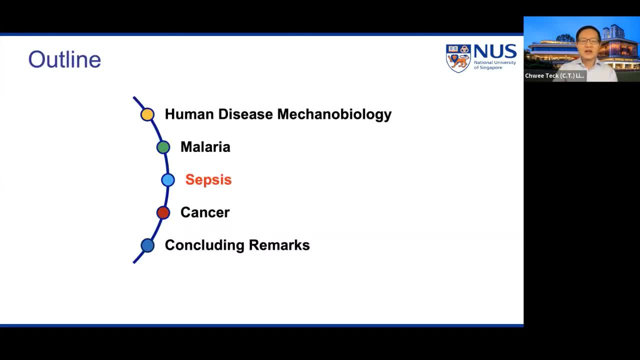 of blood from a patient, pass through a device and be able to separate the infected cells, then we have a more enriched infected red blood cell for us to look at under the microscope. So this is for malaria. The next disease I want to go to is actually sepsis. 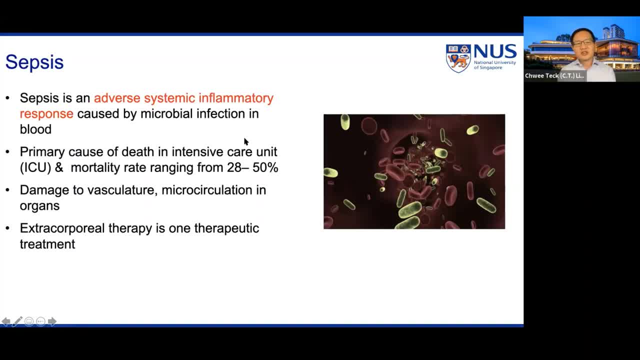 So we know sepsis is an adverse systemic inflammatory response due to microbial infection in blood, And this is actually a very serious problem because it's a primary cause of death in the ICU And, in fact, the mortality rate can range from about 28% to 50%. 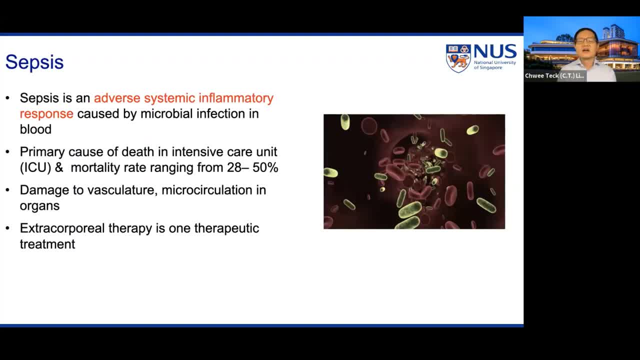 And also because of the antimicrobial resistance. a lot of these bacteria are now pretty resistant to drugs. So it's getting very hard to treat the patients And we know sepsis can cause damage to vasculature and organs as well. So one approach to solving sepsis, to treating sepsis: 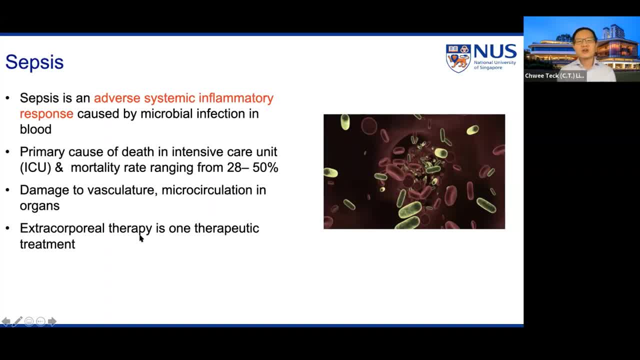 is actually through extracorporeal therapy. So extracorporeal means bringing out the blood out of the patients and then flowing through a device and then cleaning the blood before you rub the blood back to the patients. So that's extracorporeal therapy. 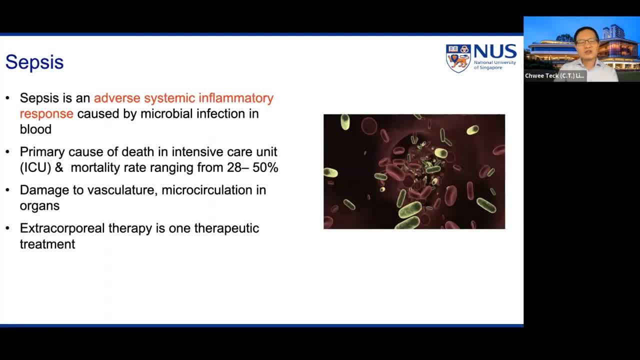 And so when we were looking at this, we felt that maybe we can also try to see if we can develop a device to be able to detect and isolate and then to remove the bacteria. So, again, we will use the cell margination effect. 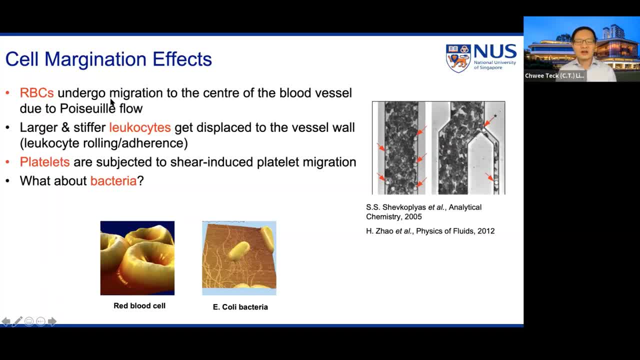 where the red blood cell will actually flow through again a channel, And then we will see if the stiffer bacteria will again get displaced to the wall of the channel And thereafter we will remove them. We know that it works for the leukocytes. 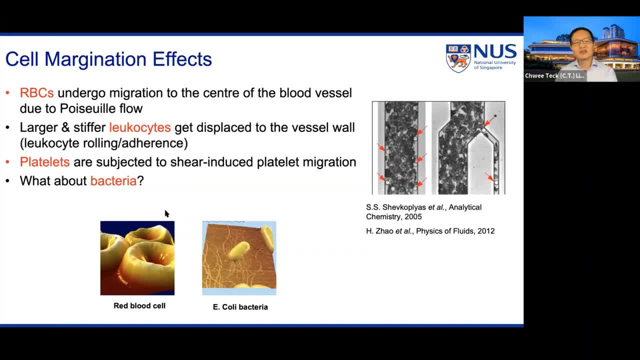 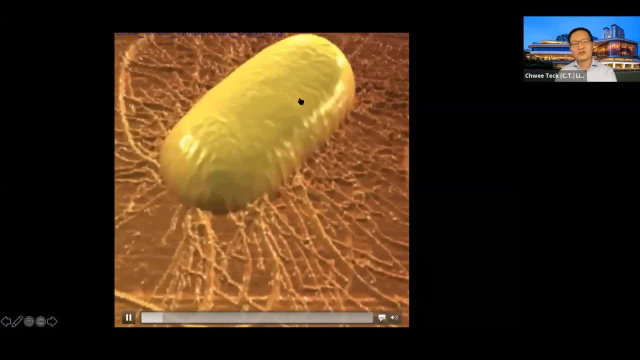 And earlier on I showed that you can work with infected red blood cells. But what about bacteria? So again we do an AFM imaging And this AFM movie shows you a bacterial. We can even see the pili and freccella. 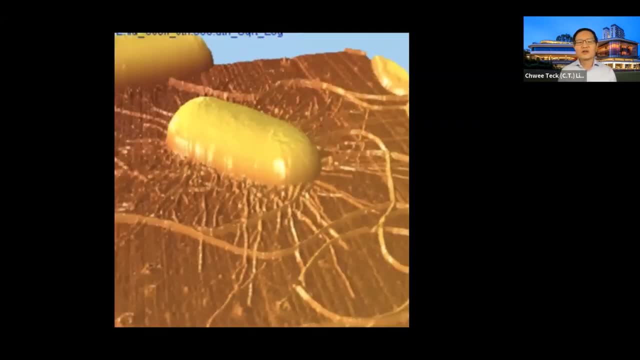 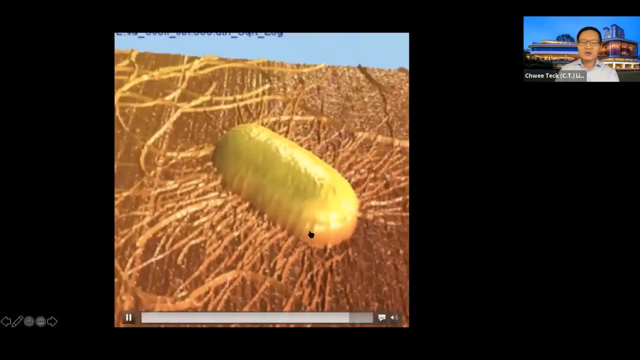 And we know the bacterial cell is a lot more stiffer than blood cells And also it has a very unique elongated shape, about 1 to 2 microns, And we just wanted to see if this works. So, again, we developed this microfluidic channel. 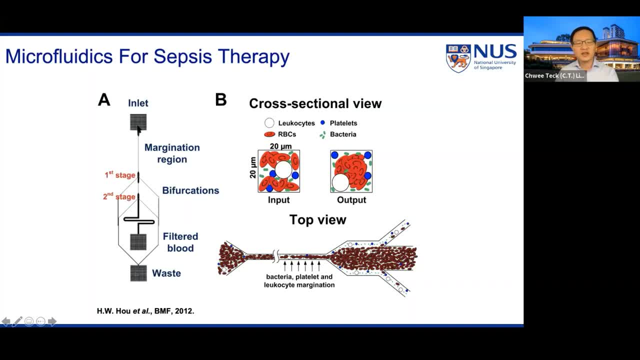 where we will have two stages of removal. The first stage is where there are the blood-containing bacteria will flow through And as it flows through the first channel, some of the bacteria will get marginated to the site. So when you get marginated to the site, 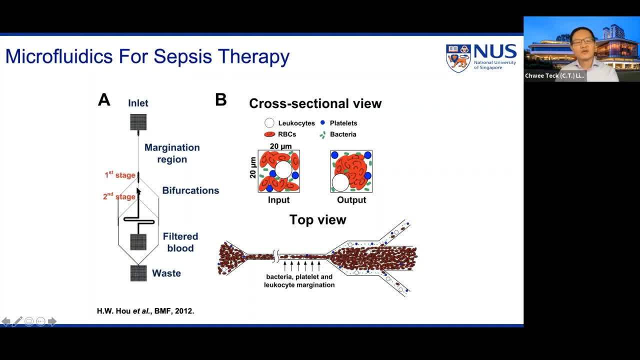 you'll go into the waste. Then there's a second stage where we will further remove any leftover bacteria from the first stage And again those bacteria will again marginate to the site and move to the waste, And then thereafter we should be able to get filtered. 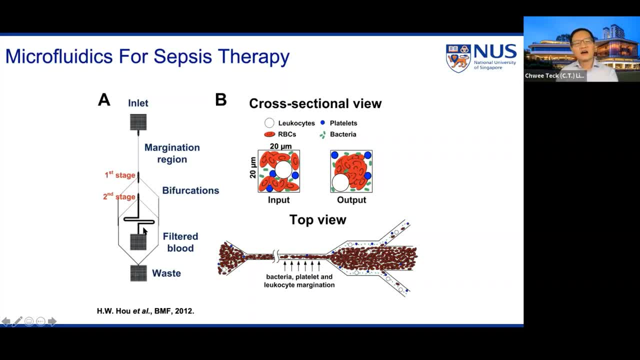 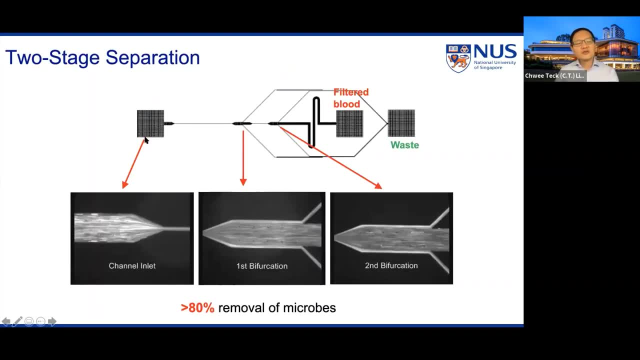 clean blood. So this is our approach to see If we can remove bacteria from blood. So let me show you what happens. So we stain the bacterias And in the first channel over here is where we input the blood with the bacteria. 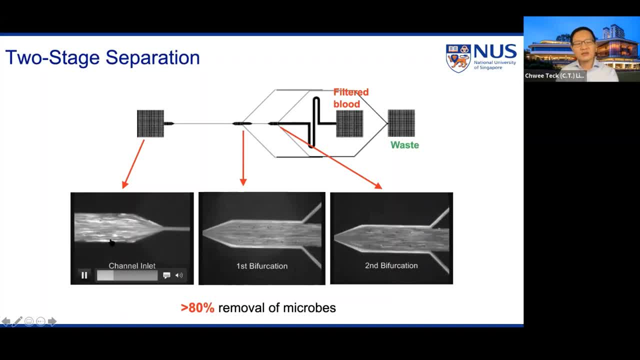 So when we first input the blood with the bacteria, you can see the bacteria is all over the place, It's body littered. So you can see there's no margination. So as it goes through the first channel, this is what happens. 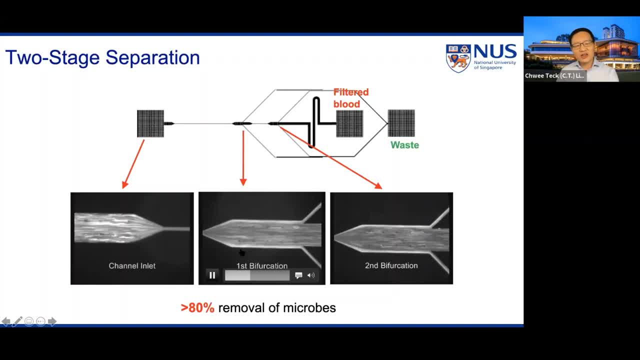 You can see that now some of the bacteria actually gets marginated to the site. There's still some bacteria in there. So this is the first bifurcation. At the second bifurcation, where we have the second stage, separation, this is what happens. 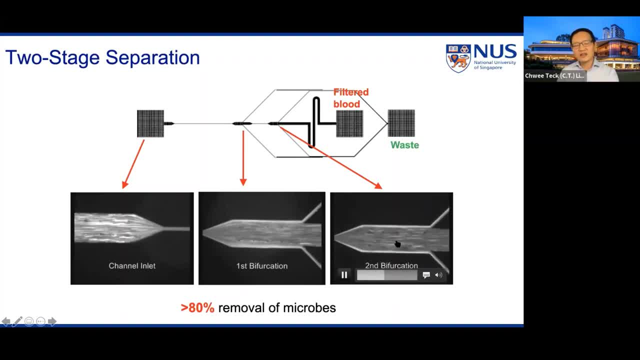 So you can see that some more bacteria gets marginated to the site And there are still some bacteria left, But the amount of bacteria left is actually a lot more lower. So there's a decrease in the amount of bacteria that passes through at the second stage. 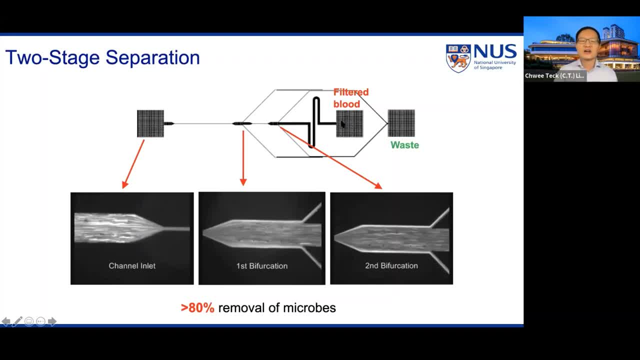 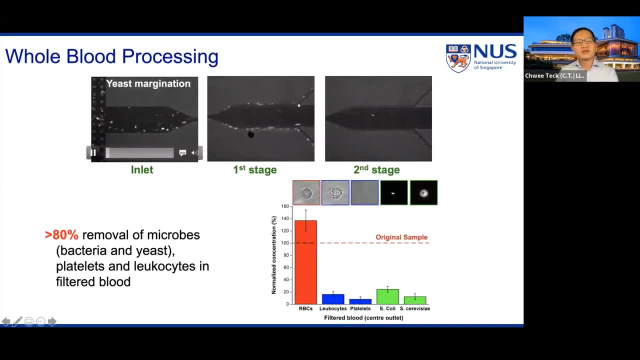 So over here is a filter blood with a smaller, lower amount of bacteria as compared to in the waste. So we also tried yeast as well And we found that we are able to also remove yeast cells from blood as well. But in general we are able to for this case. 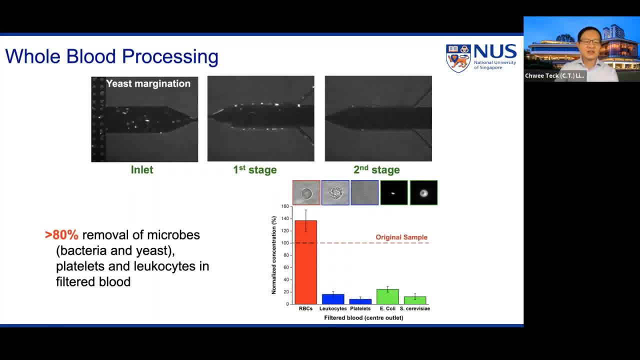 remove about 80% of the microbes of the bacteria, And so, using this device, we are able to remove quite a substantial amount of this bacteria. Of course, we can again multiply the system, And then we can And we do cleaning if we need to. 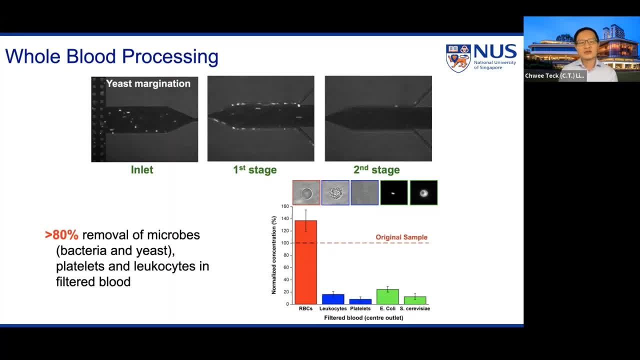 So we could in effect have not only two-stage but also three-stage to remove even further bacteria if we need to. But for this two-stage system we are able to remove more than 80% of the bacteria, But of course the system itself is very low throughput. 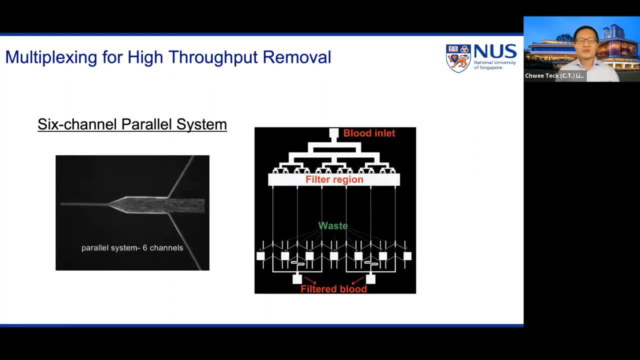 So we need to find ways to do more high throughput testing. So because I mean a human has five liters of blood in our human body And so we need to be able, We need to be able to process and remove blood in a very high throughput way. 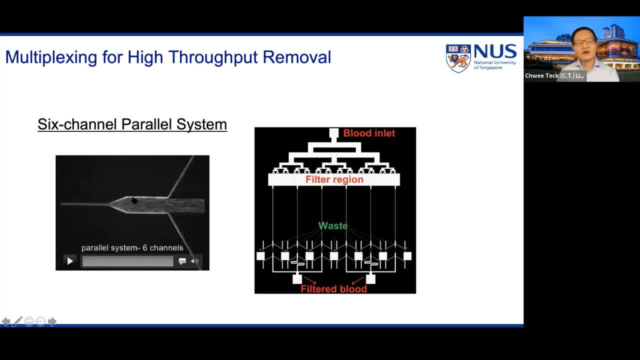 So one way is to multiplex, for example. This is just to prove our concept, to show you that we can actually be able to do a six-channel parallel system to remove blood in parallel. So right now I'm just showing you six-channel. 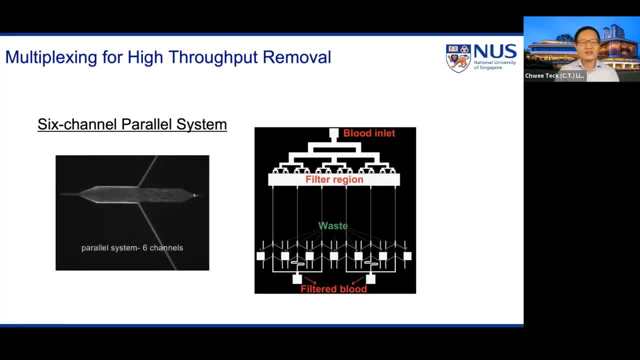 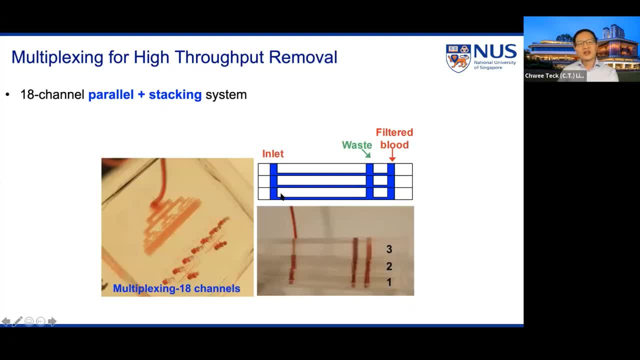 but we can literally have 100 or even a few hundred channels to increase the throughput of this removal. So in fact, we even showed that we only can do parallel, And that's actually a very good thing. And that's actually a very good thing. 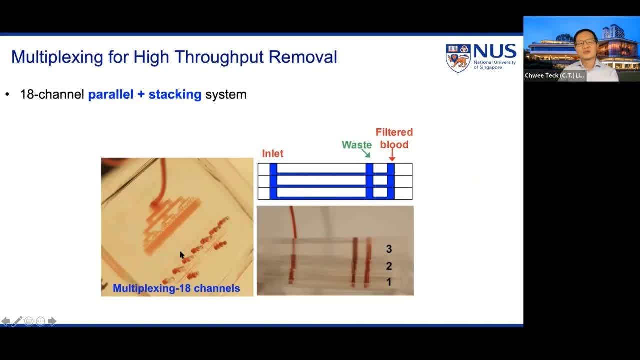 but also we stack the number of micro fluid channels as well. So over here we see a multiplexing of 18 channels, but, as I mentioned, we can literally multiplex to many more channels if need be. So this is one device we developed to show that. 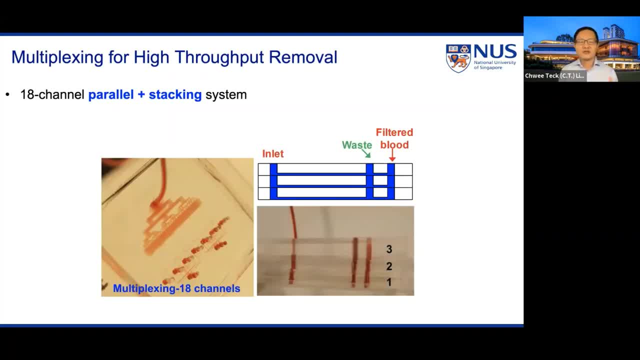 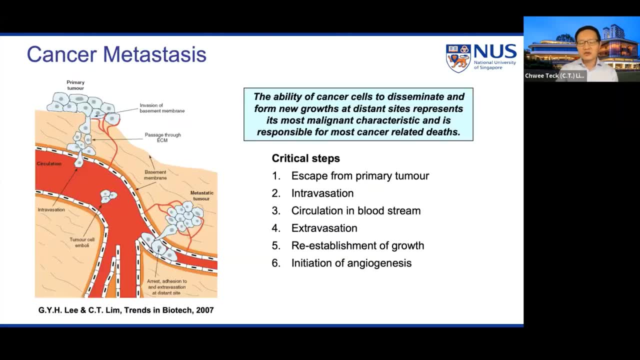 using differences in the mechanical properties of bacteria from healthy rib blood cell, we are able to actually remove the bacteria from blood of patients. So the last one I want to talk about is cancer. We know that when someone develops cancer, the cell can actually undergo uncontrolled growth. 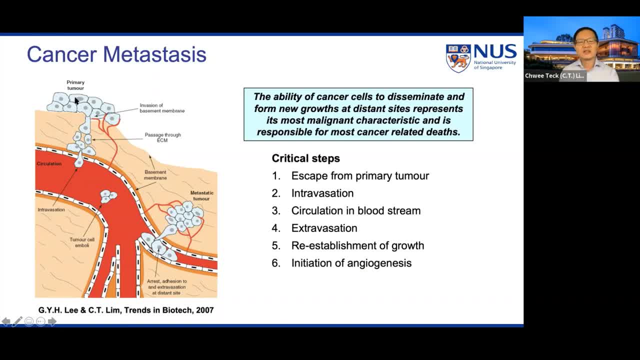 And when that happens it will develop into a tumor like this. If the tumor, if the cell, remains where it is and doesn't undergo metastasis, then it's a benign tumor. So if the patient goes for surgery to remove the tumor, 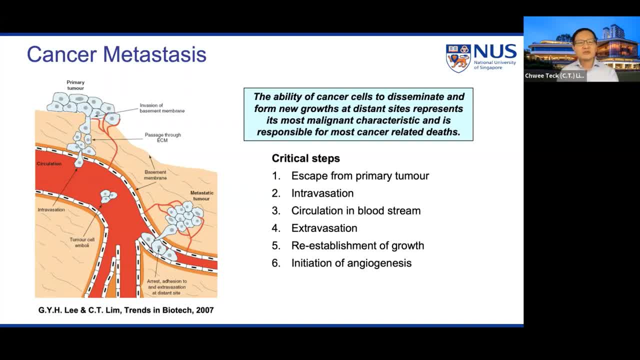 the patient will recover from it. However, the ability of the cancer to disseminate and for to form a new, new secondary tumor at distant site means that the cancer cell has become malignant And, in fact, metastasis is responsible for more than 90% of cancer deaths. 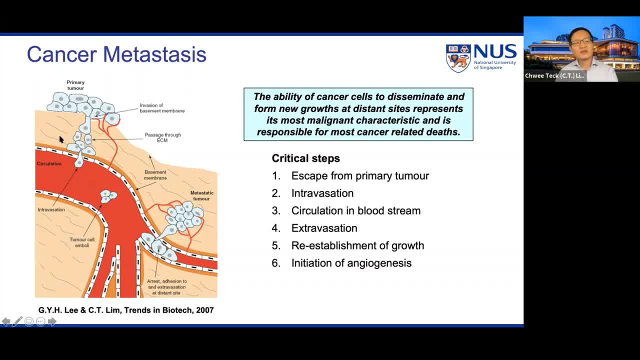 And so so it's a very important disease for us to look at and to understand the whole cancer metastas, PTSD, full cell metastasis process. So what happens is, if a cell becomes malignant, it is capable of detaching from par, it is able to squeeze its way. 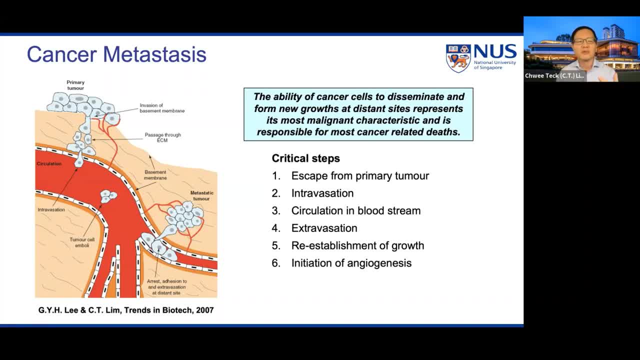 into the circulatory system and it can move from one organ to the next organ. For example, from breast it can move into bone and then it can squeeze back to form secondary tumor like this. So there are a number of critical steps. 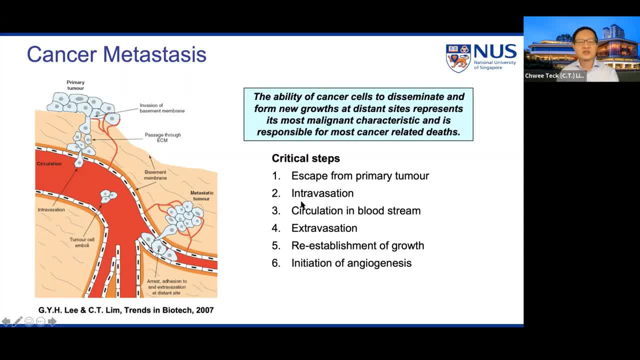 from escape from primary tumor to intravasation to circulation in the bloodstream and then eventually extravasation and then establishment of a secondary growth and then thereafter initiation of angiogenesis to form a metastatic tumor like this. So this whole process is actually very mechanical. 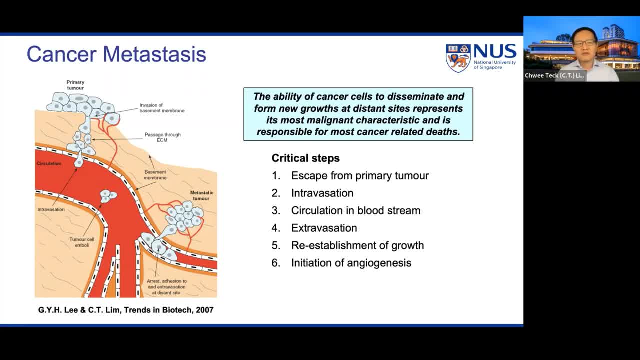 because, firstly, the cell will become more deformable, it will actually lose its adhesion, and thereafter it's able to detach from primary tumor and squeeze its way into the circulatory system, And so we want to understand how this can enable the cell 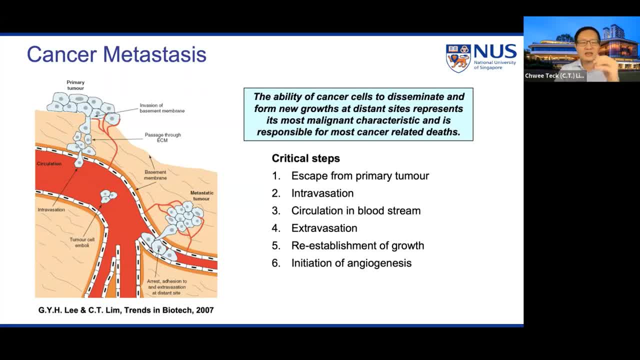 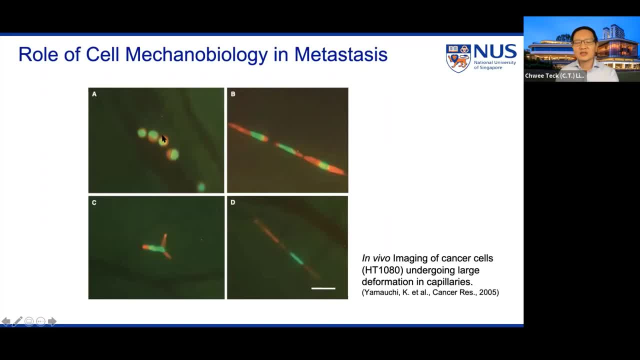 to undergo such metastatic cascade, So when we will? now there are already. I'm just showing some of the cells. for example, this is an in vivo imaging of cancer cells undergoing very large deformation in capillaries of mice And you can see that some of the cells 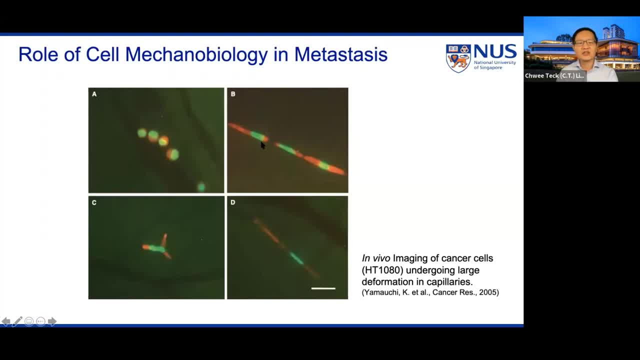 literally have to undergo large deformation in capillaries, and you can see, the nucleus itself also plays a very important role because they get excessively deformed. And yet, despite this large deformation, the cell will still be able to traverse through all these capillaries. 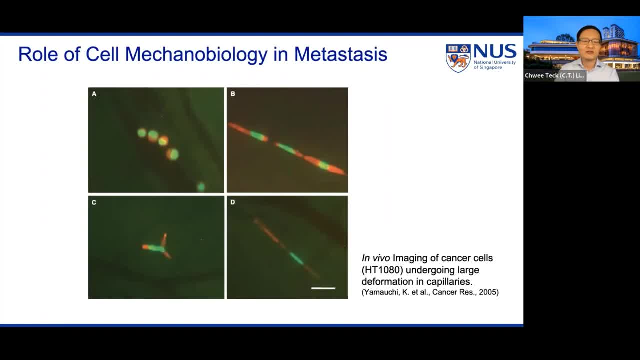 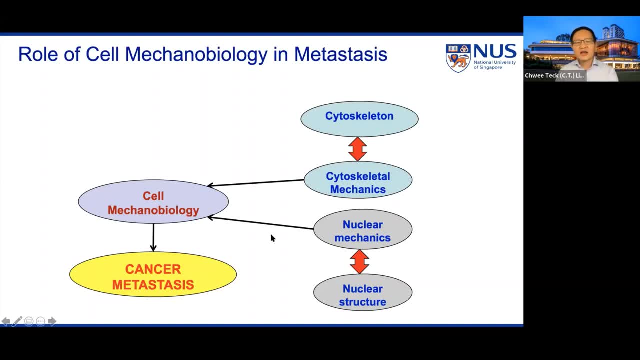 to reach to its final destination, to form secondary tumor. So it means that the role of cell mechanobiology is actually very important in metastases, And so there are two parts to it. One, what constitutes a cell, mechanical properties. One is actually cytoskeletal. 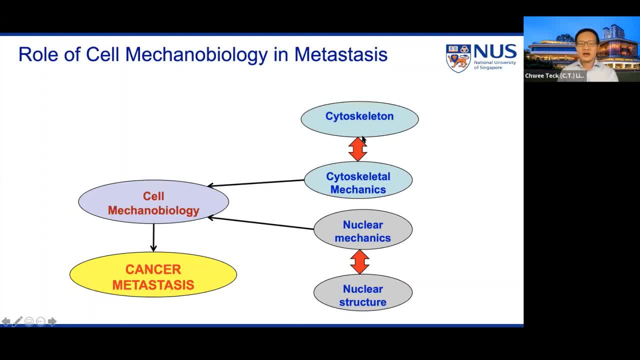 The cytoskeleton itself which leads to the cytoskeletal mechanics, And secondly it's the nucleus itself. So nuclear structure, of course, will determine nuclear mechanical properties, and both cytoskeletal and nuclear mechanics will actually determine how. 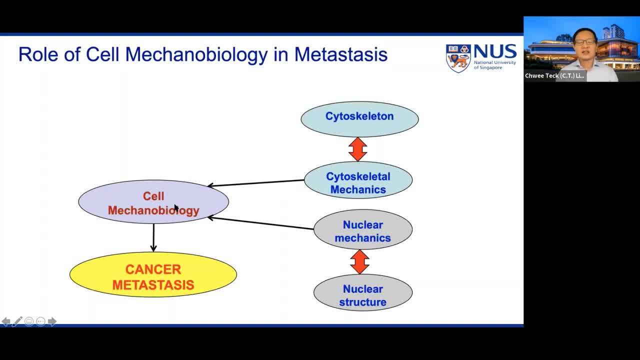 this CES will work: cell mechanobiology in the sense how cancer cell will respond to its external environment and be able to know further undergo metastasis. So in our lab we actually perform many different tests. I don't have the time to go through all. 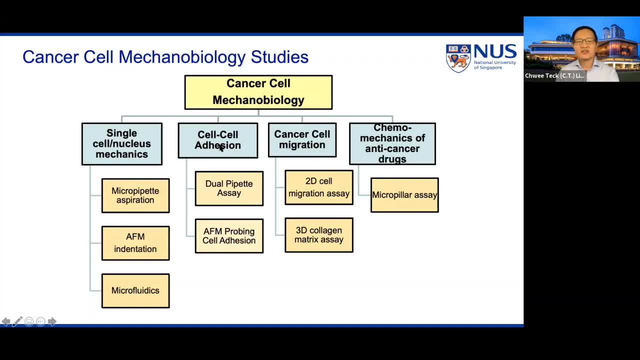 of them. We did single-cell nuclear mechanics to cell-side adhesion, to looking at cancer cell migration and even looking at chemo mechanics of anti-cancer drugs. I'll just focus on the single-cell nuclear mechanics and then show you some of the devices and technology visualized to detect cancer. 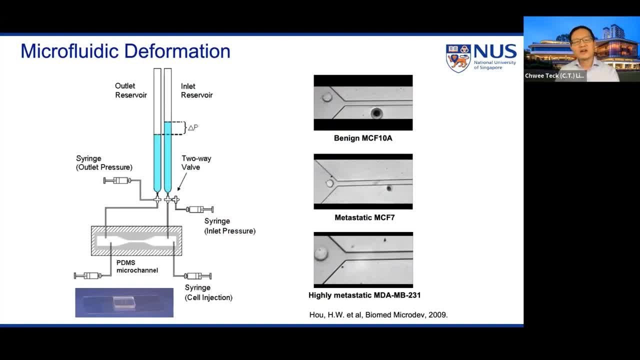 So one of the interesting experiments when we first go into this area is looking at deformability of cancer cells using micro fluidic channel. So this is mcf10a, which is a non-cancer cell. If you look at the cell itself as it goes through a 10 by 10 micron channel, it takes a. 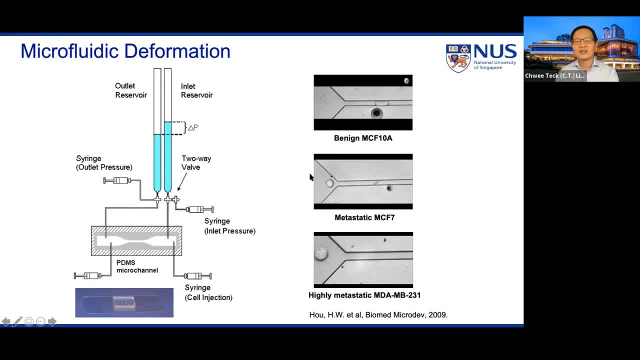 pretty long time to go through a channel like this For a metastatic mcf cell, which is a breast cancer cell. If you look at the cell itself, the time taken to traverse through the channel is much faster compared to the MCF10A. 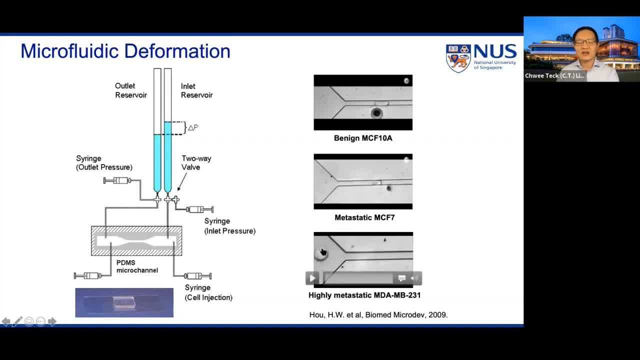 For the highly metastatic MDA-MB231 cells the time taken is even faster. So you can see that again, benign cell takes a longer time, metastatic MCF7 takes a slightly faster time and then the hydramethic cells is even more faster. 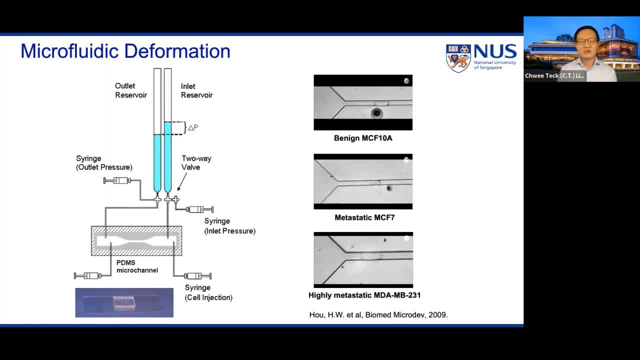 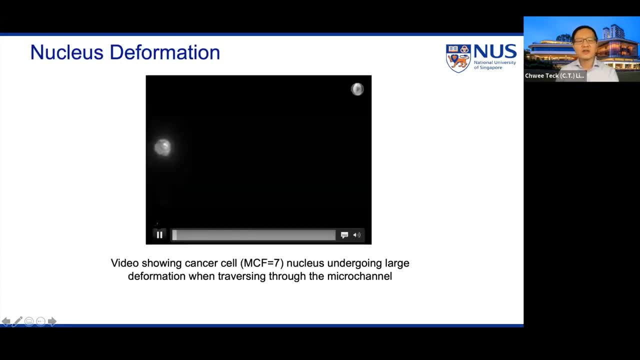 So it shows that actually the magnetic cells are much more deformable. And of course we also did look at the nucleus deformation. So if you look at this video here you can see the large deformation on nucleus undergoing deformation through a very narrow channel. 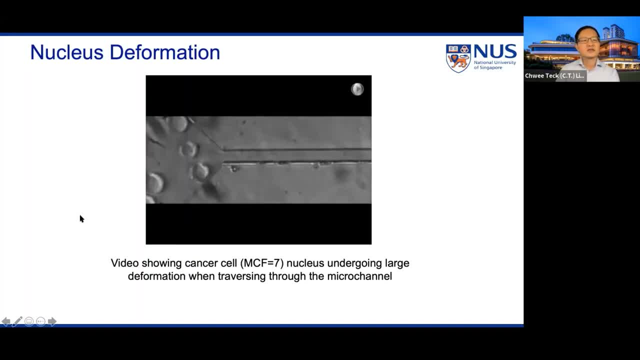 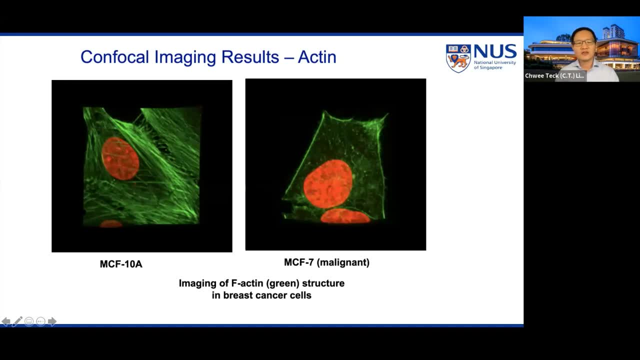 like this. So nuclear mechanics is also very important, the mechanical properties, And of course we did quite a number of different experiments, both looking also at the doing confocal imaging to look at the cytoskeletal structures of cancer cells. So this is a MCF10A- again non-cancer cells. 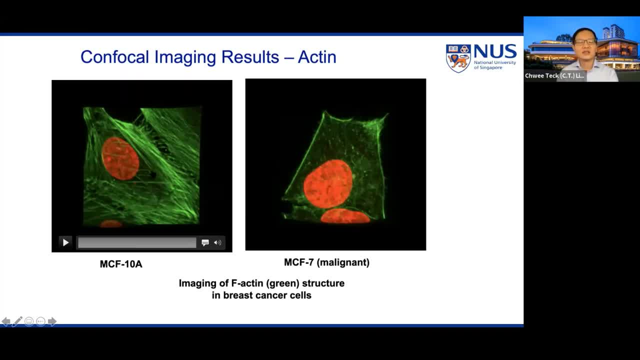 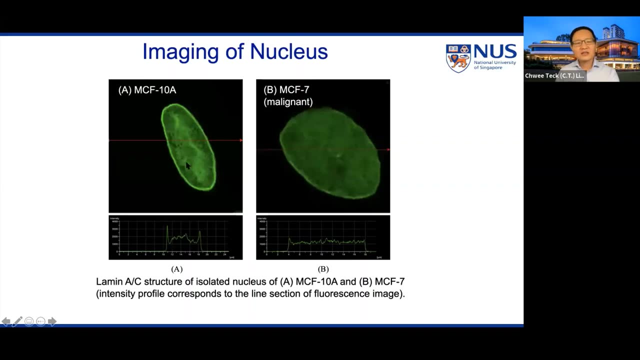 You can see very well formed F-actins within the cells, as compared to MCF7, where the actings are a bit more disorganized and not so voluminous. Of course we also look at nucleus as well, where for the non-cancer cells? 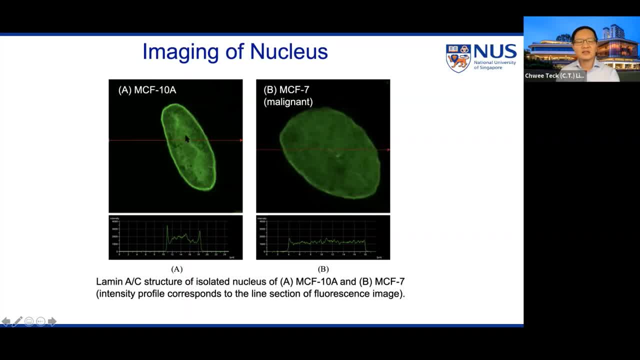 and versus the MCF7 cells. the same AC structures are much more well defined and a lot more expressed in the non-cancer cells versus the MCF7 cells. So that shows also why the non-cancer cells- actually non-cancer breast cells- takes a longer time. 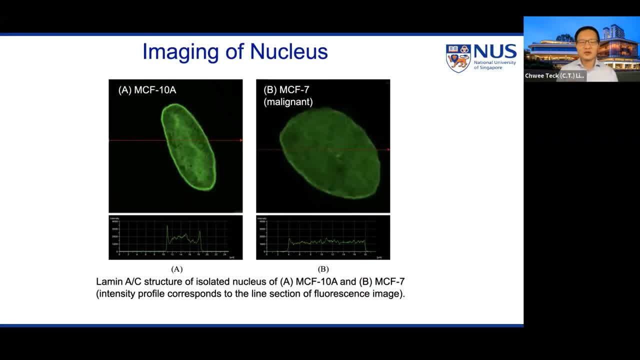 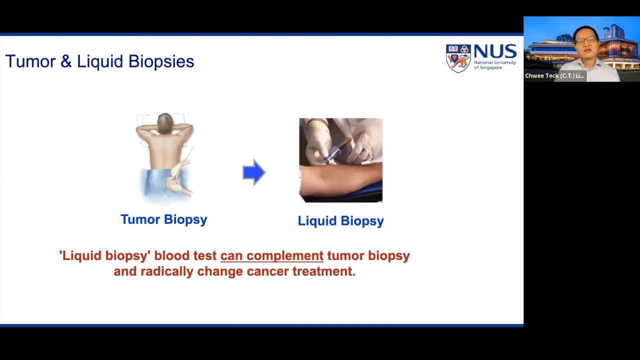 to actually squeeze through a narrow channel. I mean, if you were to look at how the nucleus actually deforms and occupies the whole channel. this is also one contributing factor to it being much more stiffer than the, the cancer cells. So we did quite a bit of these different studies. 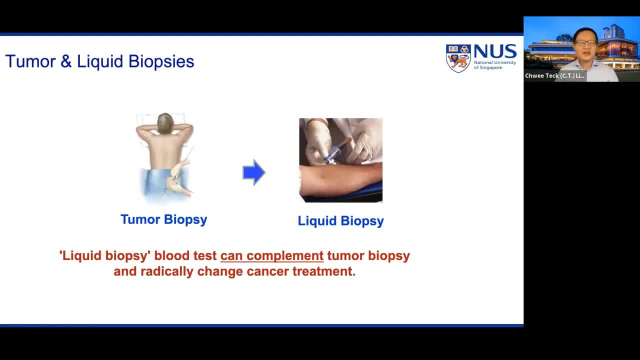 and then when we were talking to clinicians that they actually was very interested to see how we can use our understanding of this cell mechanics, to see if we can use it to detect and diagnose diseases, diagnose cancer. So we started to look at how clinicians do cancer diagnosis. 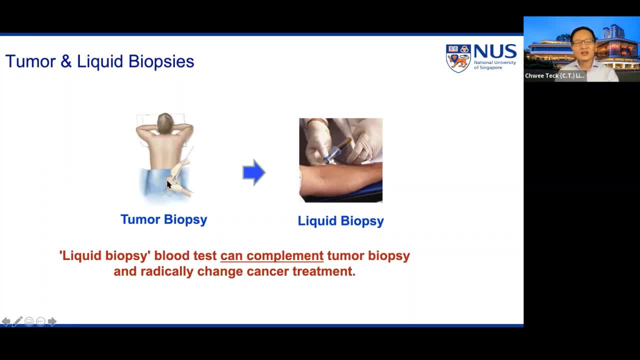 is to tumor biopsies, where you take a sharp needle you poke through the body to sample cancer cells from the patients. so we know this procedure is very invasive. it's very painful. you cannot do it frequently. normally do it once before chemotherapy treatment and once after chemotherapy treatment. 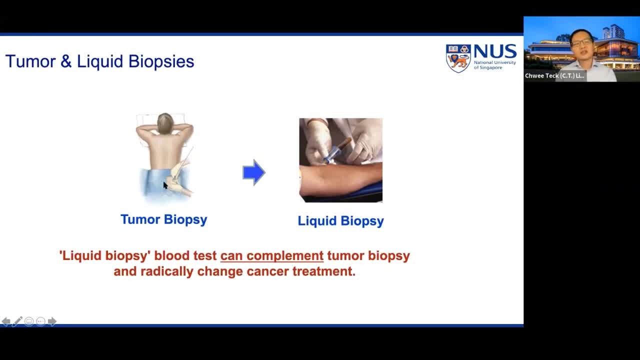 uh and and so so. so in the course, when the patient is undergoing treatment, there's no way for us to sample cancer cells to see if you know that, for example, the tumor has string. uh, or what has happened to cancer cell? have they been destroyed by the, by the anti-cancer drugs? so uh, but we also 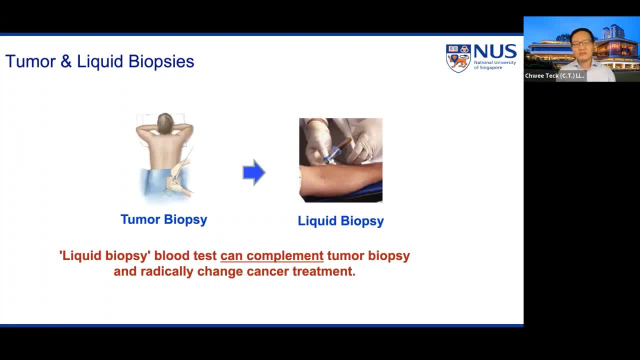 know, as i pointed out just now, that cancer cells do uh metastasize through the circulation system. so is it possible for us to actually be able to capture cancer cells from blood, which is what we call liquid biopsies, rather than from tumor boxes? so idea is that, if you can do, 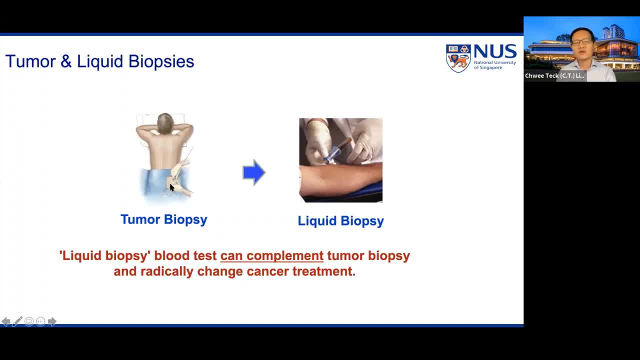 liquid biopsies, then they can complement tumor biopsies as well and hopefully change the way cancer has been diagnosed and treated. because if you can look liquid biopsies, it's non-invasive, it's not so painful and in fact you can do it quite regularly. you can do it every two weeks. 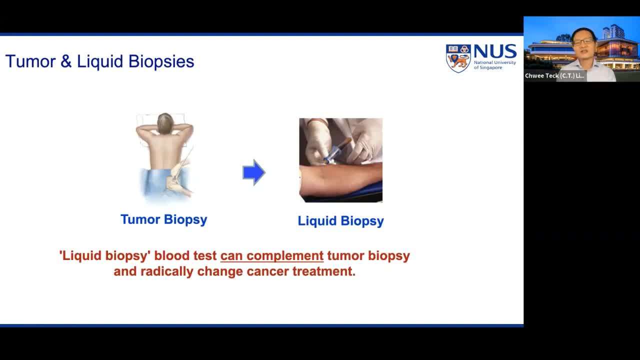 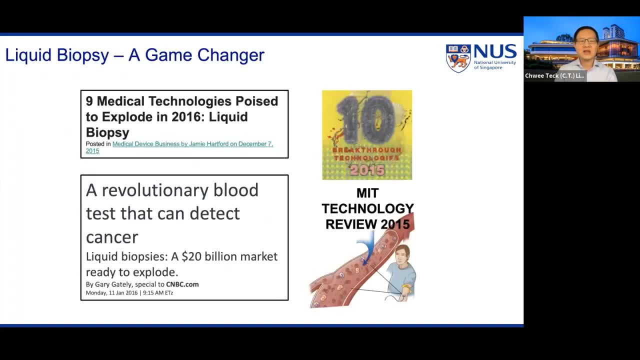 or every month, uh, to track, uh, the status of the patient with regard to the, the, the metastatic cancer cell that's circulating, circulating in the human body. so, in fact, liquid biopsy itself actually is quite a hot area. when we first started this research about 15 years ago, it was still very new, but in the last five years, there's a lot of work now being 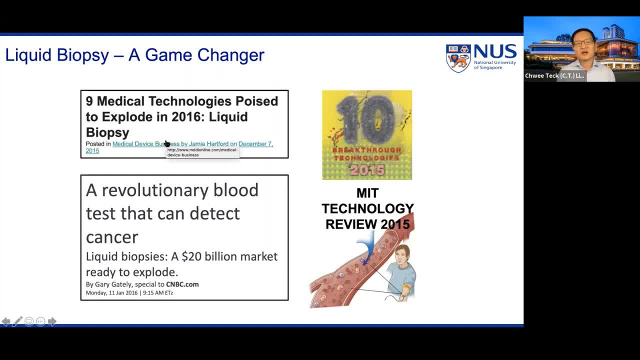 done to perform liquid biopsies, not just capturing cells, but also, uh, the cell-free dna associated with cancer, and people are now also looking at exosomes as well. it's a game changer because, uh, if, if this really works, then this will become kind of a standard test that we can actually do in a 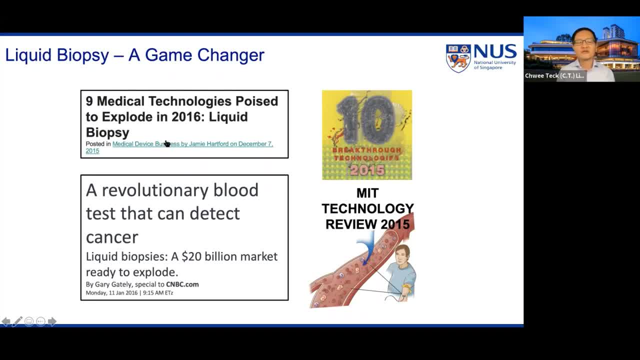 clinic or hospital very easily, because it's just doing a blood drawing from it. if you can isolate the cancer cells, then we can analyze those cancer cells, so so, so liquid biopsies, i would think maybe yes will become a standard test, because i think a lot now data are coming up from this. uh, this work. 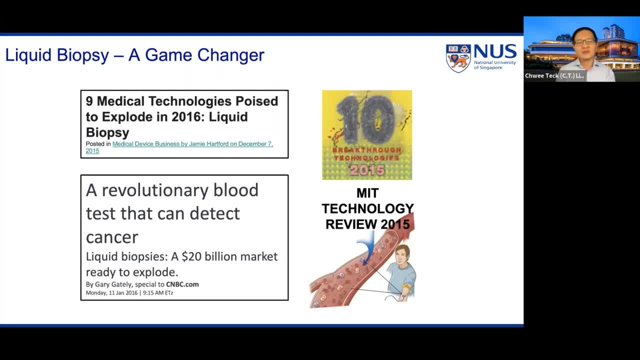 and i think it's pointing to the fact that now we are able to actually be able to, for example, determine mutation in patients from such, from such a a test, a liquid biopsy test. but of course it has a lot of challenges if you're trying to liquid biopsies because, uh, for example, if you're going 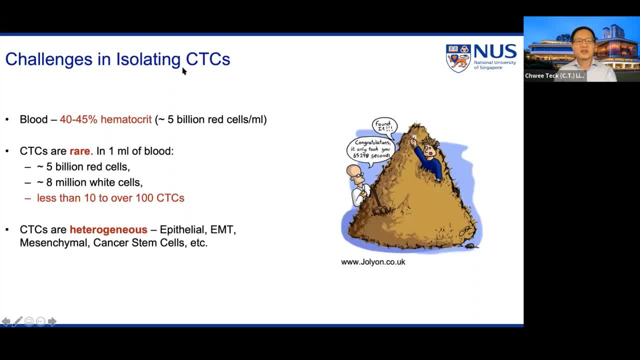 to try to isolate the cancer cells, or we call it circulating tumor cells. uh, it's actually very important to be able to do that, because it's very important to be able to do that. because it's very important to be able to do that because in blood we have 40 to 45 percent hematocrit. but cancer cells are very rare. in one ml blood there are five million red cells, eight million white cells, but they are about less than 10 to over 100 cancer cells. and what makes it even more challenging is that cancer cells are very heterogeneous. some are epithelial, some are. 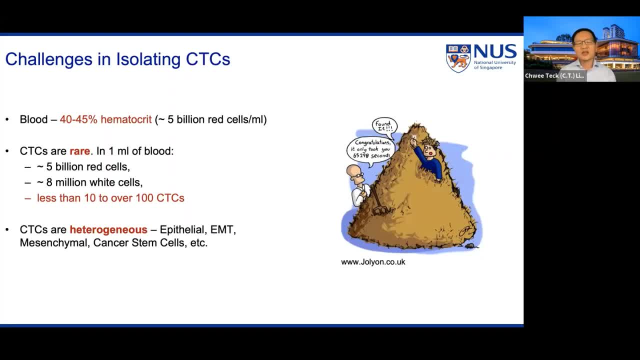 undergoing epithelial mesenchymal transition. some are actually cancer stem cells and so, uh, if you were to use antibody to capture them, then you may, only can. you may only capture a sub, a subpopulation. they all express very different proteins on the surface of the cancer cells. 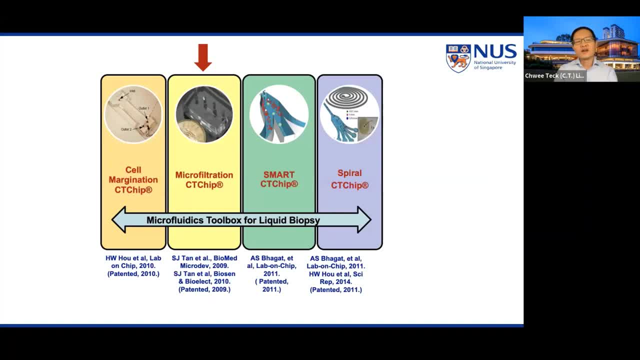 so for us, we, we, we try to do away with using antibodies, but instead use the difference in mechanical properties of cancer cells from blood cells to isolate the cancer cells. so we develop a suite of microfluidic- uh, you know- chips to do that. there are four of them. 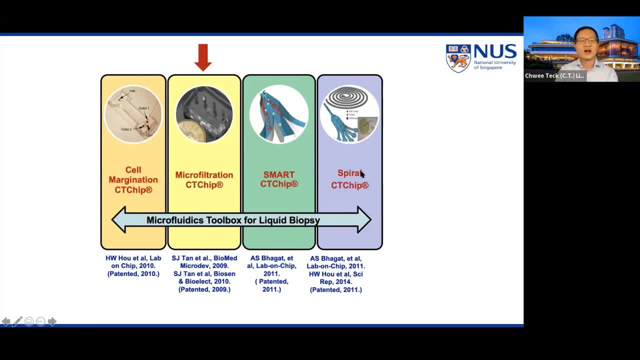 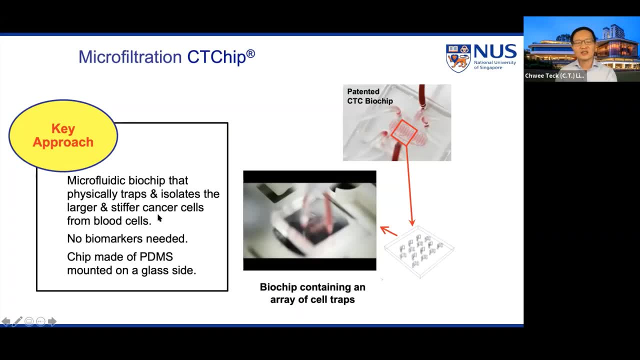 but i'll just show two. one is the microfiltration and second is a spiral. so in the microfiltration what we try to do is to be able to physically trap and isolate the larger and stiffer cancer cells from blood cells. and this is how the chip looks like. it's a pdms chip that's mounted on the. 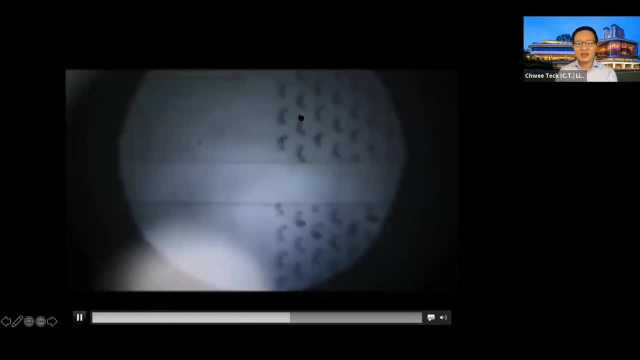 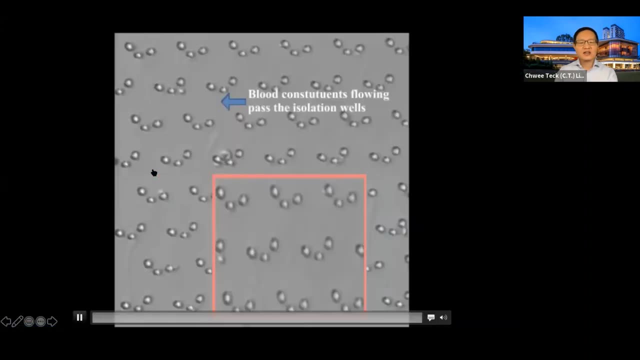 glass slide and inside the chip are these semicircular traps that can actually track the cancer cells. so so how it works is, uh, inside the chip are these three micro pillars that's sticking out, and if you look at this uh, this uh figure here movie here, you can see that the 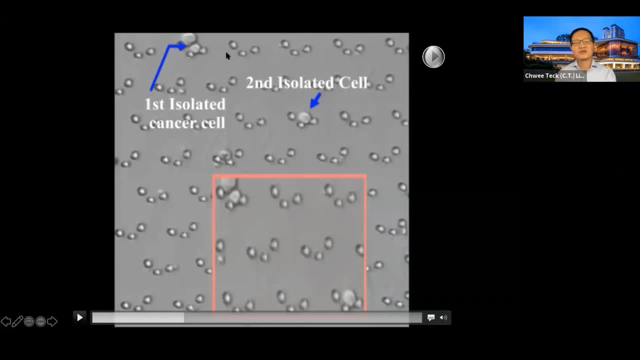 traps are somewhat. some of them are tilted slightly to the left, some are tilted to the tilted slightly to the right and they are staggered. And in this chip there are about 14,000 of these microtraps And in these three pillars itself, 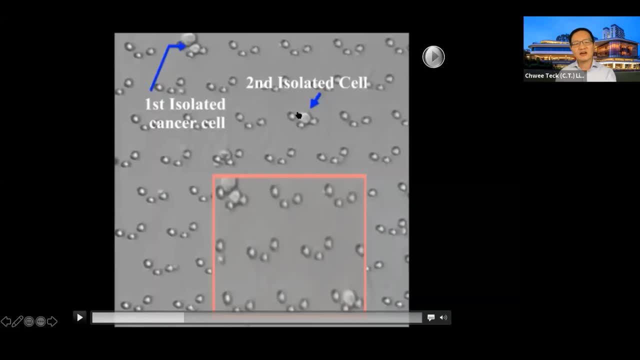 they're placed about eight microns apart, So if there's a cancer cell that's larger and stiffer, you'll get trapped like this, Whereas the red blood cells and white blood cells being smaller and more deformable, they'll be able to squeeze through these pillars. 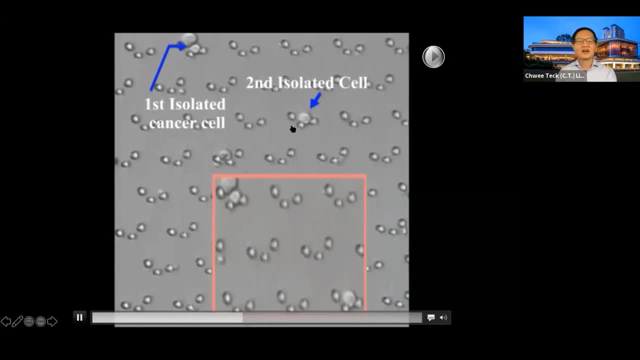 So from this movie here you can see that there are cells that get strapped like this, And so from this device we're able to trap the cancer cells as we flow the blood through this device, And so we just show you how it works. 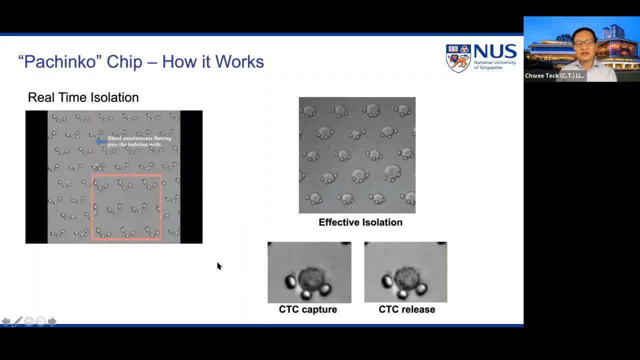 when the cancer cells come and encounter three pillars like this, It's stiffer, it will get strapped. Then, once the cells are all trapped, what we can do is we can then reverse the flow to isolate the cancer cells. So over here to release the cancer cells. 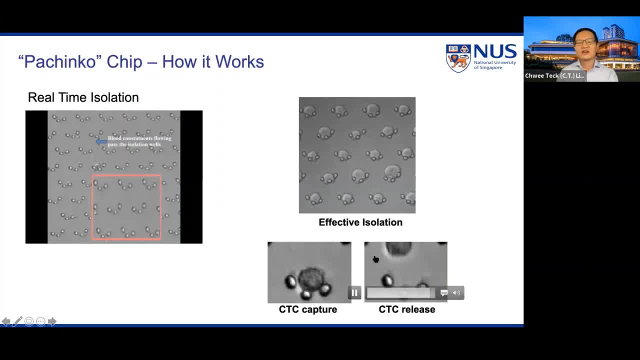 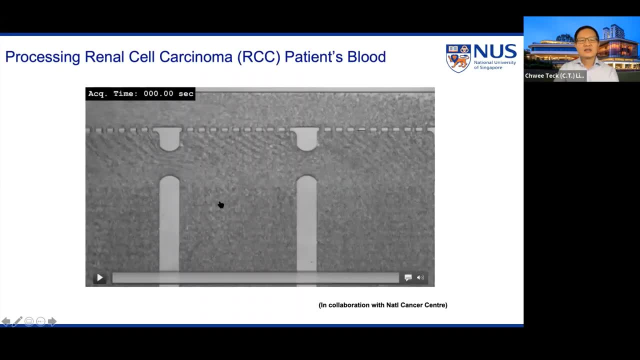 we can reverse the flow and then we are able to We release and then be able to retrieve the cancer cells And then after we can do the analysis, Just to show you processing of actual patient blood. this movie shows you the huge amount of blood. 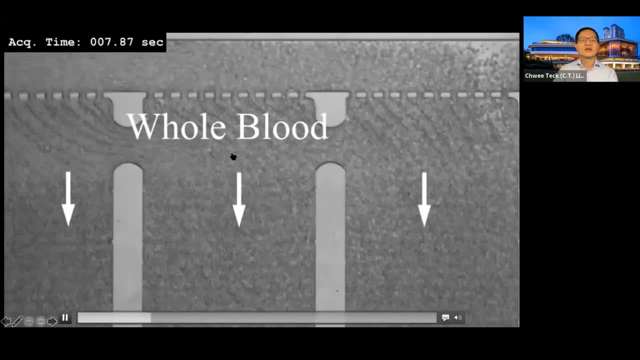 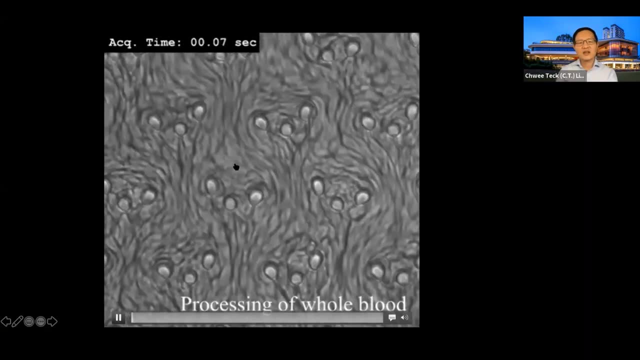 that we are processing from patients. You can see there are so many red blood cells, But I will show you a close-up movie of some of the cancer cells that get strapped. So again, in this movie there are all the red cells and white cells flowing through. 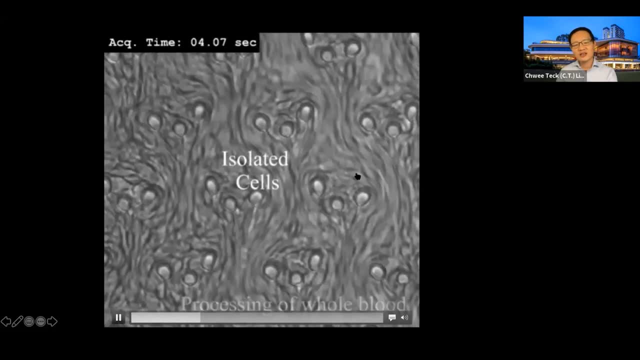 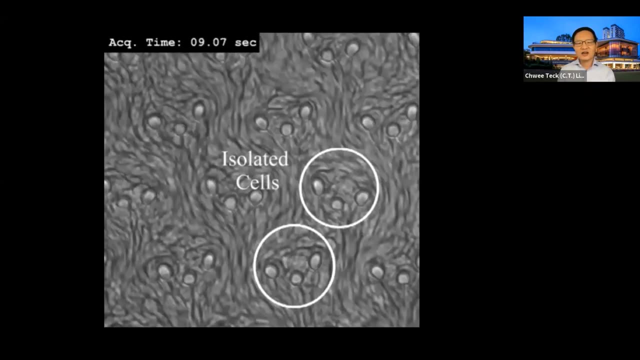 But if you look very carefully, among the three pillars here, there's actually a cancer cell over here. There's also another cancer cell here. So this movie shows you that, despite the fact that there's so much cells flowing through this, we are still able to capture the stiffer cancer cells. 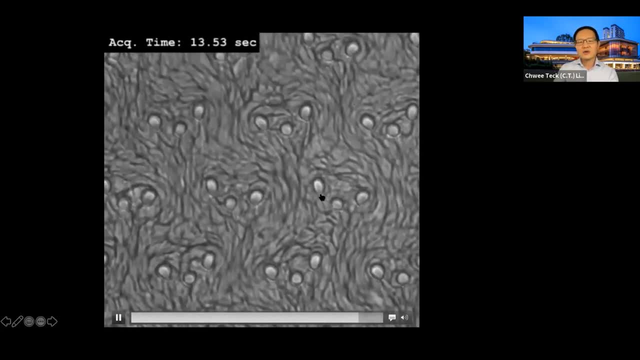 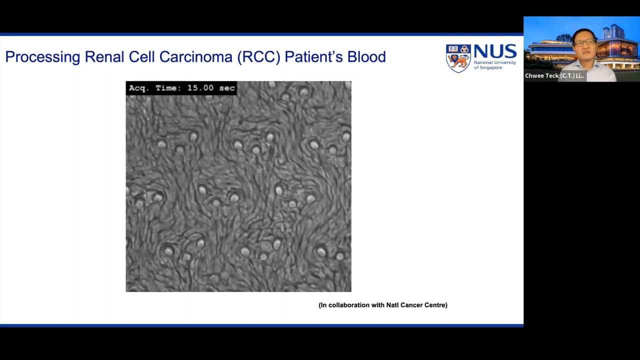 using these three micro pillars When we were doing this, actually, this device took us about, I think, about 7.5 ml of blood. It took us about three hours to process it, So we find three hours is quite long. 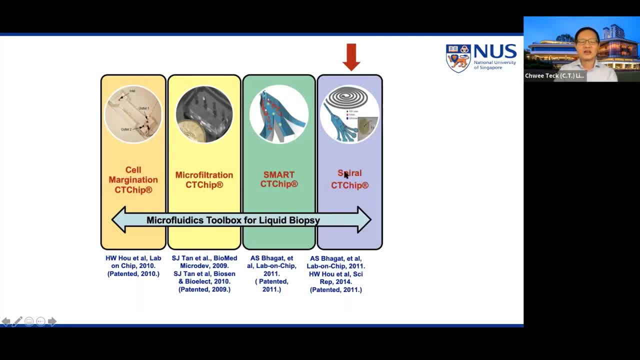 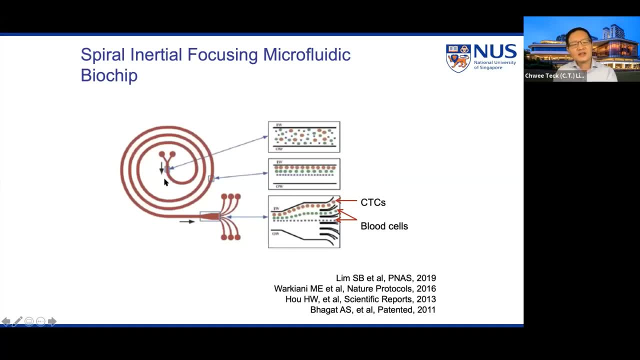 So we started to do, We started to look at another version, another different microfluidic design to isolate cancer cells. So the last device that we come up with it's actually a spiral channel. What happens is we input blood over here. 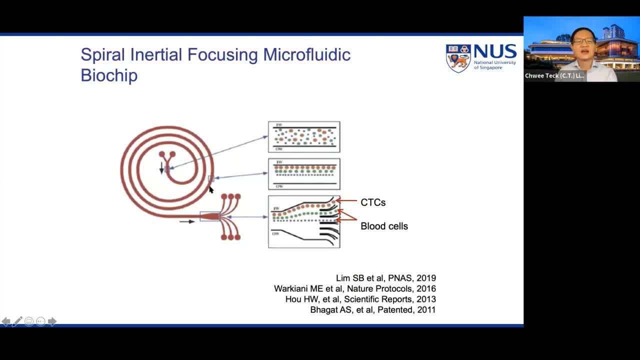 And as the blood flows through a curved channel like this and as it comes up, what happens is the larger cancer cell will get focused near the wall of the channel. The smaller red blood cells and white blood cells will get focused away from the channel. 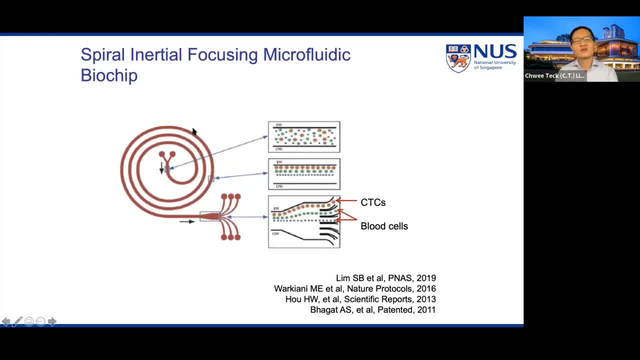 So through just flowing through a curved channel, we are able to separate the larger cells from the smaller cells. Of course, for this device, then, we can only work with cancer cells that are much larger than blood cells and white cells. So how does it work? 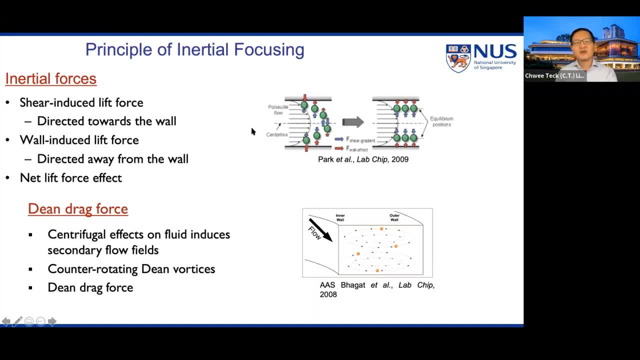 Actually, it is based on the principle of inertia focusing where, if the cell is going through a straight channel like this, it will undergo two types of forces. One is called a shear-induced lift force. It will push the cell near the wall of the channel. 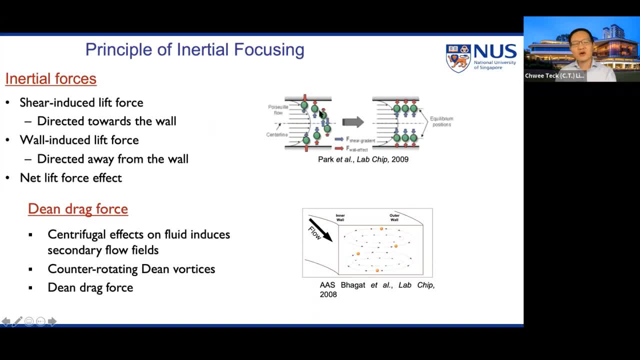 The second is the wall-induced lift force that will push it, push the cell away from the wall of the channel. So what happens is in a straight channel, as the cells experience Poisson flow, it will actually reach an equilibrium position where the cell is somewhat a bit away. 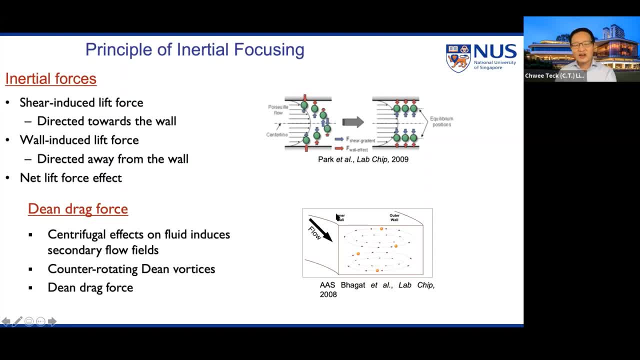 some distance away from the wall of the channel. But if the channel is a curved channel, then what happens is there will be a centrifugal force which will push the fluid from the inner wall to the outer wall. So it's like, you know, spinning, you know. 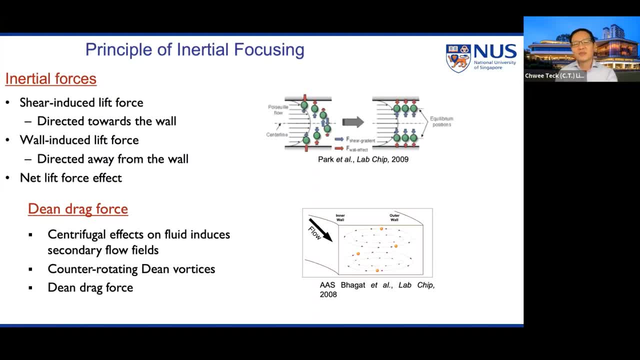 a washing machine, the clothes get pulled outwards. So when that happens, it will create what we call a counter-rotating beam vortices, And this counter-rotating beam vortices will create a beam drag force. So if you look at this equation here, 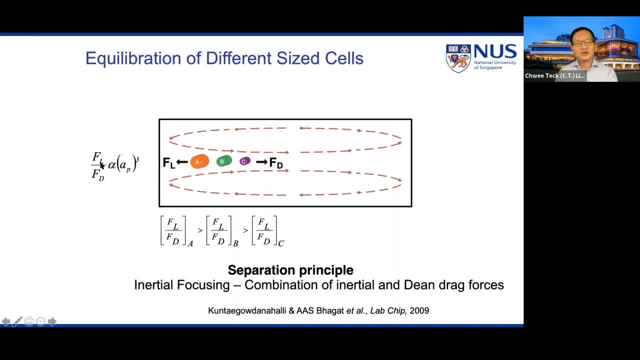 so the equilibration of the different size cells will depend on the lift force over the drag force, And it varies with the diameter of the cell to the power of three, which means that if the cell size is larger, the lift force is higher. 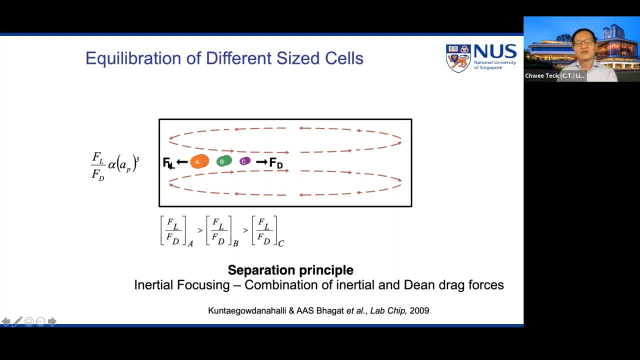 but it will pull the larger cells nearer the wall of the channel. If the cell size is smaller, then the lift force is actually lower. So the drag force will then pull the cell away from the wall of the channel So as it comes up, we can then be able to equilibrate. 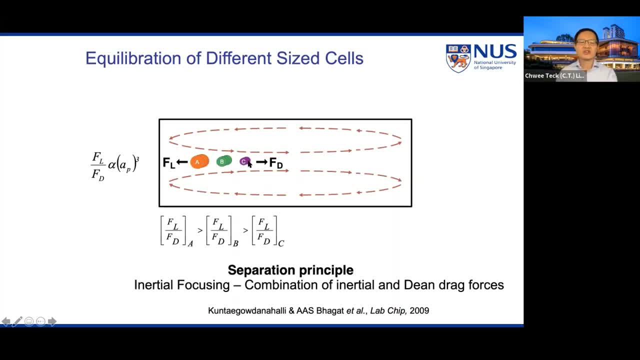 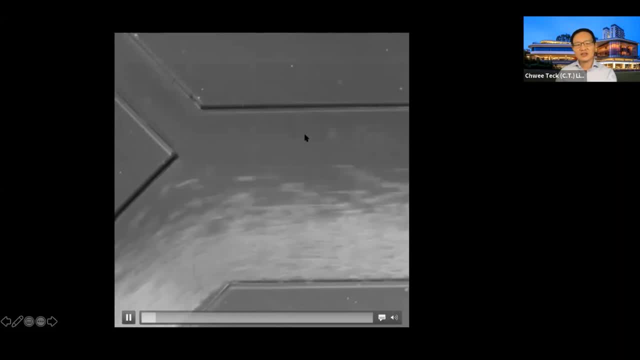 the cells of different sizes at different locations. So, using this principle, we came up with this microfluidic channel to separate the cells: the larger cells from the smaller white cells: A smaller white cells and the smaller white blood cells. So, through this very simple device, 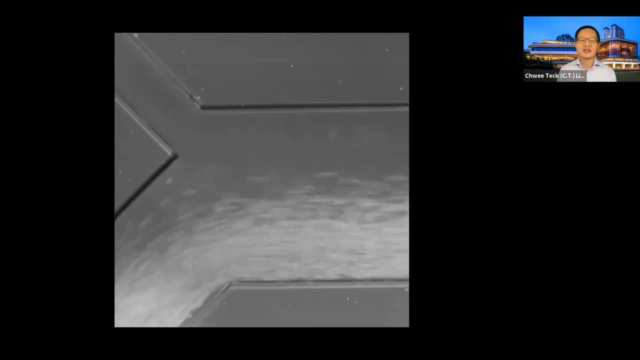 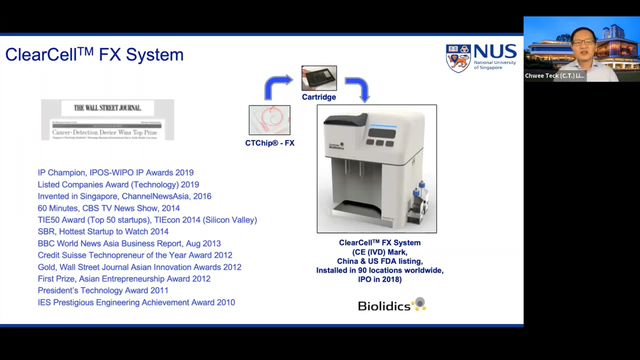 by pulling through a spiral channel, we are able to separate the cancer cells from the blood cells itself. So when we developed this, there were a lot of interest in this, so we thought that we would set up a spin-off company to commercialize this. 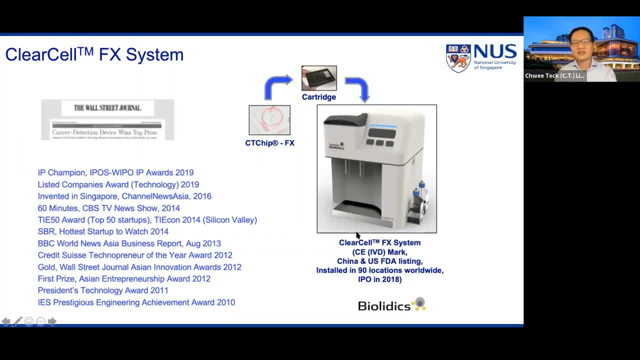 So we have a company now called Biolytics, and this is the system that we have developed, where we have a spiral chip that's enclosed in a cartridge, it's mounted on the top, And then what we do is we can collect 7.5 ml of blood from a patient. 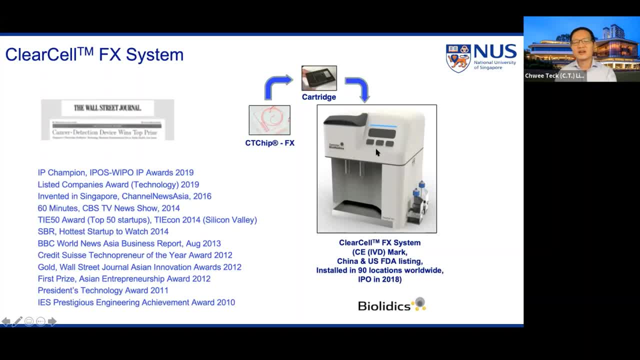 pluck it over here, press a button and then after about within 30 minutes to 45 minutes, we can collect the cancer cells from the other tube. So it's called a clear cell effect system. We have actually obtained our CIVD mark. 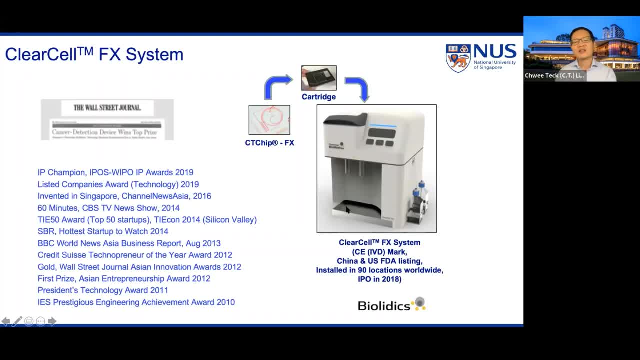 as well as China and US FDA listing as well. So currently it's installed in 90 over locations around the world. So right now we are actually some of the labs are actually using this. We have actually conducted more than 3,000. 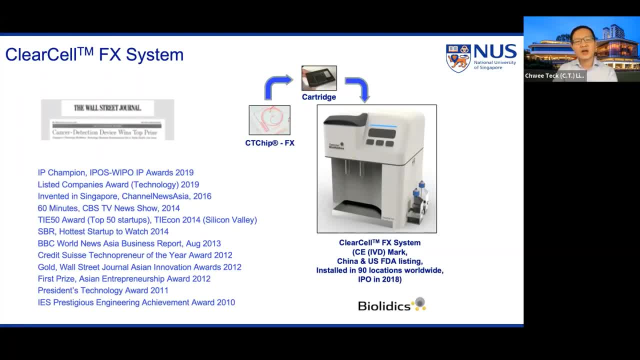 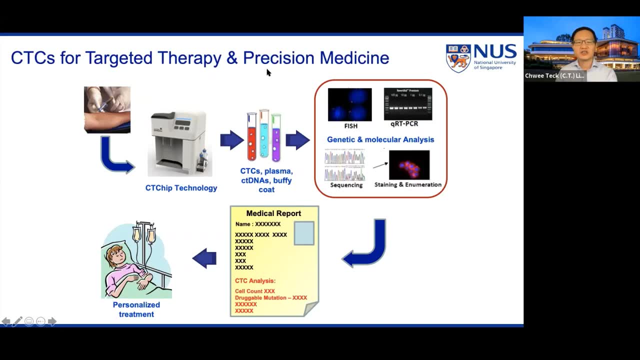 over clinical samples for three types of cancer: breast, lung and also colorectal. So ideal for this system is eventually, for targeted therapy of precision medicine. What we do is we can collect blood from patient, use our system to isolate the cancer cells. 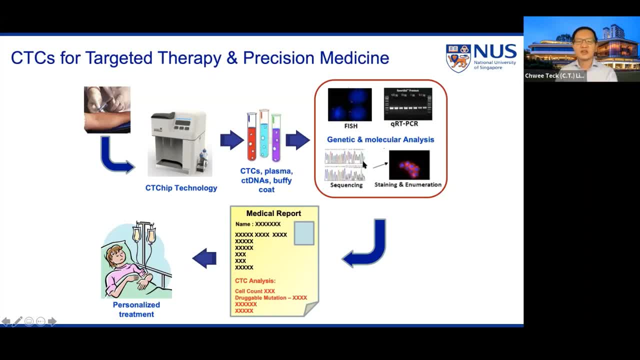 and then thereafter we can do genetic and molecular analysis And with this information we can put in the report. One of the critical information we need is actually what we call a druggable mutation, If a certain mutation that we spotted is treatable by drug. 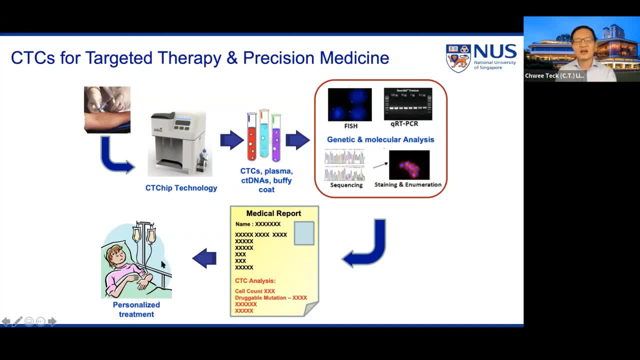 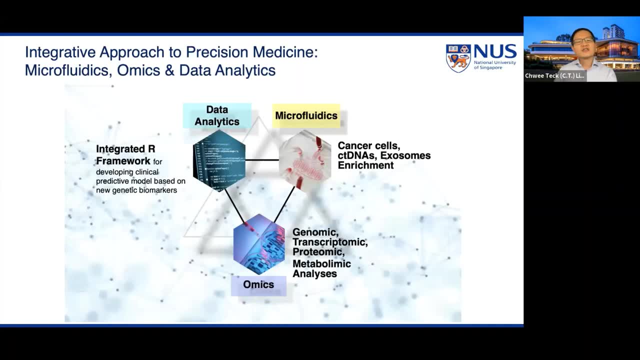 then we can administer the right drug to the right patient. So this enables what we call personalized treatment of precision therapy Moving forward. actually, right now we are looking at having an integrative approach to precision medicine So we not only develop microfluidics. 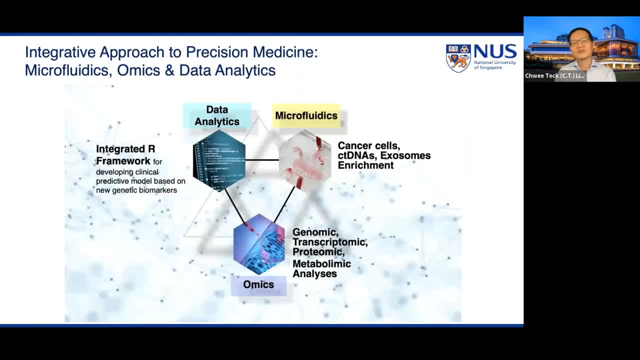 and using this mechanobiological principles to separate cancer cells as well as exosomes. but we are also now profiling quite a number of omics like genomic transcriptomics, proteomics and metabolomics as well. analysis And the last two, three years. 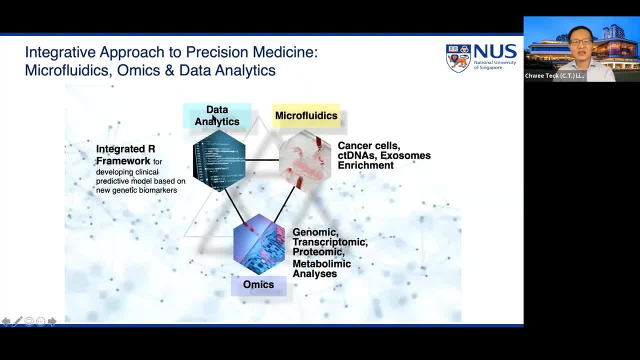 actually, we've been doing quite a fair amount of work in terms of data and analytics. With this huge information we gathered, we are trying to see if we can use data analytics for us to come up with a better panel of biomarkers for us to better diagnose, as well as prognose, cancer as well. 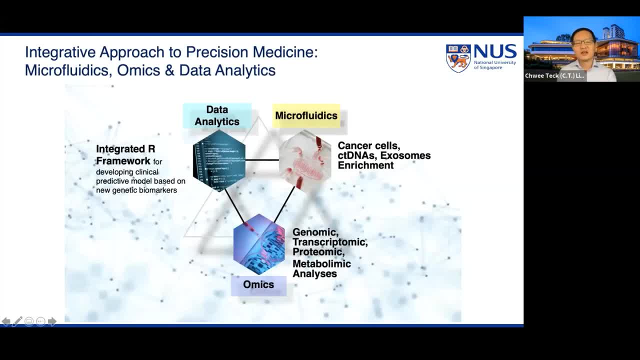 So we have actually a number of papers published in this area. I don't have time to go through them, but mainly we came up with what we call a 29 ECM gene-related panel for us to better prognose and diagnose lung cancer, And this relates to the 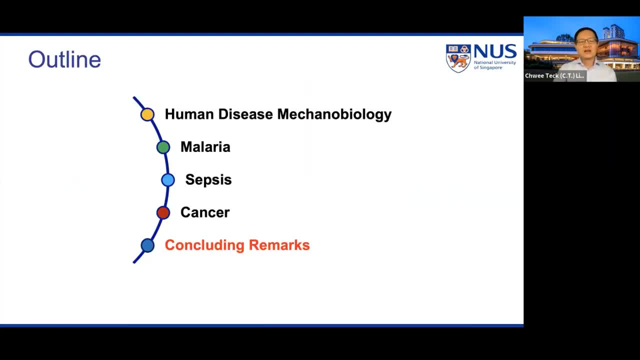 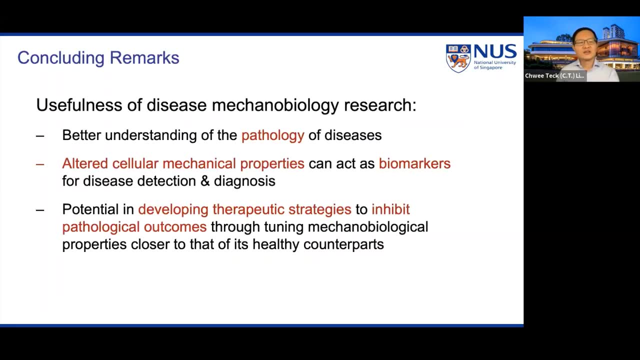 actually the extracellular matrix genes. So with that I'd like to make some concluding remarks. So I've actually show you some the disease mechanical biology research that we conducted. Those are very basic research, but I think conducting this disease mechanical biology research is quite important because they 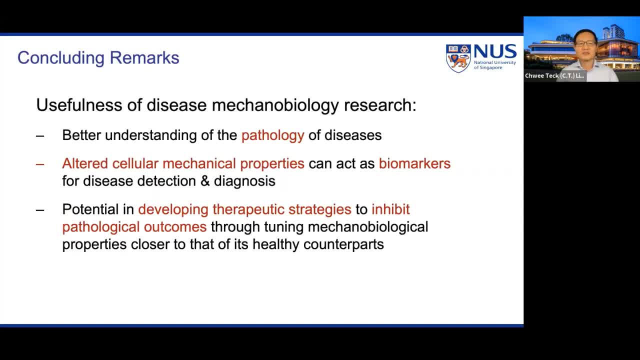 actually can give us a different perspective of diseases and help us to better understand the pathology of diseases. that clinicians and biologists normally would not have done, because their approach is somewhat different from what we are trying to do here. The other thing is, what we observed is that the altered cellular mechanical properties 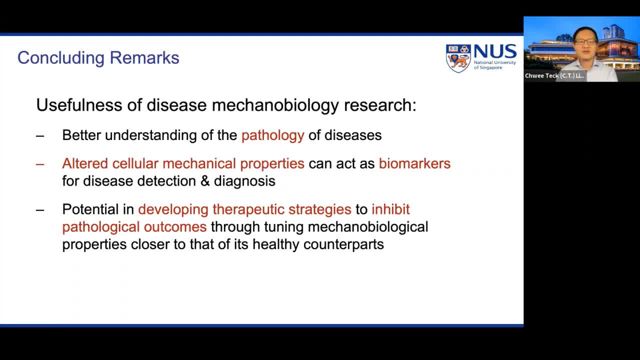 that we have observed can actually act as biomarkers, not only for us to do disease detection but also diagnosis as well. And of course there is also potential use of the knowledge that we developed here in trying to develop therapeutic strategies to inhibit pathological outcomes. For example, perhaps if we can tune, for example, cancer cells to have 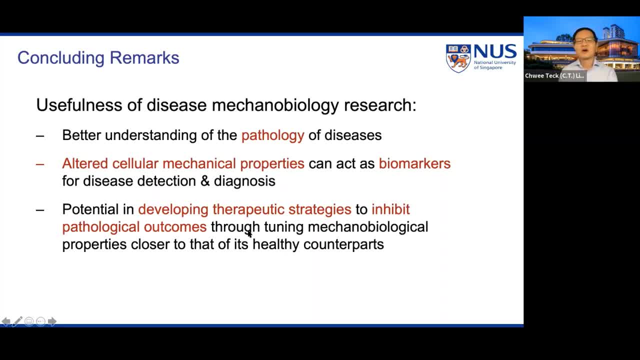 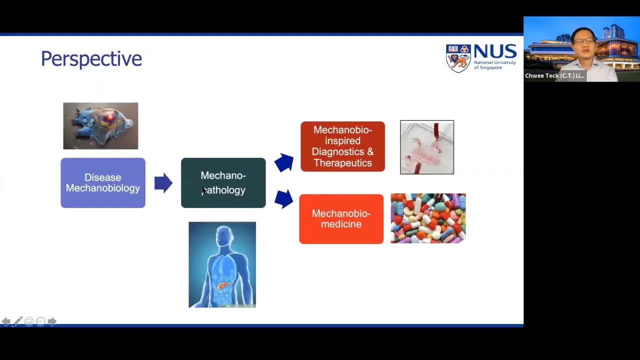 properties that are closer to its healthy counterparts. that might be one way for us to come up with a therapeutic treatment for cancer patients. So there's a potential there and I think it's something that we are very interested to go into. So to bring it into perspective, 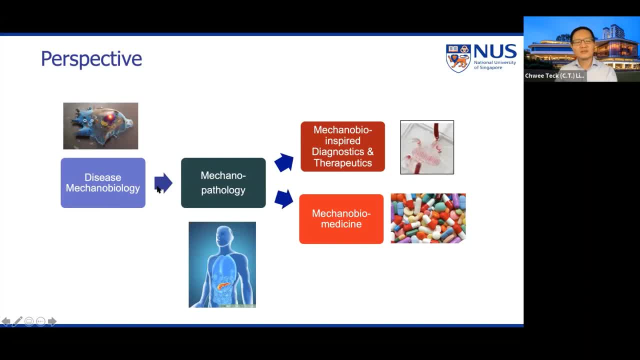 we did disease mechanical biology, and from here we can bring some insights into mechanical pathology. But at the same time, with this knowledge we not only can come up with mechanical, bio-inspired diagnostics and therapeutics, but moving forward also. hopefully, the knowledge we gain can also help us to develop. 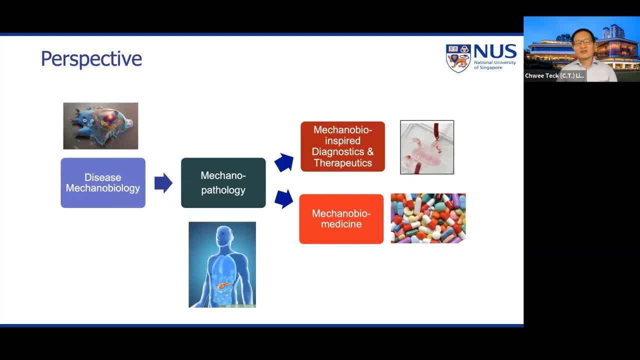 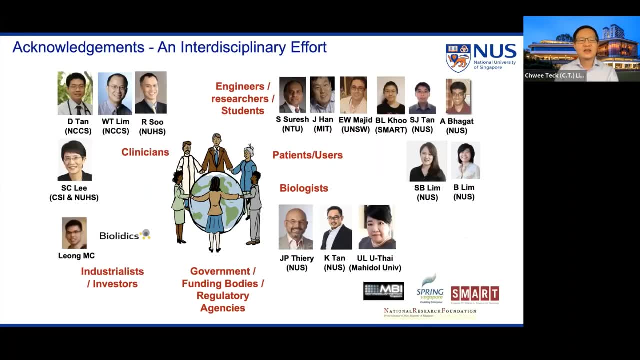 what we call mechanical biomedicine or mechanical bio-treatment of some of these patients suffering from some of these diseases. So, before I end, I just want to acknowledge a number of people: the engineers and researchers and students For malaria, for example. we'll be working. 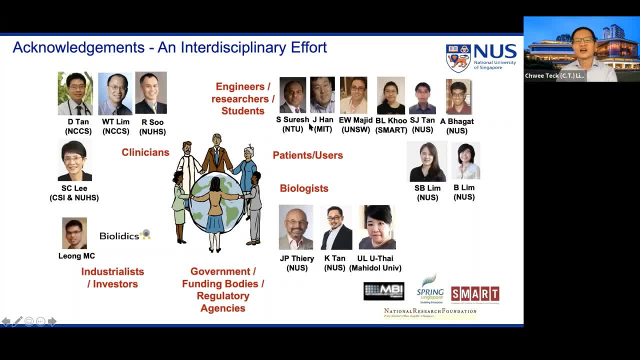 with Professor Subha Suresh, who is now the president of NTU, and also Jae Han from MIT and our postdocs Majid Wilwan, Suijin Ali, as well as Subin and Dina. We also work a lot with 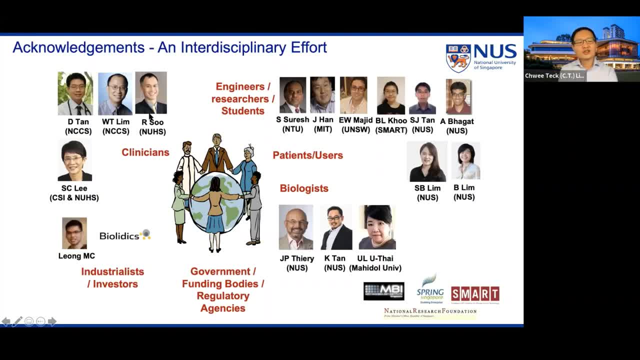 the clinicians from both the National Cancer Center and also National University Hospital and also Cancer Science Institute, And although I'm an engineer, but I feel that it's very important also to understand biology, So we do actually collaborate a lot with the biologists. 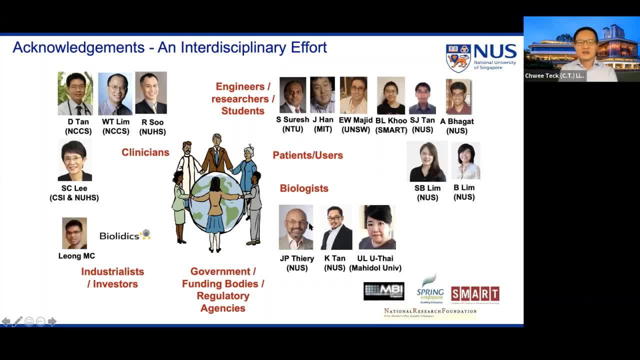 and try to also learn from them. like John Poitier and Kevin, John Poitier is actually working in cancer and Kevin in malaria, and Professor Wu-Sah from Mahido University has been helping us actually with our malaria project, especially in obtaining some of the clinical samples And, of course, 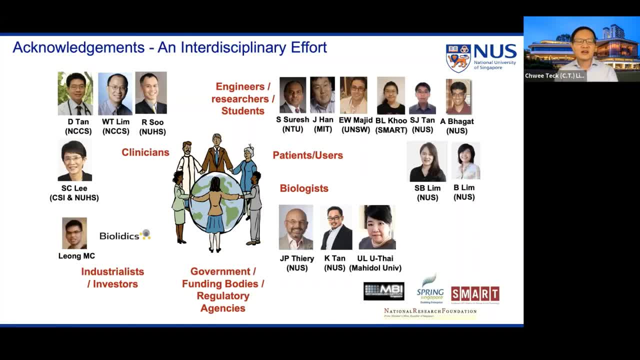 because we are very interested in spinning up some of our devices and technology. so we do work with the industrialists and investors as well. For example, we have Manchun who is working with Biodidx. And of course, I want to also thank the patients. Actually, we don't know who the patients 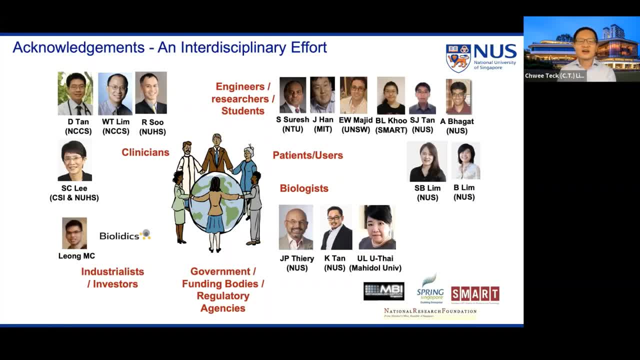 are, but I would like to thank the patients, the biologists, the biologists, the biologists- We really- they are very generous in giving us their blood for us to do the test, And some of them actually are very sick, and so we are very thankful to them. 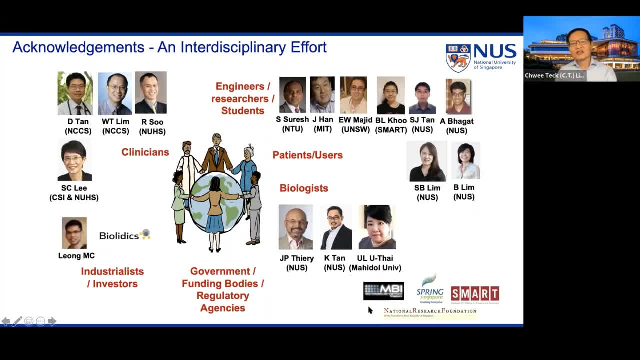 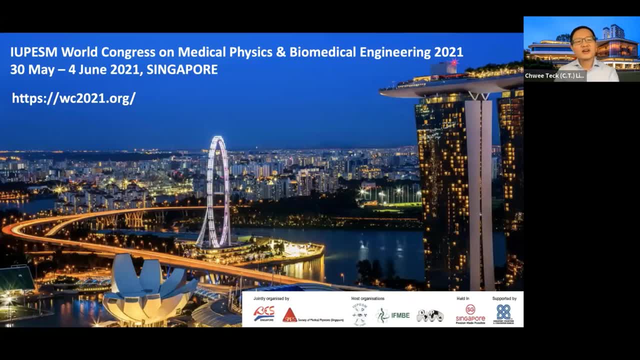 for their contributions. Now, of course, I want to thank the funding agencies as well: MBI, SPRING, SMART and also National Research Foundation. So before I end, I just want to make a quick announcement that we'll be organizing the World Congress. 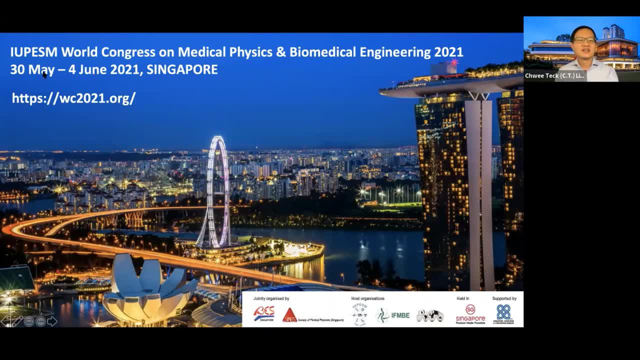 of Medical Physics and Biomedical Engineering next year 30th May to 4th June, So hopefully by then this pandemic will be over, but we'll see what happens. But this World Congress is held once every three years, So it will rotate in North America, Europe and 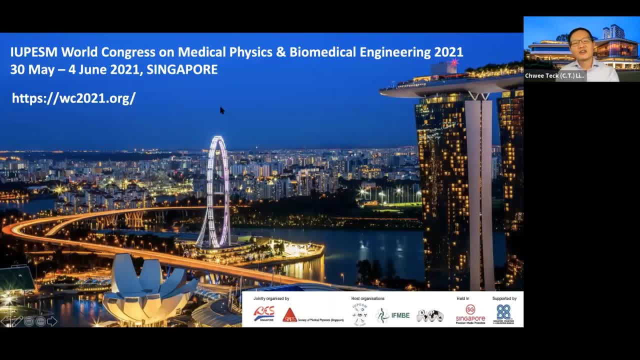 Asia. So next year you'll be in Singapore and I'll actually will be chairing it, So we are expecting about 2500 delegates. So you are welcome to actually join us. If you want to find out more, you can actually visit our website at wc2021.org. 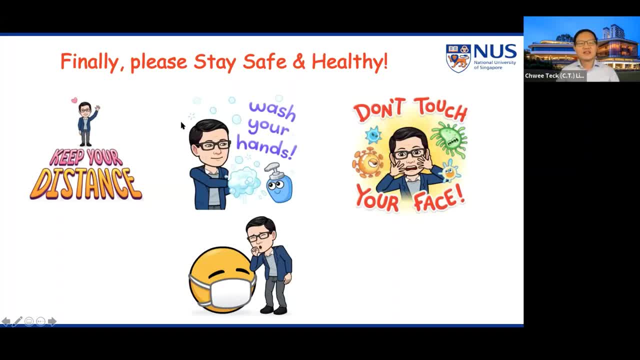 And finally, now, in this pandemic situation, hopefully you'll stay safe and healthy. keep your distance, wash your hands and don't touch your face. Also, wear a mask, which is really what we are doing right now here in Singapore as well. So with that, thank you so much for. 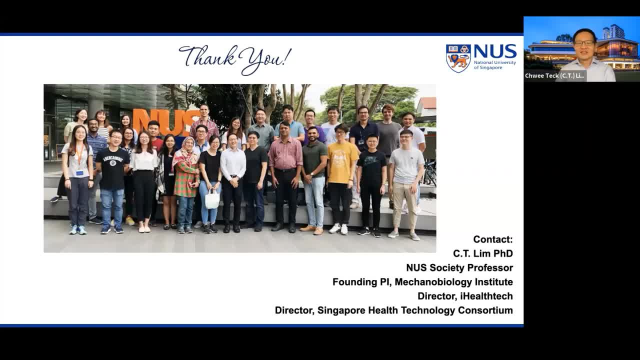 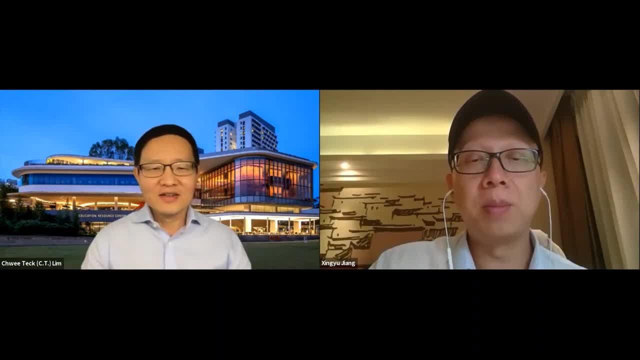 attention and I'll be happy to take questions. Thank you very much, Professor Lin, for a talk with not only insight in fundamental science, but also the importance of the COVID-19, but also real-world application, particularly in the clinics, And it's my understanding that you're also working to fight the. 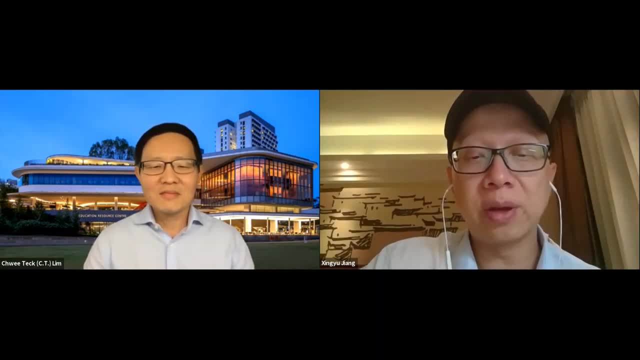 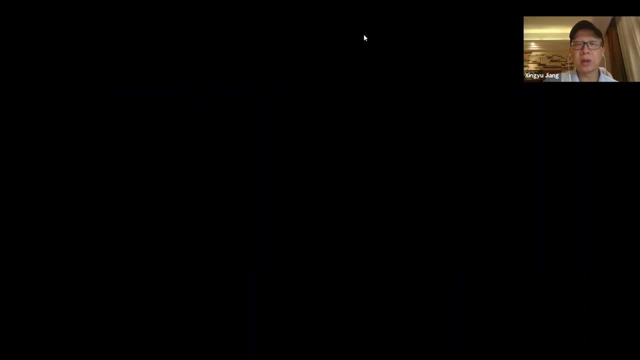 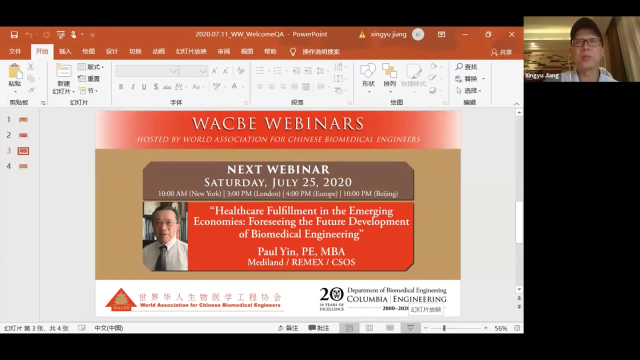 COVID-19.. Maybe next time when you give a talk to us, you'll tell us about that. Before the question and answer period, let me do a short ad of our next presentation, which will take place Saturday, July the 12th. 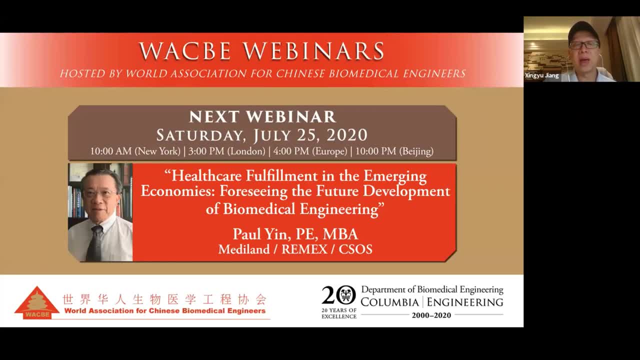 Thank you. Okay, so we are on the 25th at 10pm Beijing time, exactly this time, two weeks from now, And Paul Ying will tell us about healthcare fulfillment in the emerging economies, foreseeing the future development of biomedical engineering. So very applied topic: People. 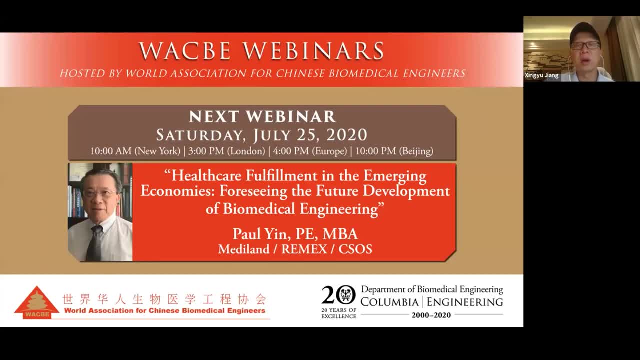 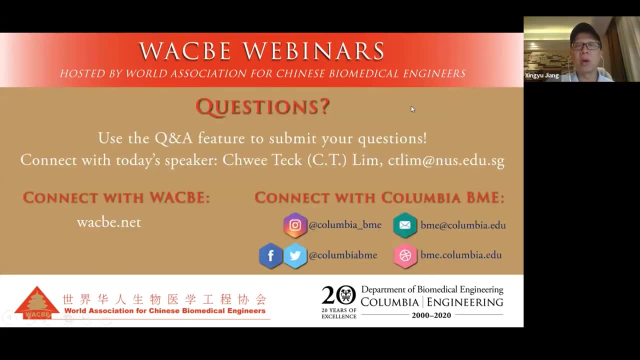 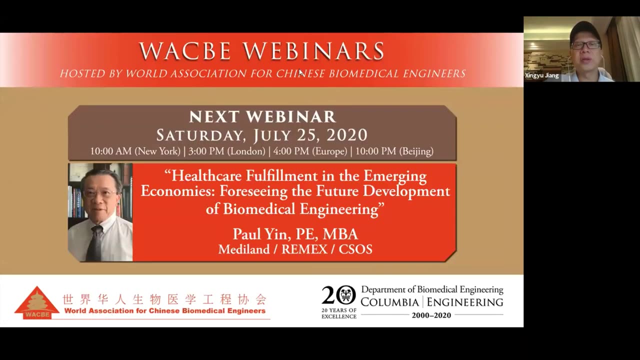 who are interested in this topic should mark it in their calendar and join us in two weeks time. So now the floor is open for questions. I will select questions based on their relevance. I see quite a few people have raised questions, but some of them are not entirely relevant And, in the meantime, if your 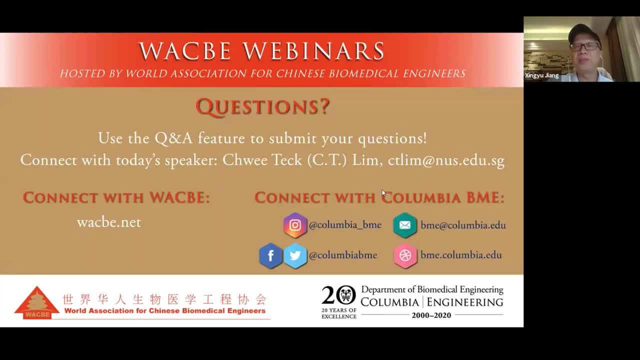 questions didn't get answered. you can email Professor Lin in the email outlined in here, And I will also like to thank Columbia BME for hosting the talk. So the first question is: is the process of filtering red blood cells in the multiplex channels traumatic? 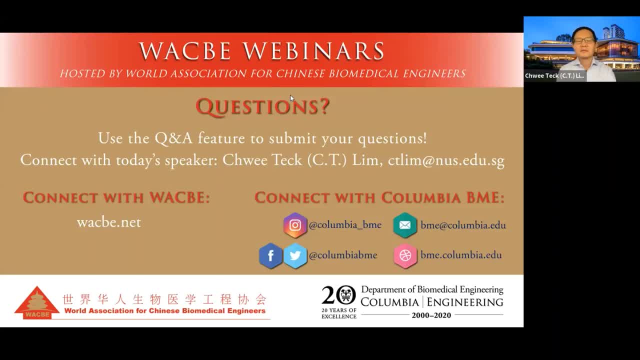 Right, yeah, So this is a very interesting and good question. Yeah, so when we filter the blood, we do take note of the forces that's acting on the red blood cells. So so we, when we first, when we designed the device, for example, we carefully, you know, kind of calculate what the shear forces and pressure. 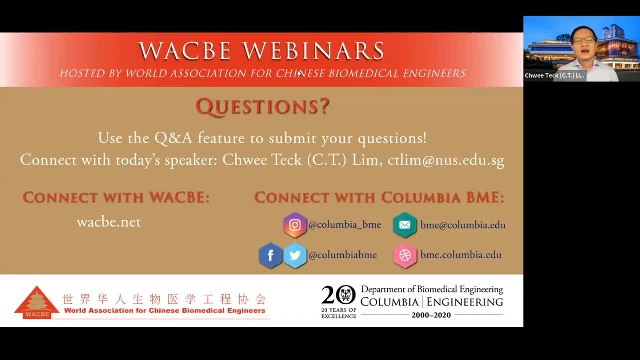 will be acting on the blood cells. Of course, when you do the experiments, after we collect the RBCs, we also look at whether RBC has been lysed and so on. So the filtering actually, I would say, is not not traumatic in the sense that we want to preserve the red blood cell after flowing. 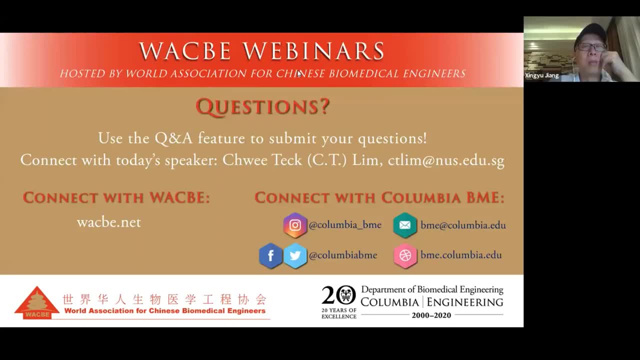 through the device. So it could be, for example, either slowing the flow or designing the structure such that it will not be, you know, create any, any effect that would damage the red blood cell. So I would say that this is part of the 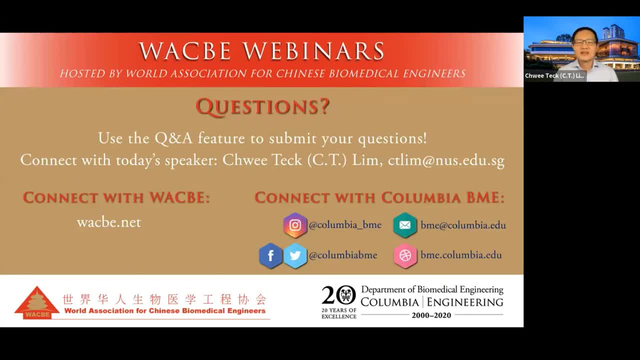 design consideration. Thank you. Next question: since cellular biomechanics may be influenced by extracellular mechanical signals, how can we relate properties in vitro to properties in vivo? Thank you, Right, Yeah, So that's okay. Another interesting but not easy to answer question. 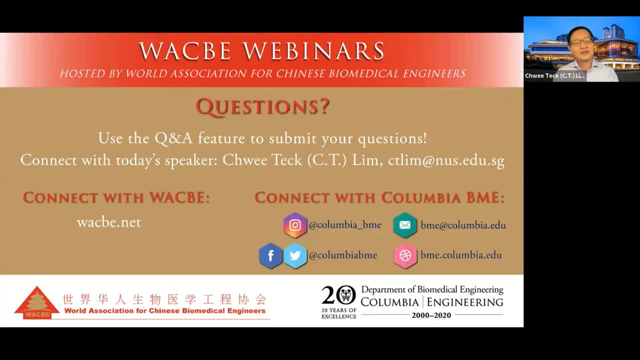 Yeah, I mean a lot of experiments we do, yes, definitely in vitro, And you know, if you talk about in vivo, right, it's hard to actually be able to estimate, for example, the kind of the, for example, if you're talking about in the, in the tumor itself. 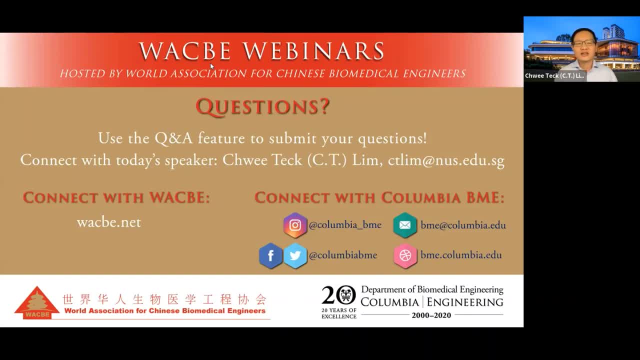 Actually, one of the research we have is looking at cell adhering to a tumor, looking at the tumor stiffness and whether the difference in the tumor stiffness will either encourage or discourage cell proliferation or tumor growth. And most of the time it's not that easy to know exactly how much of the forces of pressure is actually acting within in vivo itself. 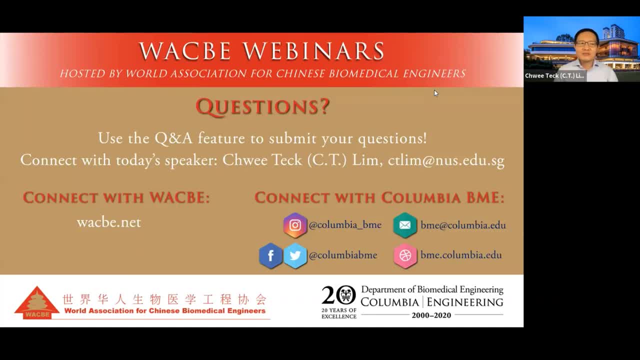 I think the only closest we can do is maybe in mice where we can insert some probes to kind of measure what the forces is, but certainly in the human body I don't think we can actually be able to actually do that. We can estimate but we will not be able to do that. 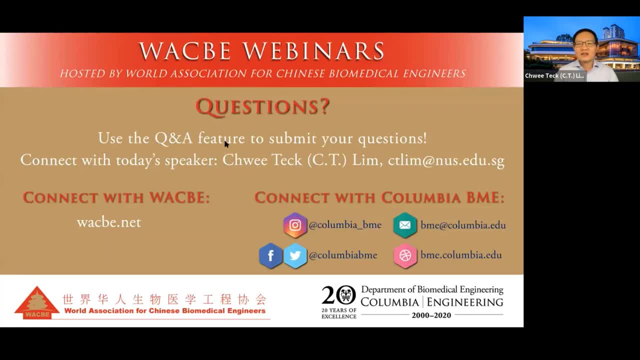 But we will also try to see, for example, in mice. we can probably probe it and then try to mimic the kind of parameters that we observe, What we think we are observing in vivo, to the in vitro environment. Yeah, so it's not that easy if you want to say, you know, have an in vitro that will be able to perfectly mimic that in vivo properties. 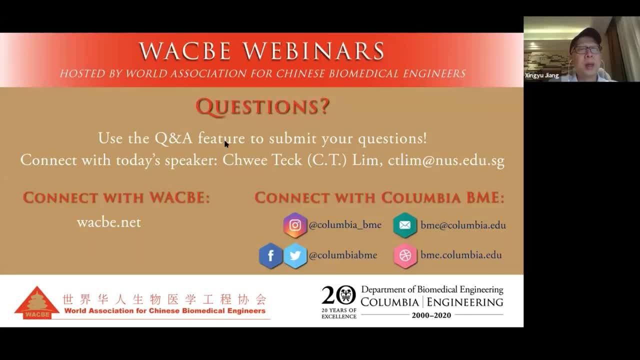 Thank you. Next question: Can you please give some explanation on the reason why malaria infection increases cell stiffness? Is there any? And do you get a molecular understanding of how the infection increases the stiffness? Right, yeah, So there are two parts to it. when malaria infects into the red blood cells, it will actually causes changes. 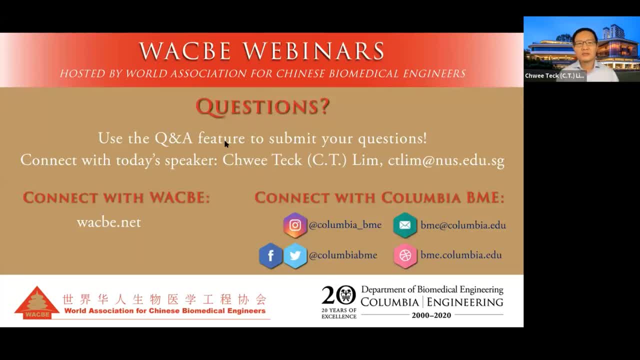 So it will actually. Firstly, it will multiply, it will consume the hemoglobin, It will actually produce many byproducts within the red blood cell, And so some of this additional products in the red blood cell will cause the whole red blood cell to be stiffer. 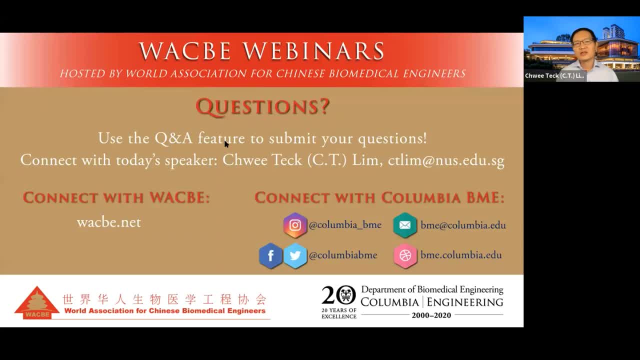 And then secondly, is that it will actually export protein to the membrane and some of this protein will interact with the spectrum network, which will cause the spectrum network to be also stiffer. And so when we do micropalpate aspiration to measure the shear modulus of the membrane, 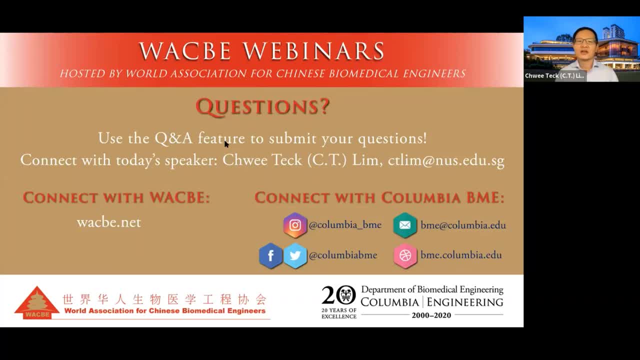 we'll see also, there's an increase in stiffening of the membrane. So there are two parts to it. One is within the cell, because of this byproduct that's produced when the parasite consumes the immunoglobulin that causes the whole cell to be stiff, and then second is the membrane. 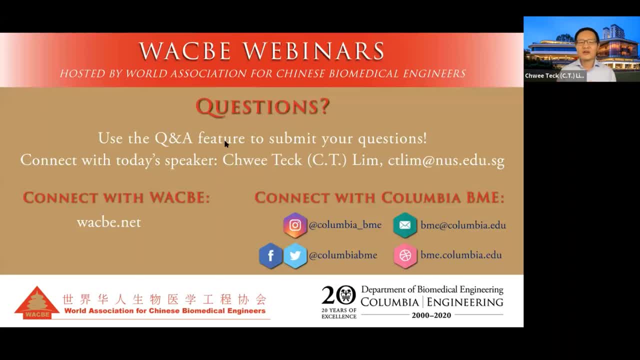 itself. So that's what causes the whole malaria-infected cell to be stiff and also sticky. Thank you. As time is drawing very close to the end, I would like to maybe ask the final question. So you mentioned the ClearCell, the commercialized product, can work with breast cancer. 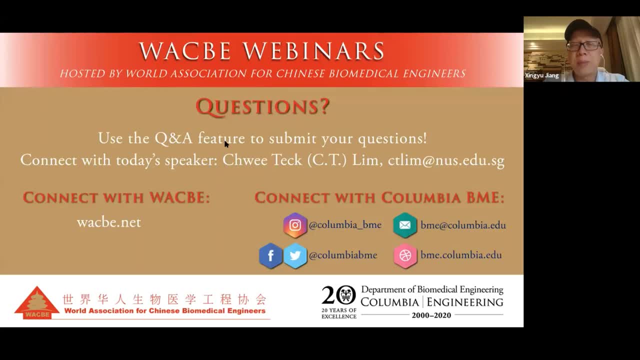 Can you talk about breast, lung and colorectal cancer? I didn't hear hepatic cancer, which affects the Asian population in particular. Is that in progress or is that something that's already done but you didn't mention? Yeah, So hepatitis, we have actually also tried. we were able to actually, at least for the 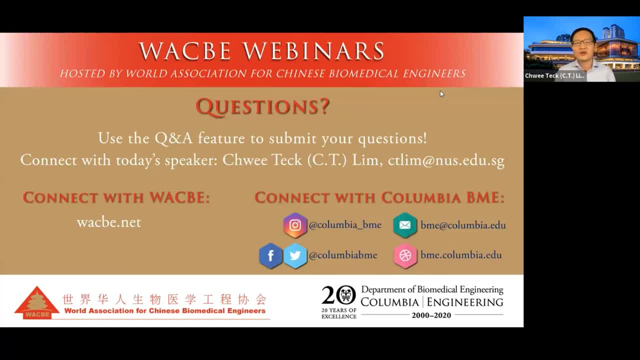 small number of tests that we've done, we found that we were also able to detect them. The reason why we're going for, like, breast and lung is also because you know. if you're going for lung it's also because those are because when you go for FDA approval, normally 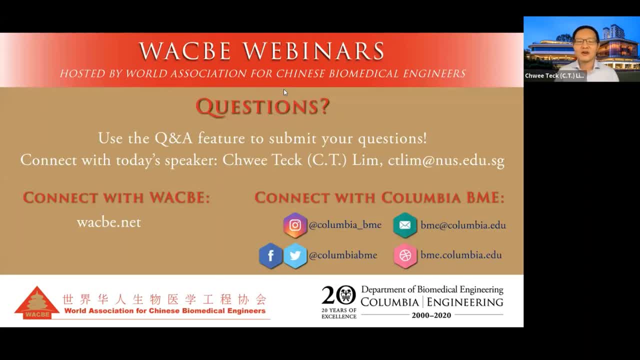 you have to state you know what type of cancer you're going for. you cannot say all cancer types, And so we are kind of zooming in on the more serious cancers, the more prevalent ones. So lung, breast, colorectal, actually also prostate, for example, are the cancers that? 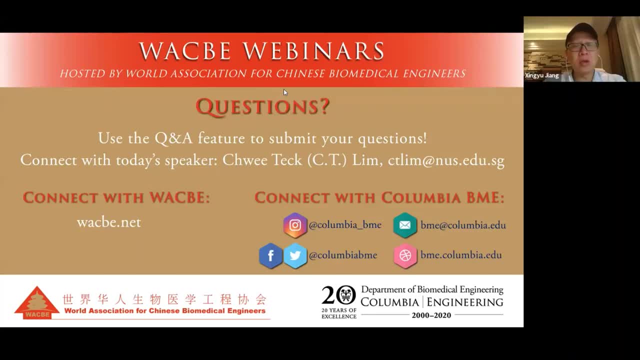 we're looking at. Okay. Well, there's one final question which just came up which I think is important. maybe you can briefly answer this. Okay, So is it possible to remove cancer cells from blood for those patients with late stage? 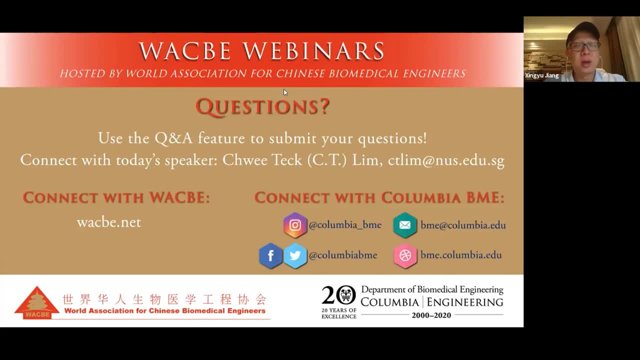 cancer that are too late for surgery, Right Yeah, Blood cancer, Yeah, So that's a good question And in fact I didn't mention. but we did develop a. we kind of multiplexed and stack up a number of microfluidic chips to do cleansing of cancer cells from sorry cancer cells. 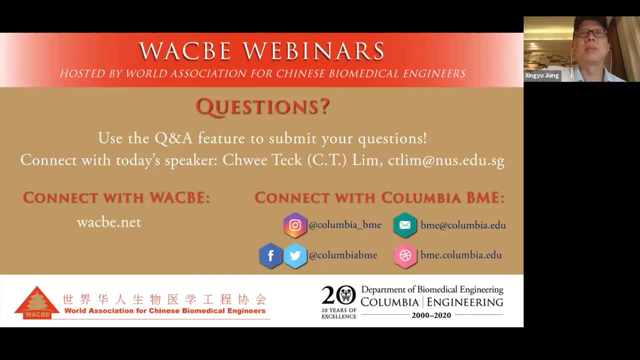 from blood cell right. So it's like a diagnosis? Yes, But the reason why we do this is because we're talking to a clinician. the clinician was doing operation on the spinal tumor of patients And when they do operation, the patient tend to lose a lot of blood, sometimes one to two. 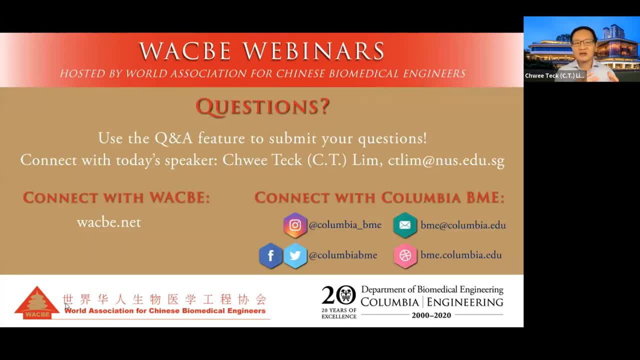 liters or even more. And he was asking: can we salvage this lost blood and then clean it of the cancer cells before they rub the blood back to the patient? So in that context we came up with the system- Okay, So we came up with the system to clean blood of the cancer cells before we rub the blood. back to the patient instead of using donor's blood. But if you're talking about trying to remove cancer cells from blood for very late stage patients who cannot go for cancer for surgery, then we are not treating the cancer at the source, because the tumor will still be there. the tumor will still be shedding cancer cells. And even if you can remove cancer cells from blood, you know the tumor will still be there. So so you know, normally we don't treat patients. We don't treat patients that way. Yeah, I think there's a subsequent question about blood cancers. 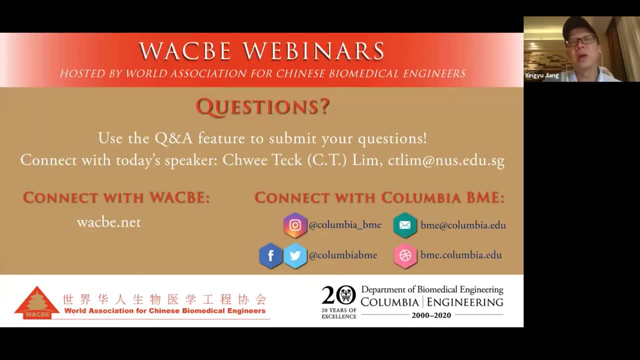 Would it be possible viable strategy for removing the cancer cells for blood cancers, Right, Right, Yeah, So it's a good question, As I mentioned, because we are trying to remove cells, cancer cells- because they are stiffer, sorry, they are basically larger or stiffer than blood cells, right?